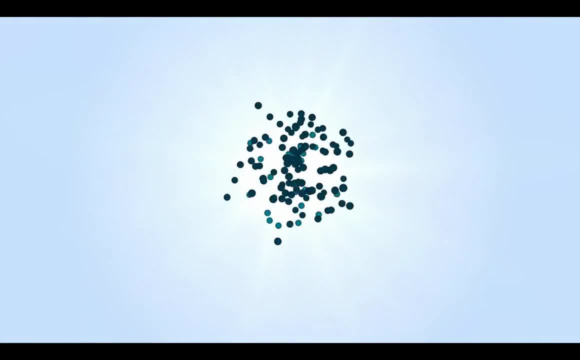 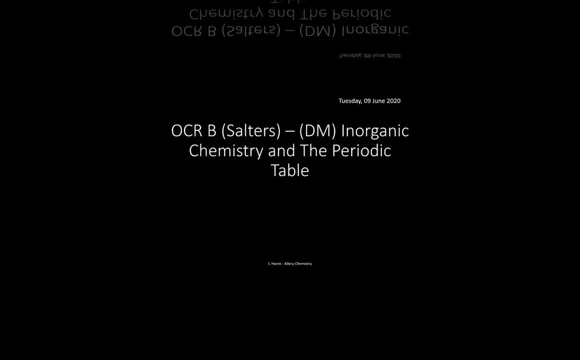 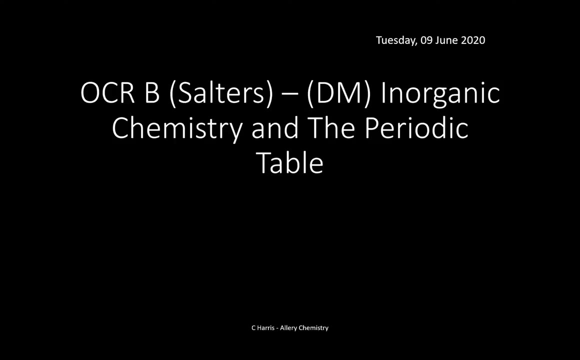 Hello, my name is Chris Harris and I'm from Aloe Chemistry, and welcome to this video on inorganic chemistry and the periodic table. This is for the development metals topic and there's two videos in this topic that cover the DM topic and it's for OCRB salters, So this video actually goes. 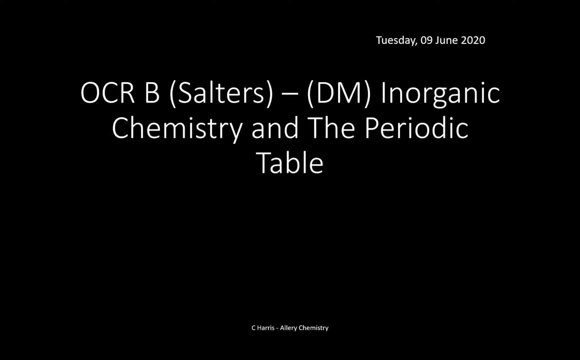 through the specific content for salters. So if you are studying salters at A-level chemistry or A-level chemistry salters, then this video is perfect for you. It's not generic, it's actually tailored towards the specification and in fact, there's a full range of salters videos There's. 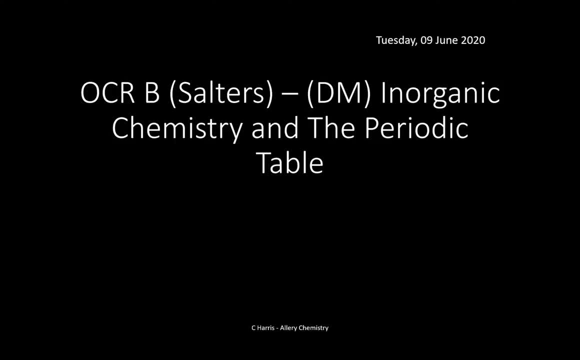 year one and year two videos, all on Aloe Chemistry YouTube channel. I've also got some generic white board tutorials as well, where we go through some specific topics which are quite generic, and there's a full range of of stuff on there. It's all for free. All I ask is you hit the subscribe button and that'll be. 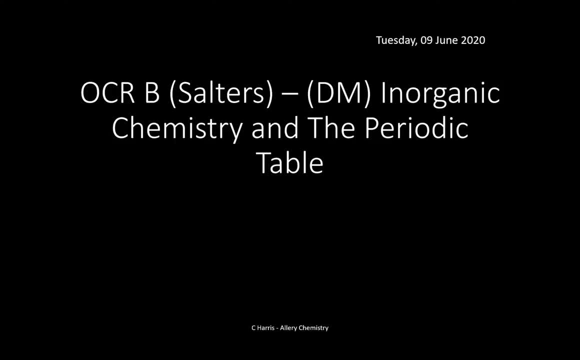 absolutely fantastic. Also, this video here is actually created from revision slides that I've made and they're available to purchase, So if you'd like your own copy of these, and click on the link in the description box below. they're great value for money. You can use them on the. 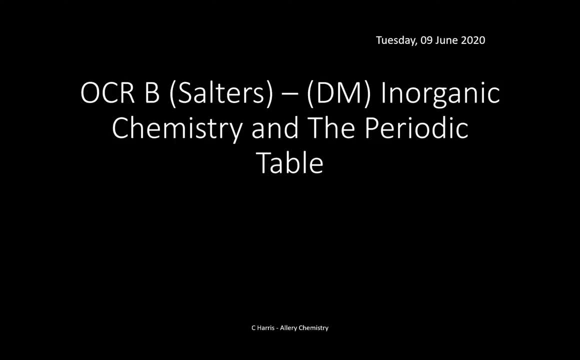 move on your smartphone or on your tablet. I've known people to print these out as well and use them as revision notes. you know for their for their own use and put it in their files So you can use them for anything you're interested in. I've also got a full range for year one and year two. 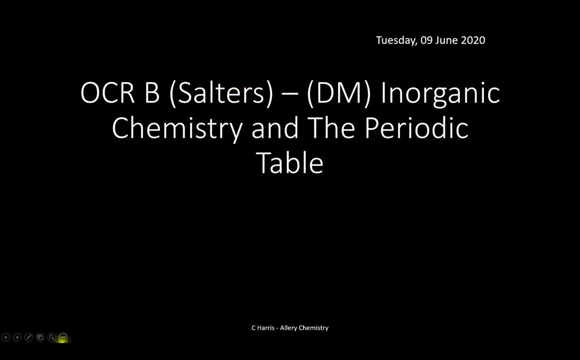 salters all available in that link, So just go and have a look on there. Okay, so, like I say, this is dedicated to salters for the developing metals topic. there's two videos in this series that covers DM, so I've decided to split it up because otherwise it'll be a very, very long video, if it. 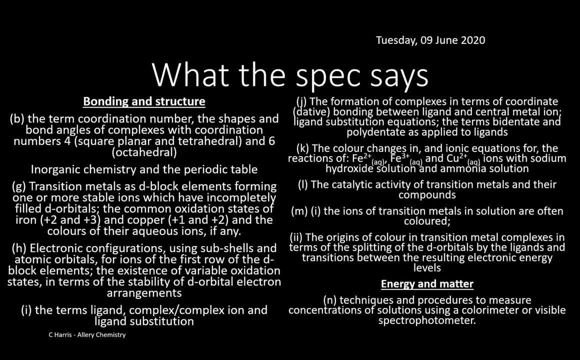 was all in one go. So this is. this video is going to cover areas such as transition metals. we're going to look at that. We're going to look at what ligands are. We're going to look at the orbital splitting- I've got some colors as well. so reactions of that, including ligand substitution, and then finally, 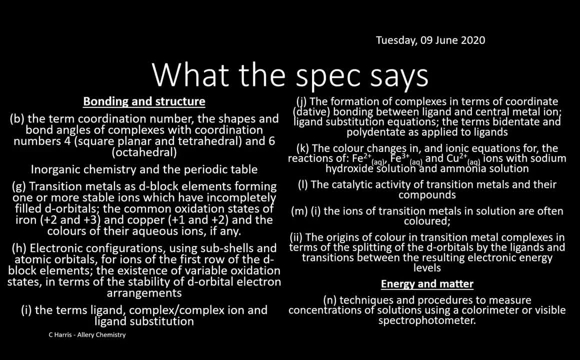 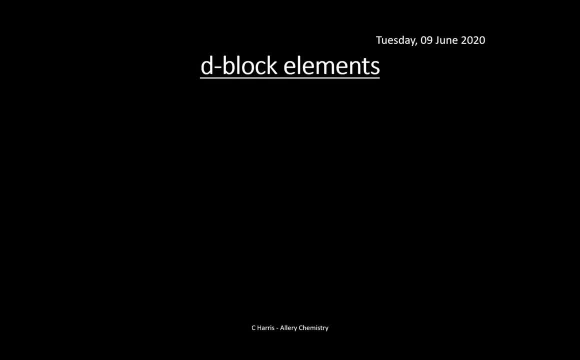 we're going to look at some colored complexes and how we can analyze them and determine the metals. that's in solution. so that's the running order for this video. so we're going to start by looking at d block elements first, so you need to know where the d block elements are in the 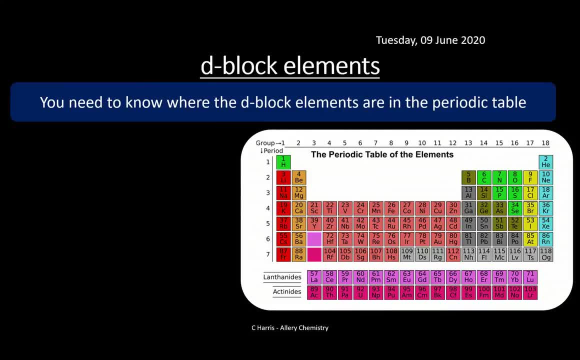 periodic table. so you can see there that we've got the periodic table and put in front of us. and the d block elements is this middle bit here that's highlighted in red. so it's this bit here. okay, so these are d block elements. so some of these elements are transition elements, not all. 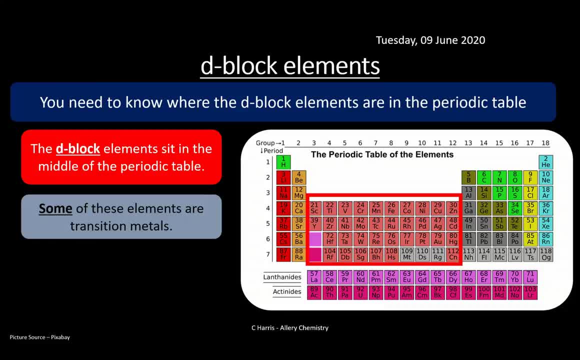 of them, though you must distinguish the difference between a d block element and a transition element, and we'll look at that a little bit later. so the ones that you mainly need to know, the ones in the top row of the d block there. so that's scandium, which is sc through to, you've got titanium. 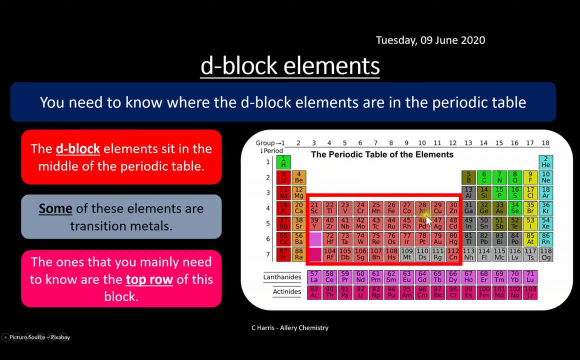 vanadium, chrome, manganese, iron, cobalt, nickel, copper and zinc. so you just need to know mainly these ones here, and the video is really going to focus on that. but you may be asked some of these, but it's merely you need to be quite knowledgeable on these, these ones here, and you'll be doing just fine if you can. 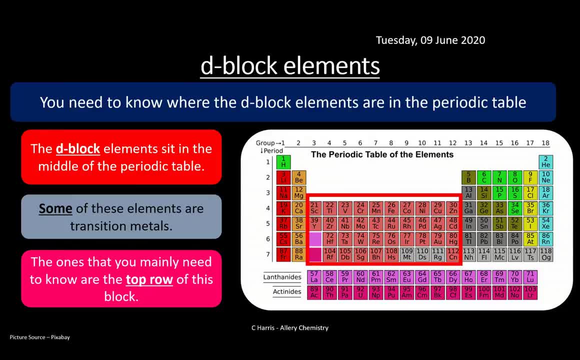 do that okay. so we're going to look at the electron configuration so we know where these d block elements are. so we need to know why they're called d block elements first and what the difference is between that and transition elements. so the electric configuration is actually quite important. 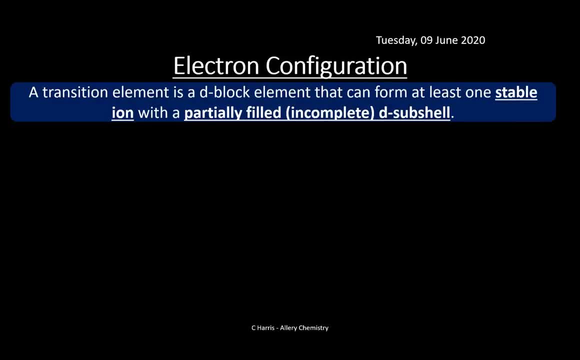 and you would see this in year one chemistry. so this is just using some of the knowledge from year one chemistry and adapting it to transition metals. so a transition element is a d block element and a transition element is something that forms at least one stable iron with a partially filled or 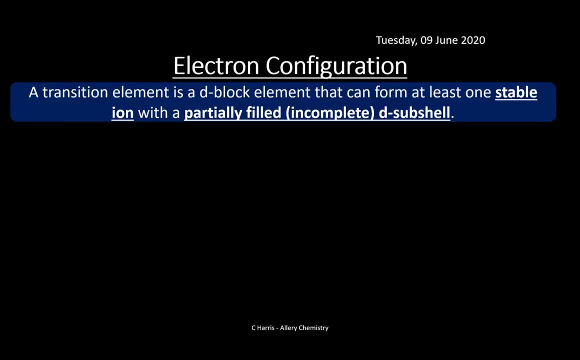 incomplete d subshell. okay, so that's a transition element. that's very important. okay, so it must have an ion. okay, that has a stable. it's a stable iron. there's a partially filled d subshell, not an atom, as you'll see later. so a d subshell can hold up to 10 electrons maximum, okay, and for period. 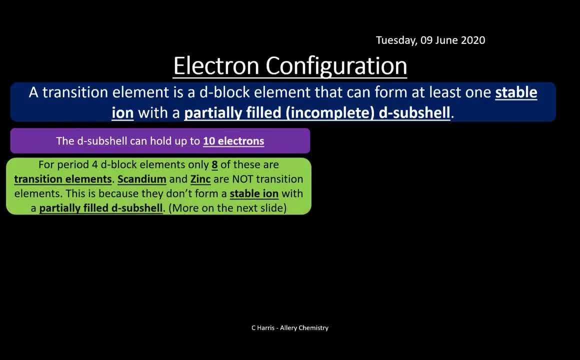 and for period four d block elements. only eight of these are transition elements. so scandium and zinc- these are the ones which sit either side of that top raw, so scandium is on the left and zinc's on the right. these are not actually transition elements. this is because um when they their 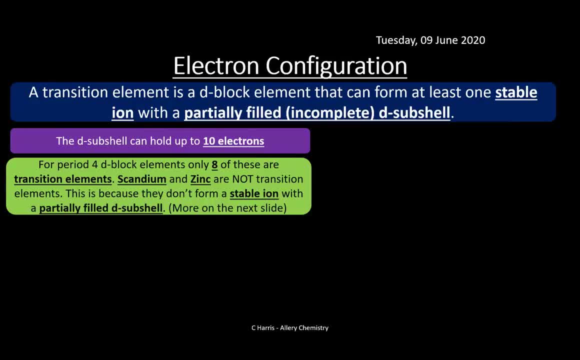 stable iron that they form. um doesn't have a partially filled d subshell, so therefore it cannot be a um, a transition element. but look at more of that a little bit later in the in the next slide. okay, so the electric configurations of the eight transition elements in period four. so we're going. 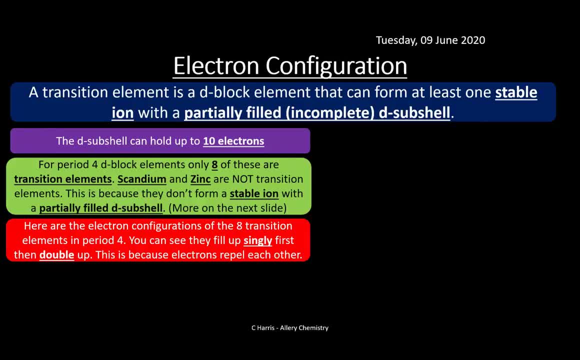 to look at them, and what we're going to see is you'll see they fill up singly first, then they double up, and this is because the electrons actually repel each other. i liken this a little bit to um, say, if you get on a bus, um, and so when you get on a bus, i normally find um, i don't know. 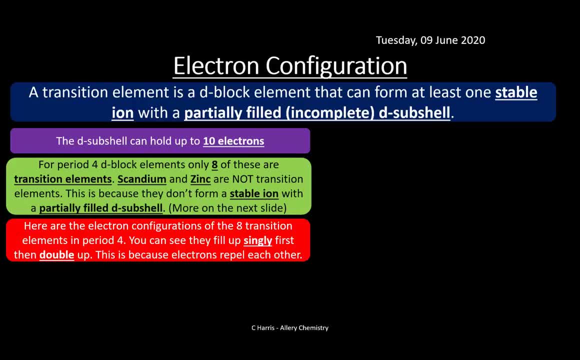 something that i that i normally um that i observe anyway- is that people would normally like the privacy and they'll sit on their own seat. so if somebody's sitting in one of the seats, they won't go and sit next to them. if there's an empty one, they'll go and sit in that empty one first and it. 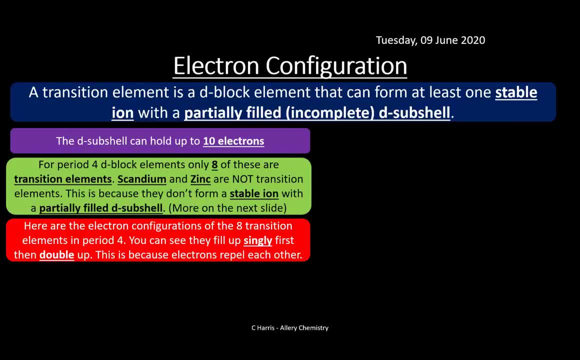 oh, it isn't until all of the seats are actually occupied. then if you want a seat you're going to have to sit next to somebody else on the bus. so electrons are in a similar position in the fact that what they'll do is they'll kind of occupy their own um, their own orbital, first and then. 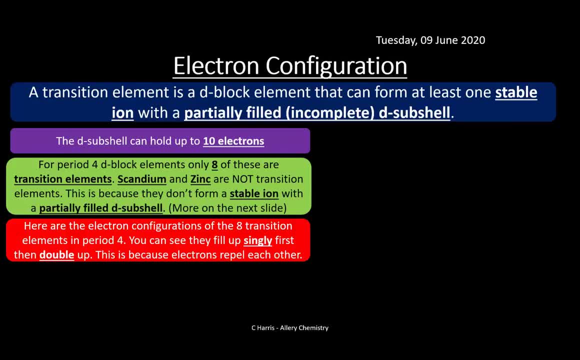 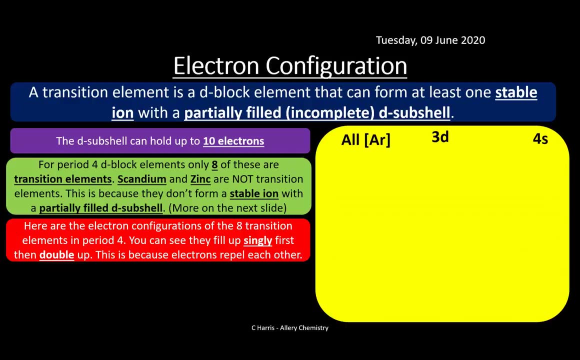 serve doesn't actually make it. it's all essentially a. i've got ar in square brackets and basically what this means is this is the electron configuration of argon. so all of this is the electron configuration of argon. so this is basically these electric configurations I'm going to show you of the transition metals in the top. 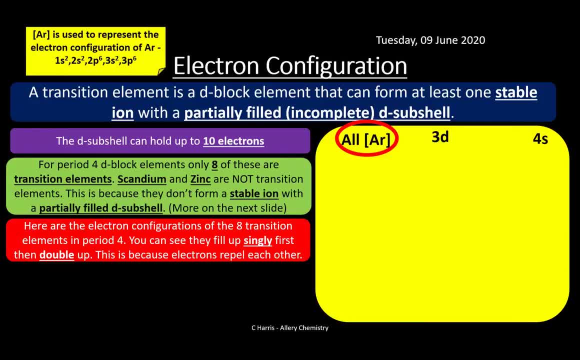 row of the transition metal block or the D block. then, instead of writing out the electric configuration all the time of the first few orbitals, you can see here what we can do is we can just write AR, that's the transition, that's the noble gas configuration, and then 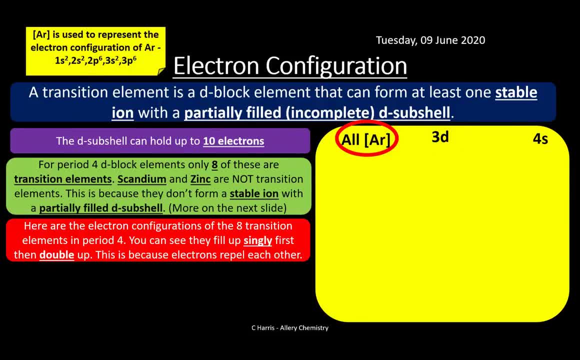 whatever's changing here. So that's the noble gas configuration there, but you'll see what I mean. So titanium has the noble gas configuration. whoops has the noble gas configuration. plus, it has two electrons in the 3D subshell and two in the 4S one. These two are very 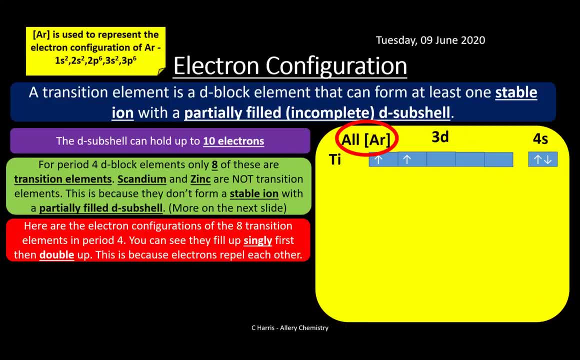 close in energy. that's why these are written here. Vanadium is the next one down that has three electrons in the 3D and four and two in the 4S. Now it gets a little bit strange when it gets to chromium and you'll see there's chromium. 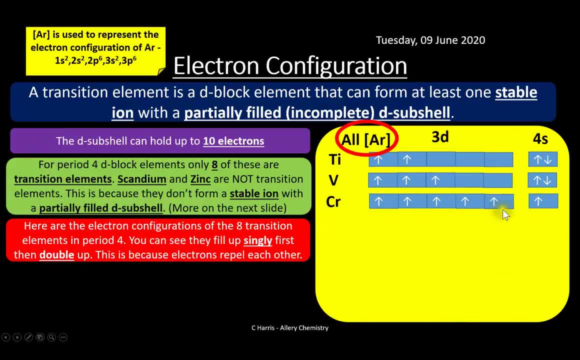 So what actually happens is that in order for this to form a half full 3D subshell- that's quite stable that configuration- One of the electrons in the 4S actually jumps down into the 3D orbital. here, Because these orbitals are very close in energy, the electrons can. 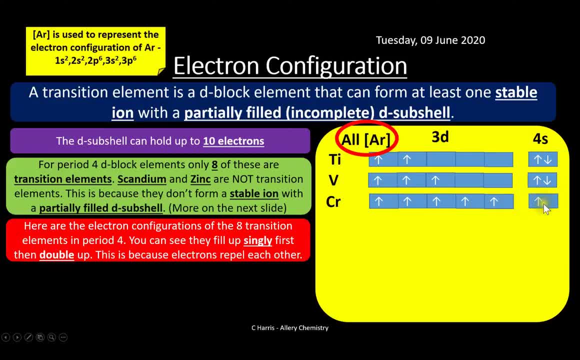 move fairly readily between 3D and 4S, and so actually this configuration is more stable than having the four electrons on their own and two in there. So this is the most stable configuration, And the next element is manganese. So manganese, here we put the electron back. 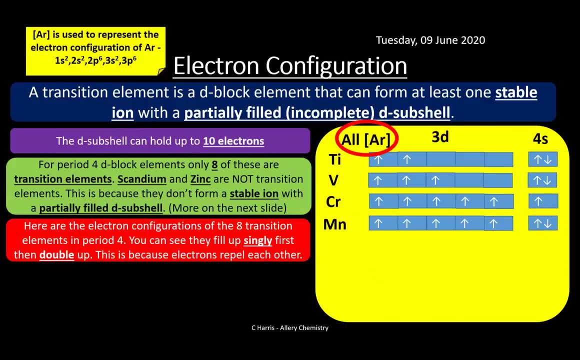 into the 4S orbital. again here, The next one is going to be iron. So now, you can see, at this point we now have to pair up some of these electrons because there's no other space for them to go. So iron is that, and then we've got cobalt, which is that, and 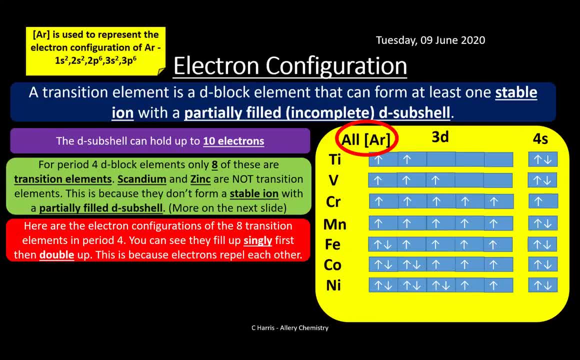 then we've got nickel, which is that one there. Now another one. here's another strange one. You can see, now we have a position similar to chromium, where we have, if we add a little bit of electron in there, we can have, or we can form a full 3D sub-shell which is stable. 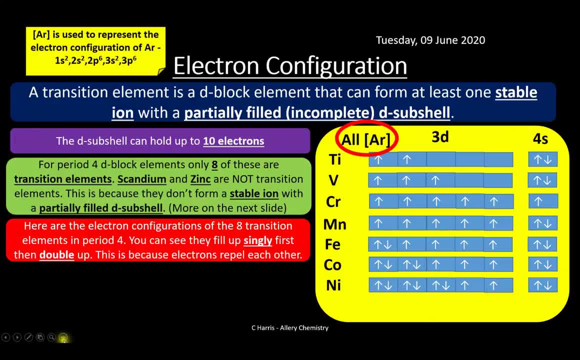 but one of the electrons in the 4S has to jump into this orbital here. So that's what happens with copper, which is there. So there's two things to watch out for. here you've got the copper and you've got the chromium electrical configurations, which are slightly different. 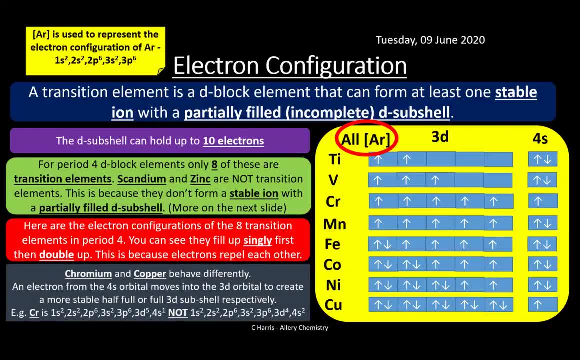 So that's the key thing that you've got to remember: They don't have the electron configuration. so, for example, this is for chromium. Chromium doesn't have the electrical configuration. okay, where it's got 4s2, 3d4, it's 3d5, 4s1. so one of the electrons jumps into the. 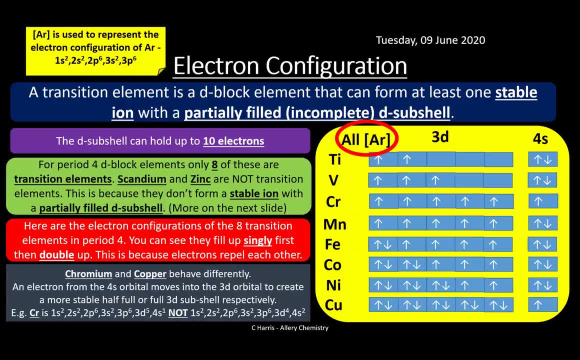 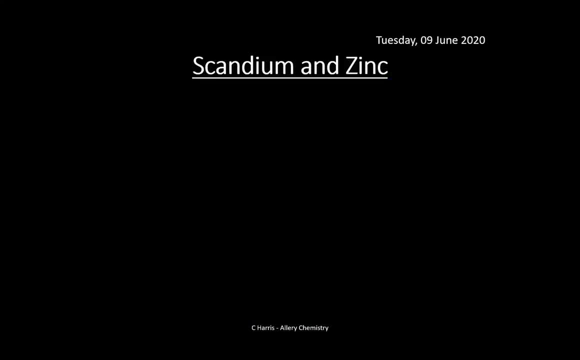 3d orbital because it's more stable. okay, so just make sure you're fully aware of that, because that's a bit of a pitfall that they could pick you up on. okay, so let's look at scandium and zinc. so, remember, we told I told you about these. 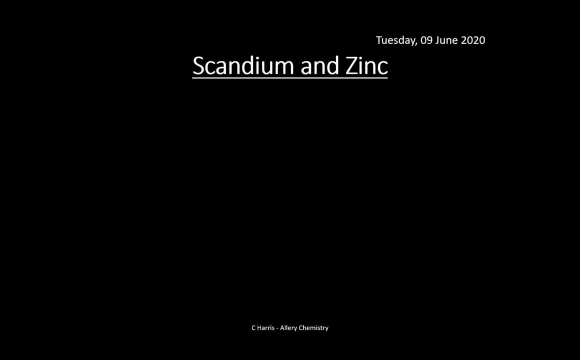 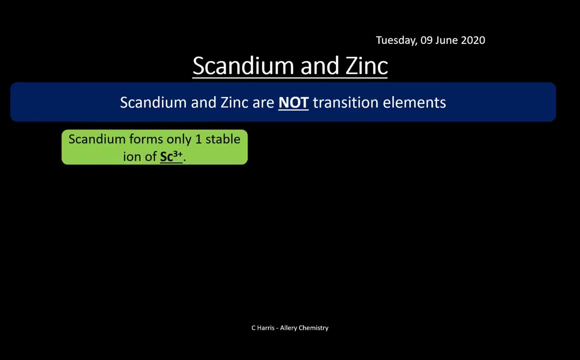 two elements in particular. so these are D block elements, but they're not transition elements, so we're just going to kind of dig into this a little bit more. okay, so scandium only forms one stable iron, which is sc3 plus. that's the only stable ion that it forms. so this has an empty D subshell. okay, so we take. 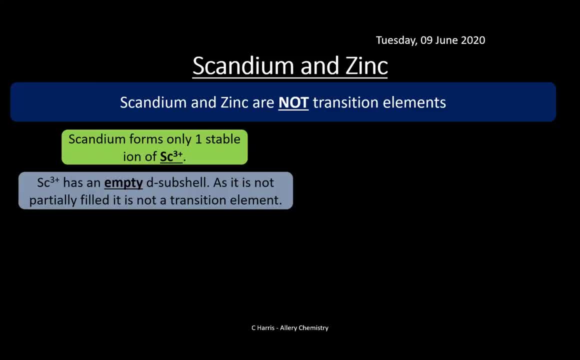 three electrons away from scandium. so if you imagine it, the electric configuration, we take one from the 3d and the two 4s ones and that means you don't have any electrons at all in that 3d subshell. so because it's not partially filled, then 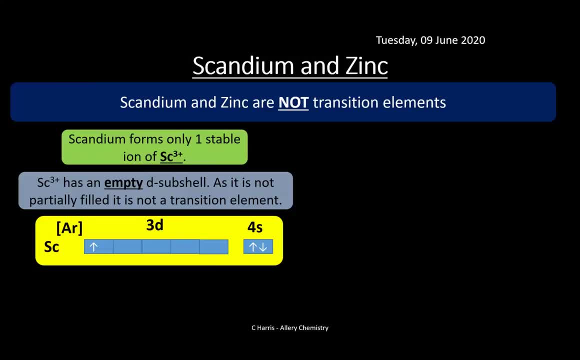 there is. there's your electric figuration. it's probably better for show you, isn't it, rather than just imagine it, and so you can see there. that's the electric configuration for scandium element, but the ion, the only stable ion, it forms, is scandium 3 plus, and you can. 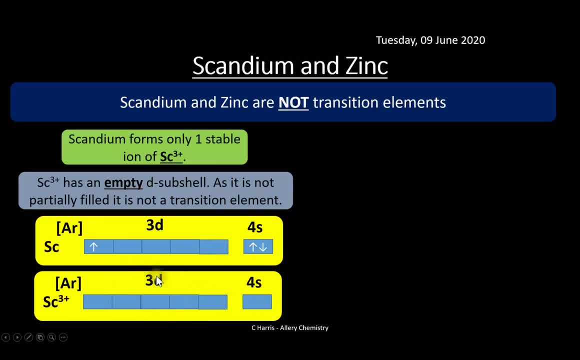 see that is empty, so it's not partially filled. so because the 3d subshell is not partially filled, that means scandium is not a transition element, and likewise that goes with zinc as well, so zinc's at the other end of that, of that, of that. 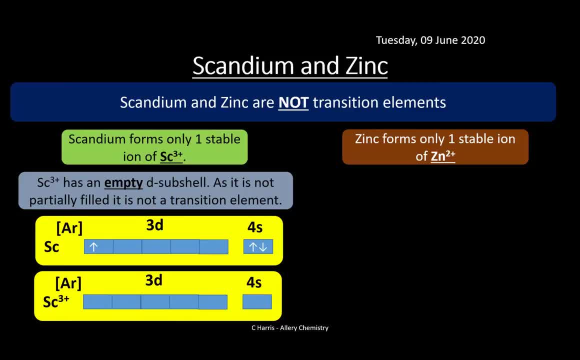 role there. so zinc only forms one stable ion, which is zinc 2 plus. so zinc 2 plus has a full D subshell. as it's not so, it has a full D subshell. so that means it's not a transition element. now the reason why is, if we look at our electric configuration, 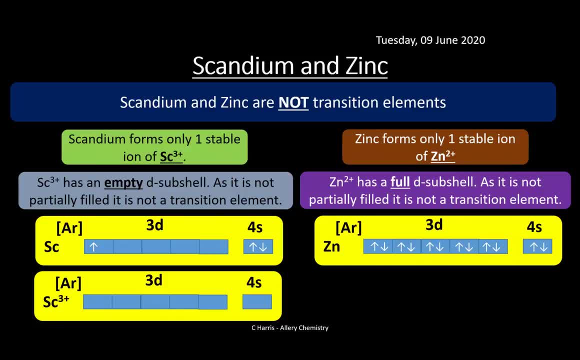 of zinc it's full. so we've got 3d, a full 3d and a full 4s. but actually- and we'll see this a little bit later on as well- when we remove electrons from an atom, we remove them from the 4s first, then the 3d. so the effect on zinc is it still has a full 3d. 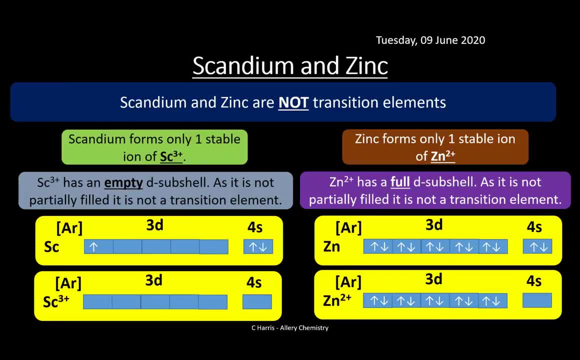 subshell, the 4s. one has no electrons in there whatsoever, okay, so, very important, when we're removing electrons, we remove them from the 4s first, then the 3d, okay, so that's really, really important. when we're looking at ions- and this is the 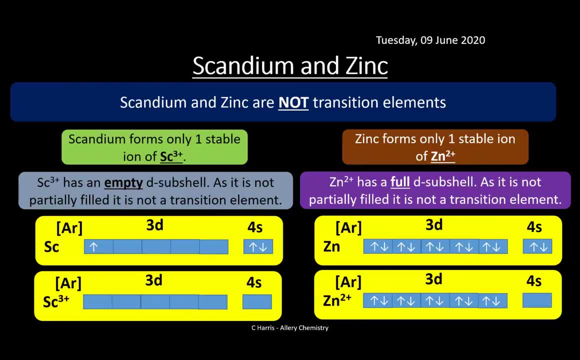 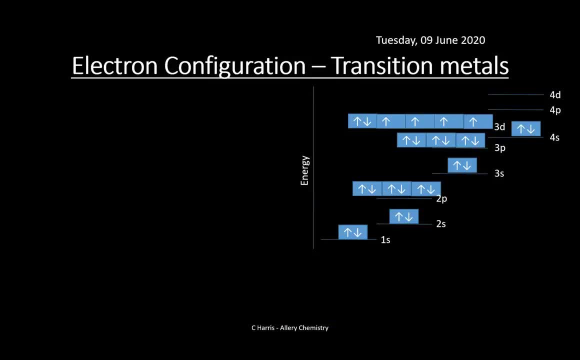 reason why scandium and zinc are not transition elements, but they are D block elements. okay, so let's look at this in a little bit more detail here. so what we've got is an electron configuration or electron diagram showing orbital energies, and you can see here this shows it a little bit better than the original. 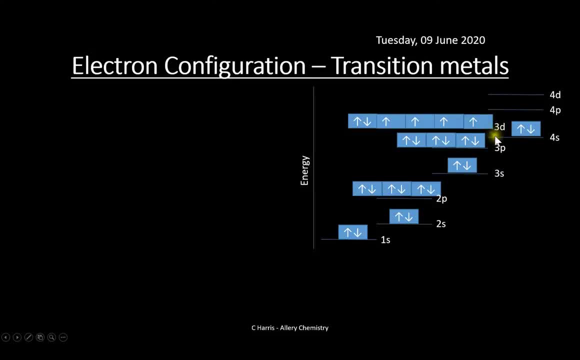 electron. so it's a little bit better. where you've got 3d and 4s are kind of very similar in energy. okay, the energy levels here are very similar, so the electrons can move quite readily between them. so what we're going to do here is 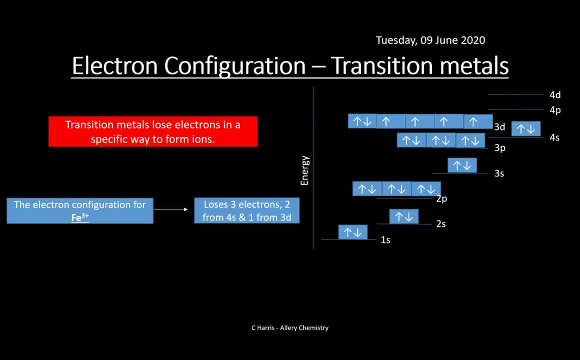 we're going to look at how transition metals lose electrons, a little bit like what we've seen with with zinc. this is just to confirm it. but if we look at the transition metal in particular for iron, so the electric configuration for one of ions, ion, is Fe 3 plus, and Fe 3 plus is formed by the transition metal and the 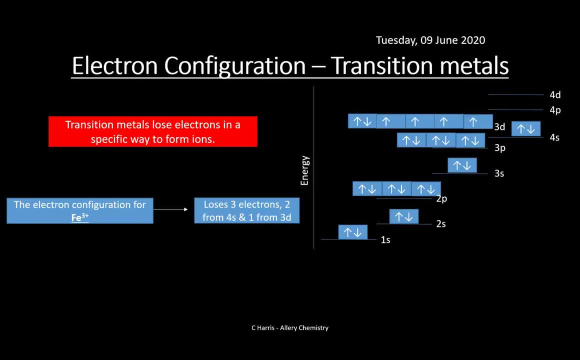 transition metal is formed by the transition metal, and the transition metal is formed by the transition metal is formed by losing three electrons, and so the electrons are losing three electrons, and so the electrons are lost from the 4s first. so two electrons in the 4s and then one from the 3d. so this is what we. 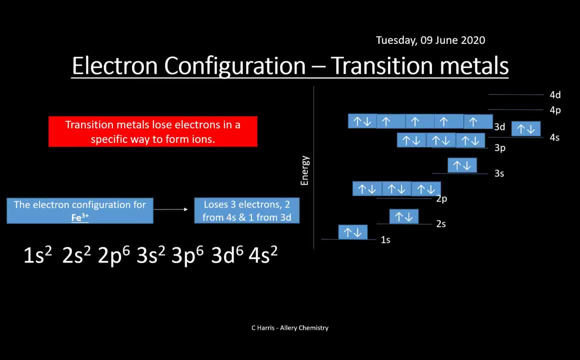 should have. so you can see here that we've got the electric configuration of ion, which is there. now if we remove three electrons we end up with this configuration. there we are okay. so we end up with 3d 5. now that is a partially filled d subshell. so ion is a transition element. so that's so that's. 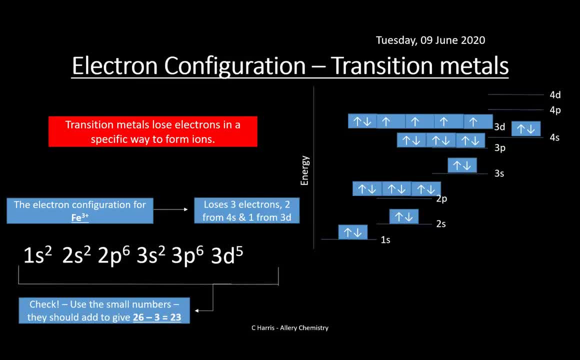 that's fine. what you should always do is check. okay, so use the smaller numbers on here. tells you the number of electrons in this atom here. that's what the smaller numbers tell us. so using the smaller numbers they should give us. so it's 26 is the number of electrons in iron atom. we're. 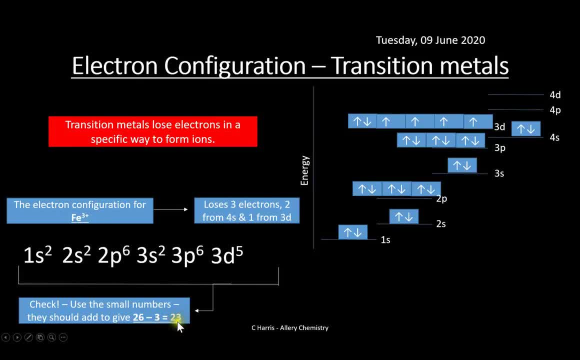 going to take three electrons array and we're going to have 23 that's left over. so add these smaller numbers up and they should add up to 23. so just make sure you've got that, okay. so we loosen the 4s in terms of the diagram, there it is, and then we take it from the 3d. so that's the diagram. 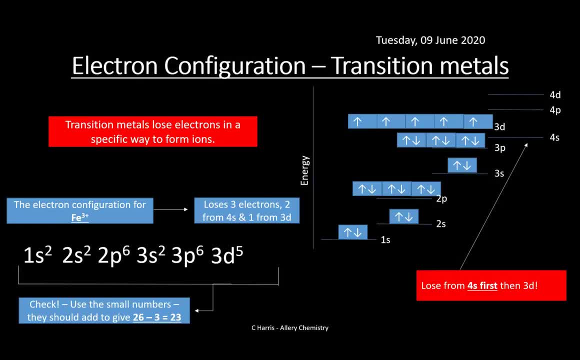 for iron 3 plus. okay, as long as you remember that remove from the 4s first. you must empty that first, then the 3d. okay, so that's when we're ionizing or removing electrons from it. okay, so let's look at. so we've looked at the electron configuration, we've looked at the 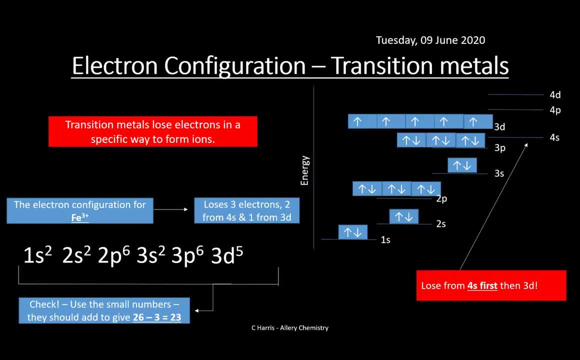 um, we've looked at the structure of you know well what's a transition metal and what's a d block element, so we distinguish between that. so now what we're going to look at. we're going to really focus quite a lot in this video, understandably on 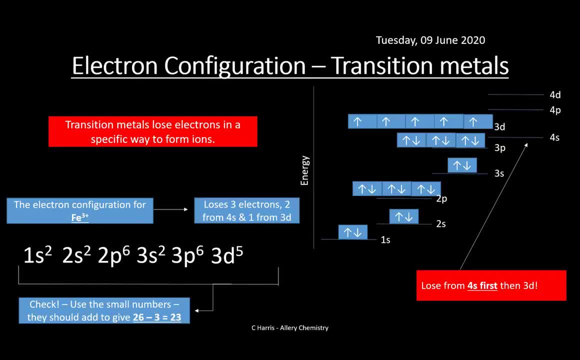 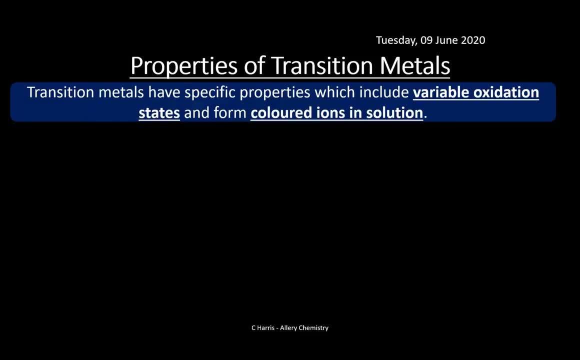 transition metals rather than just scandium and zinc. so what you need to know are the properties of transition metals. so transition metals actually have some quite unique properties and this, this kind of whole um module of um developing metals. so the dm topic is all about metal. so it's all. 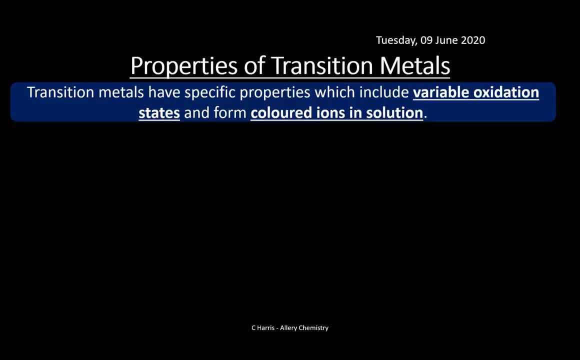 going to be about transition metals and and and their reactions, or other metals and their reactions. so transition metals have specific properties, which include they have variable oxidation states and they form colored ions as well in solution. okay, so we're going to look at quite a lot to do with colors, a lot of color in. 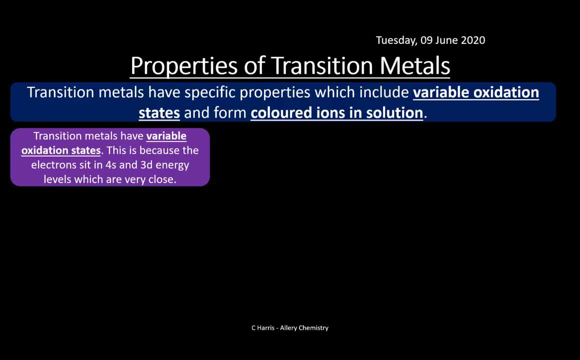 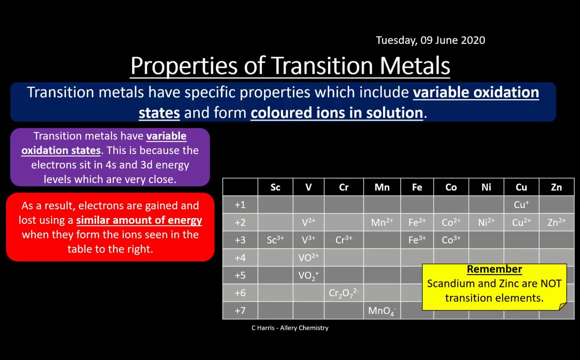 this one. it's a nice, nice topic. okay, so transition metals have variable oxidation states and this is because- remember what we said before, that 4s and 3d energy levels are actually really close to each other. okay now, as a result, the electrons- uh, electrons are gained and lost using a similar amount of energy. uh, when they form the ions seen. 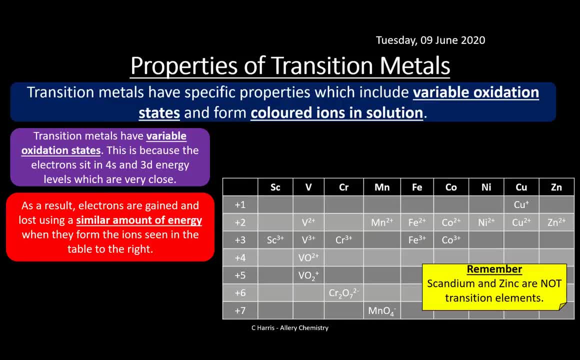 in the table to the right. so you can see here that we have various different ions are formed um depending on the transition metals. so this is just some of them here. obviously, remember zinc and scandium. these are not transition elements. these are the only stable lines they form, but the rest 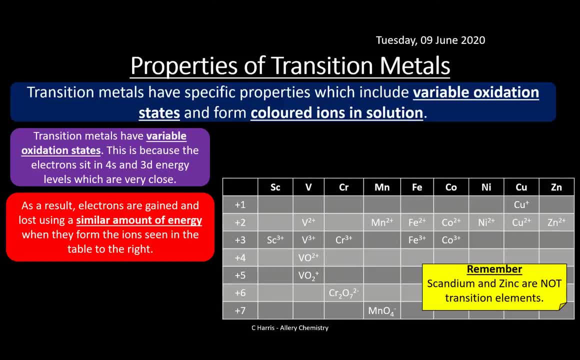 are transition elements, as you can see, uh, in between there now, the ones that you need to know. thankfully, you don't need to know all of them. the ones that you specifically need to know are the ones that are circled okay, so you need to be aware of the copper and the iron ones there and, in particular, you need to. 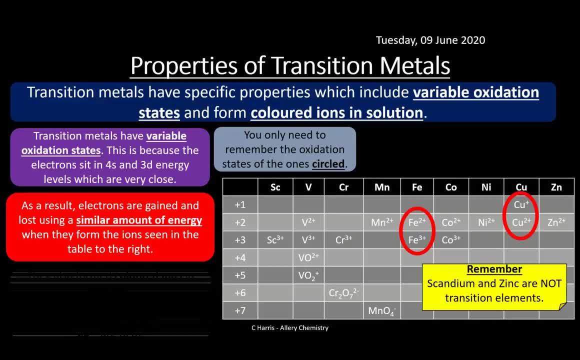 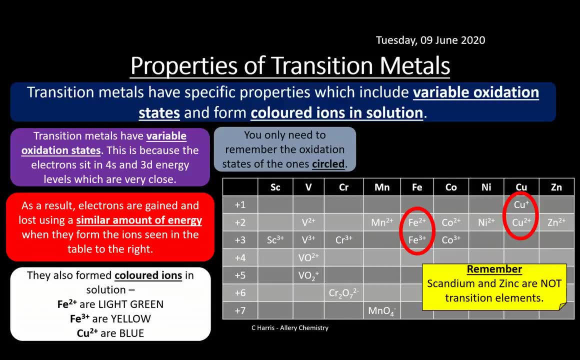 know the colors of these when they're dissolved in solution. so here they are, so you can see um the colored ions is. iron, 2 plus is light green. so you need to know that fe2 plus is light green color when it's dissolved in water. fe3 plus like a yellowy orangey color, and when they're dissolved 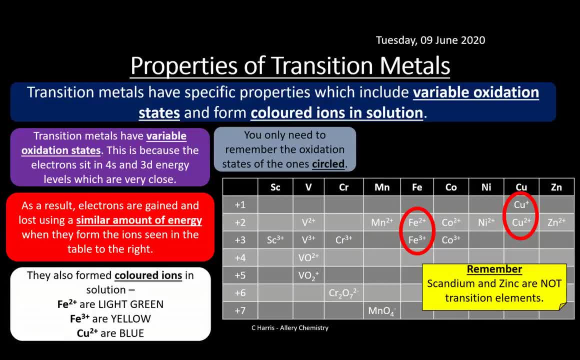 in water and copper 2 plus is blue. now the copper 1 plus. this is unstable. so copper plus is unstable in solution and what will happen is this will readily disproportionate into cu2 plus and copper readily. so although you know, you do need to know about the copper plus. you do need. 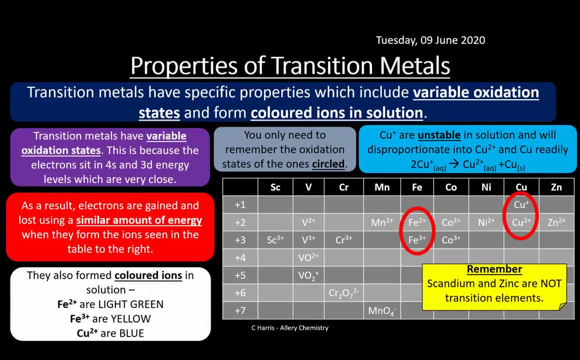 to know that that readily um, um disproportionates, which means the oxidation. basically it's this element here- is reduced and oxidized simultaneously. so you can see here it's been oxidized to form cu2 plus and it's been reduced to form cu, as you can see there. so you can see that 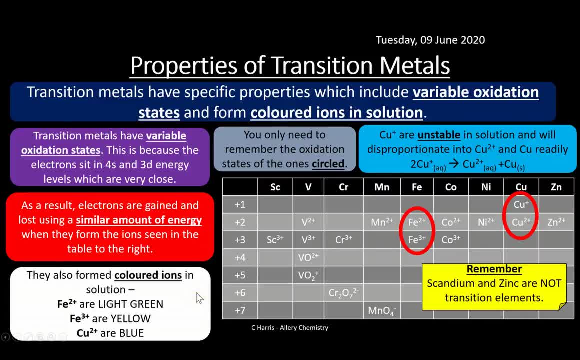 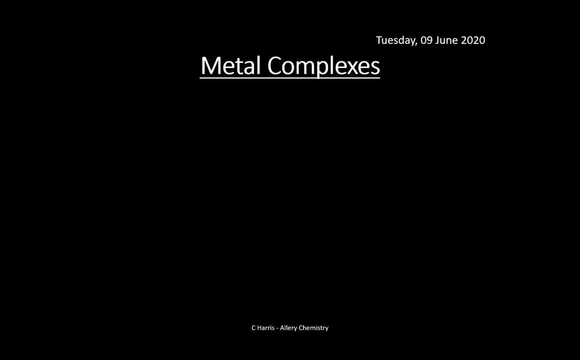 this one's unstable, so it disproportionates into these two species there. as long as you're aware of that, that's all you really need to know with copper plus, but you do need to know the colors of fe2 plus, fe3 plus and cu2 plus. okay, so let's look at the complexes. so one of the one of the um. 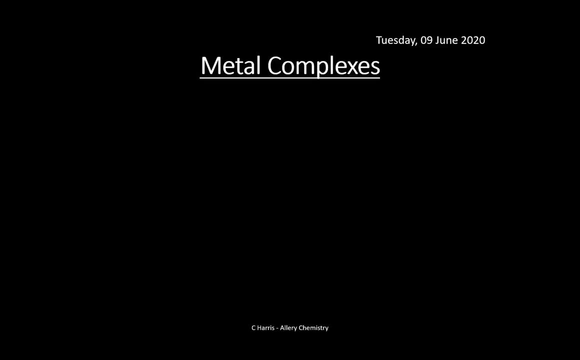 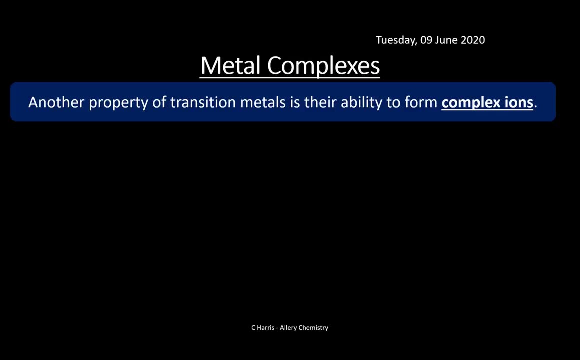 one of the features of transition elements is they're able to form complexes. now they sound complex. sounds complex, doesn't it? um, it's not. it's not actually that bad. it's fairly straightforward. um, it's a common property of these and it's a very useful one, as you're going to see later, we're going to 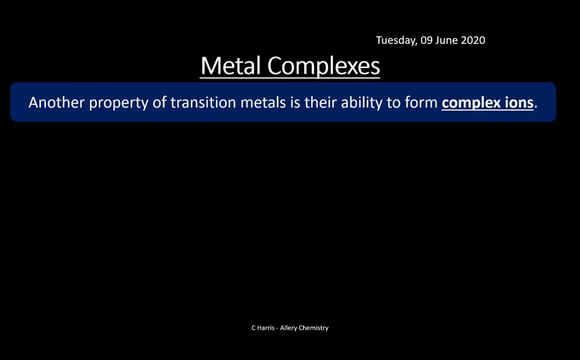 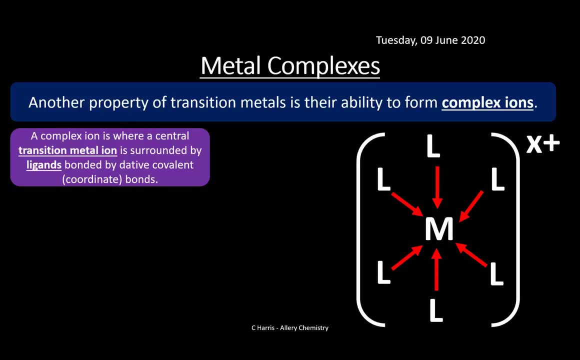 look at what these complexes look like. but um- the ability to form complex ions- is quite unique to transition to transition elements. so a complex is basically um, or complex ion is where we have a central transition metal ion and it's surrounded by ligands bonded by dative, covalent or coordinate. 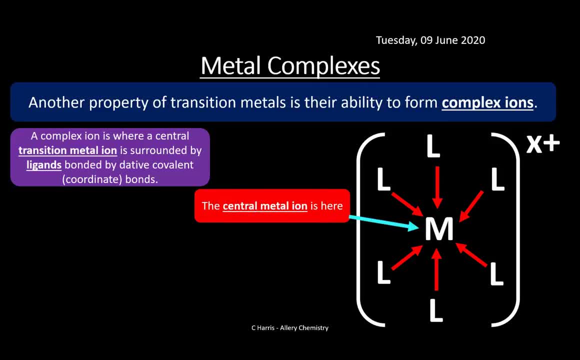 bonds. okay, so this middle bit. here there's your central metal ion in the middle. this is what the complex looks like. the red arrows actually show um dative, covalent or coordinate bonds, and this is where electrons come from one species. in this case, it will be the ligand and they're donated to. 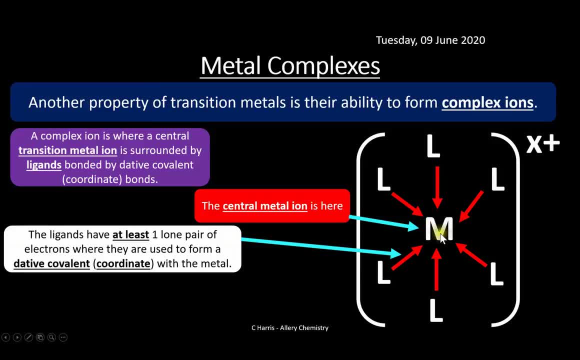 the central metal, uh, central metal ion in the middle here. so that's quite unique in terms of. they form this coordinate bond, this dative covalent bond. okay, complexes as well. um, um, generally not always, but they have a charge, um, as you can see on the top there, um, and they 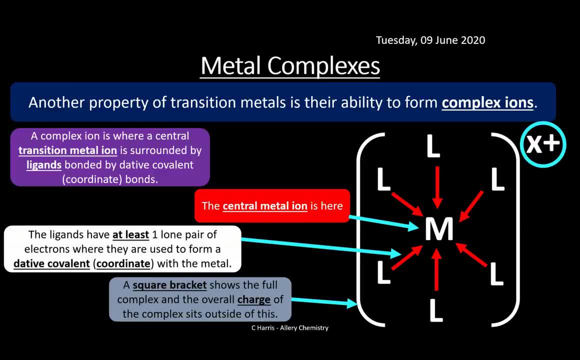 actually have a square bracket and the square bracket basically shows the overall charge of the complex. okay, so you can see here that we've got um ligands here. these ligands may have a charge or they may not, depends on what that is. we'll look at ligands in a minute. um and then. 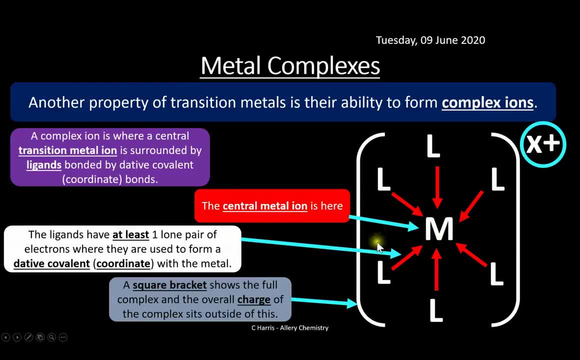 the metal line itself may have a charge. so if we basically um add all these charges up, we get an overall charge of the complex. now, sometimes the overall charge might be nothing, in which case there isn't a charge there, so it doesn't always have to be one there. okay, so complex ions can. 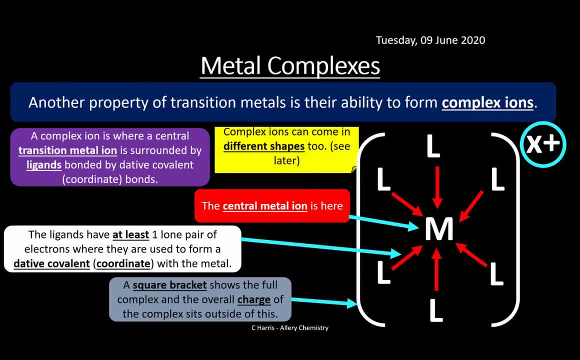 come in different shapes as well, um, but we'll look at the shapes of these complexes a little bit later on. so, as long as you aware of what a complex is, that's basically a complex. it's like a big molecule with a metal line in the middle and we've got ligands and l stands for ligands. 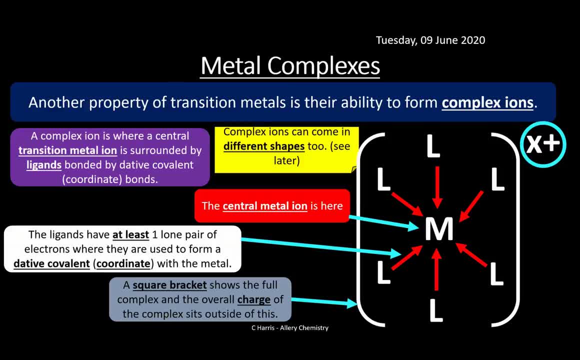 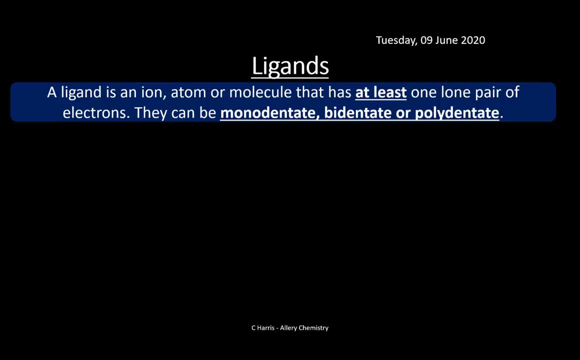 which go around, and actually that's what we're going to look at now. what these ligands are, um, okay, so a ligand is basically just an iron, an atom or a molecule that has, that has, at least one lone pair of electrons, and they can be monodentate, bidentate or they can be poly. 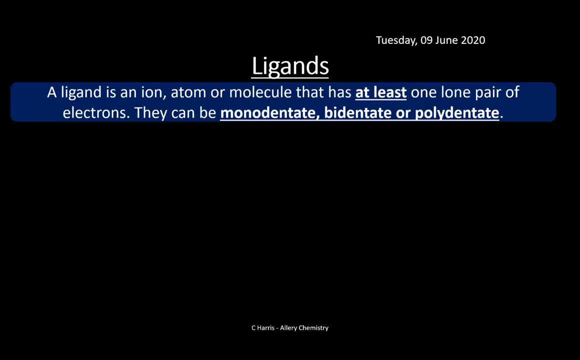 polydentate, monodentate or unidentate, so they're the same thing. so monodentate, bidentate or polydentate, okay, so ligands have this unique, well, this very specific property which has must have a lone pair of electrons, because it's going to form a datacomponent and it's going to form a 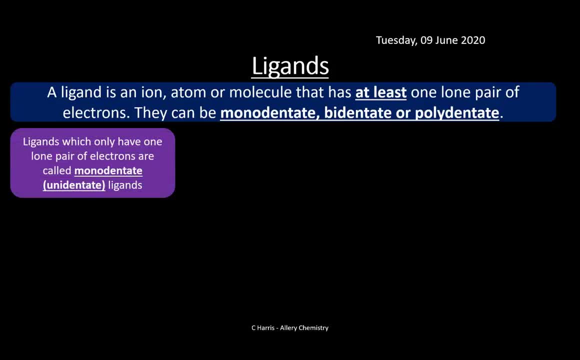 covalent or coordinate bond with that central metal line. so ligands which only have one lone pair of electrons are called monodentate or unidentate ligands. so specific examples that you need to know are: water, so h2o is a monodentate ligand, ammonia, which is nh3, as you can see there. 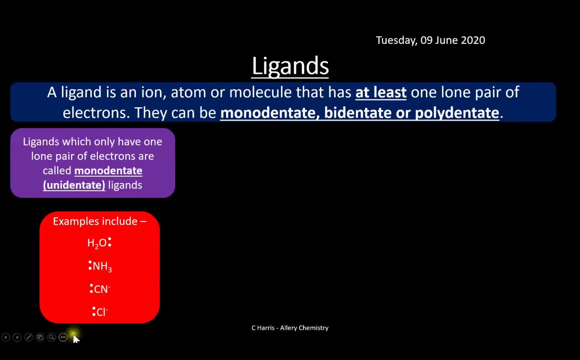 there's nh3 cn minus the cyanide ligand and a chloride ligand. so these are all monodentate or unidentate ligands. okay, so they only have one lone pair of electrons that is unidentate and they're used to form a date of covalent bond with the metal line. so ligands which have two lone pairs. 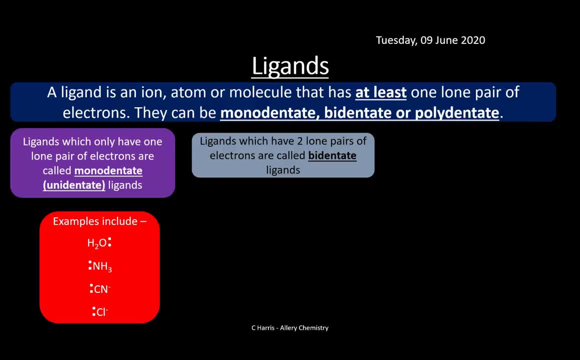 of electrons are called bidentate ligands, and there's specific examples that you need to know are: ethane, diuret, as you can see there, it's just like a carboxylic acid, a dicarboxylic acid, sorry, um, with a lone pair, obviously on the oxygen. and we also have uh, ethylenediamine or also. 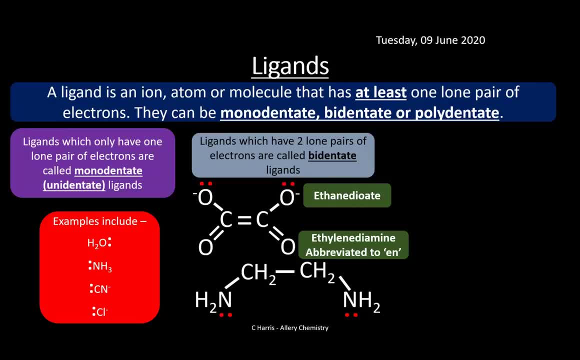 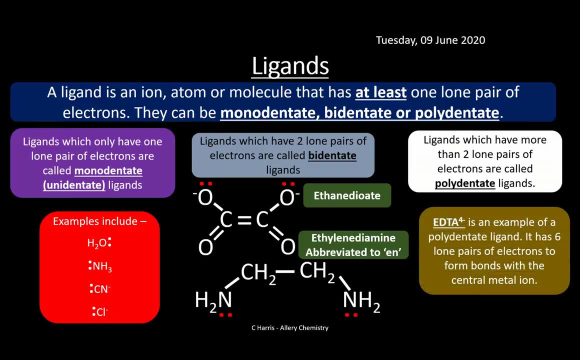 abbreviated to en. so using en is just a bit quicker than writing all that molecule out. okay, so ligands which have more than two pairs of electrons are called polydentate, um polydentate ligands. so these are. a classic example which you do need to know is edta, so edta4 minus. 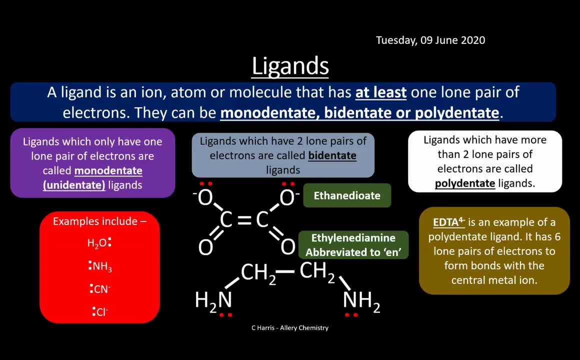 is an example of a polydentate ligand. it actually has six lone pair sites which it can bond onto that um central metal ion in the middle. so it's quite a big ligand. it's massive. it literally surrounds that metal ion in the middle. so this is a polydentate ligand. 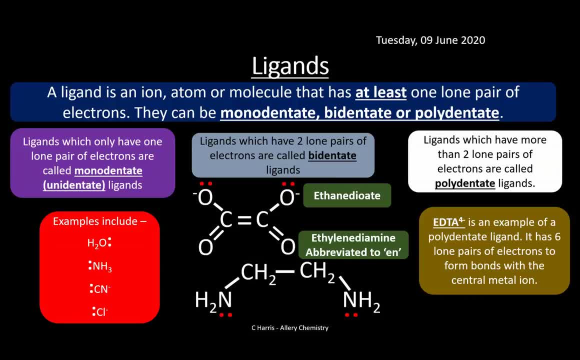 poly meaning bonds more than once, okay. so multiple times poly, okay. so now we know what a ligand is, we now need to attribute these ligands. remember what we said about the shape as well. the shape, the shape of the complexes can change, but what we're going to do is look at these ligands and, and how do? 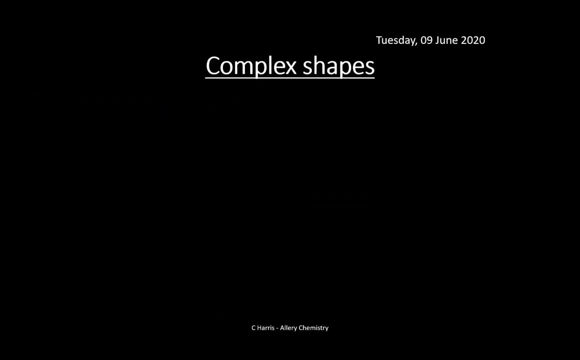 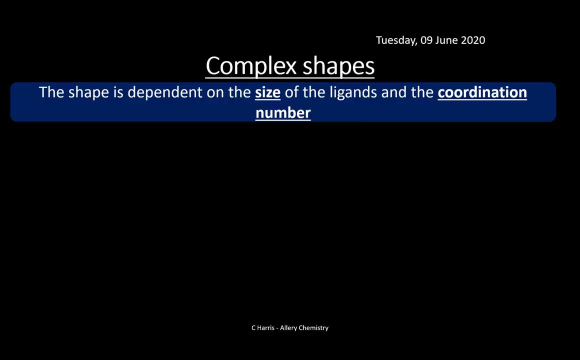 these ligands help to determine the shape of your complex. okay, so let's look at complex shapes. so the shape is dependent on the size of the ligands and the coordination number as well. now what you get confused. you can't mix up coordination number and ligands. okay, there's a big difference, but we'll. 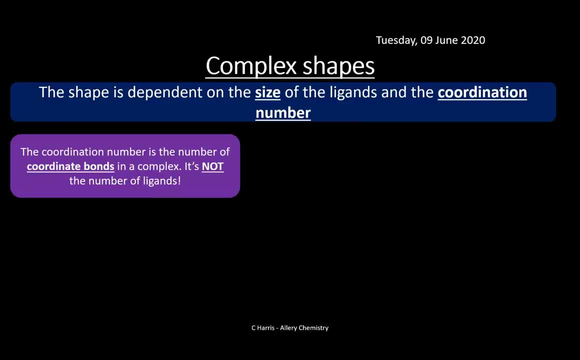 look at them. so the coordination number is the number of coordinate bonds in a complex, it's not the number of ligands. okay, so coordination number, coordinate bonds, number of coordinate bonds, not the number of ligands. so you might have, for example, edta can form four coordinate bonds. 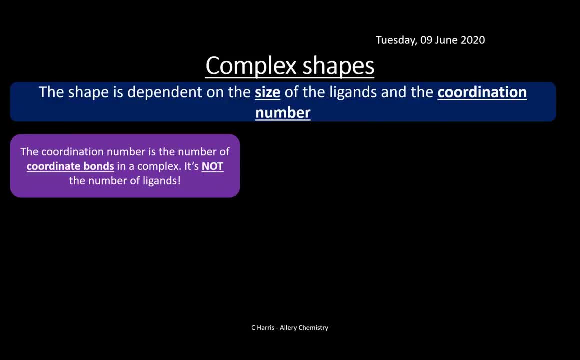 okay, so it has a coordination number of six, but we only have one ligand because edta is a large ligand. so let's have a look at um this, the size of these ligands, because the size is important here. so some ligands are small and small ligands. you can fit six of them around that central. 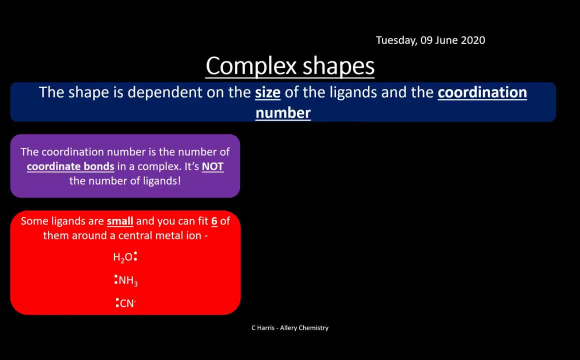 metal line, such as water, ammonia and cyanide. these are classed as small ligands, okay, so you can fit a large, a lot of them around there. so i'm going to use this analogy of a bit like um pigs around a trough. so you've got a trough and the trough is like the metal line in the middle. 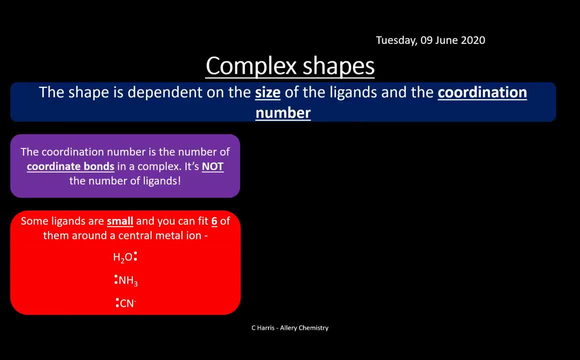 and you've got the pigs which then feed from the trough. okay, this around the trough. Now, if you've got tiny or small pigs, then you could fit more of them around that trough, but the troughs are fixed size. okay, so the baby pigs or piglets, should i say, um, these actually, um, you know you. 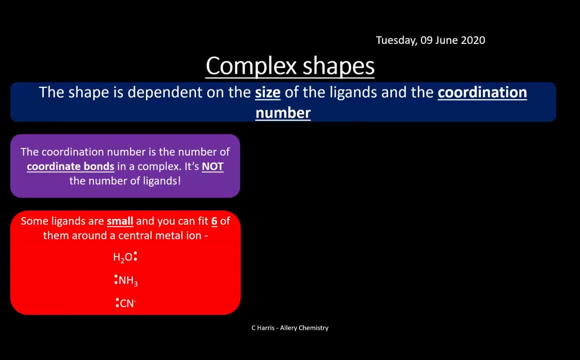 can fit six of these around that trough so they're classed as small ligands. so bigger ligand is chloride ligand. so the sale minus is bigger now because it's bigger. we can only fit four of these round, so that's a little bit like um bigger pigs. you can only fit four pigs around this trough. 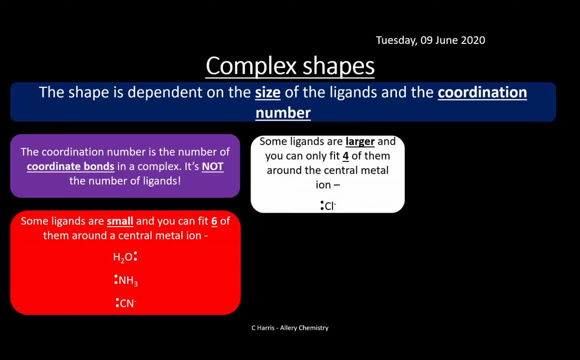 because there's simply not enough space to fit mountains, so you could only fit down a kick inside them around. so chloride ligand, or cl. minus, is classed as a larger ligand and you can only fit four of them around. the metal ion and finally, um. the other ones are your bidentate ligands, such as: 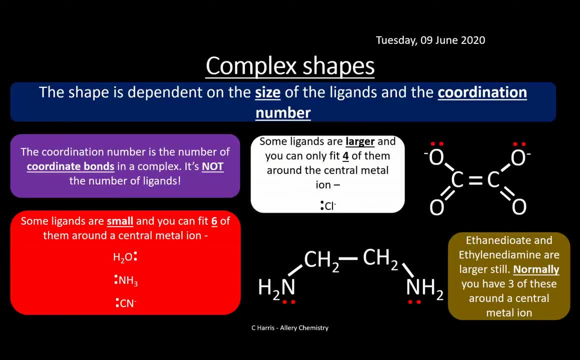 ethane diuret and um ethylenediamine as well. these are larger again, as you can see. they're a bit more bulky and normally we can only fit three of these around the central metal ion. so these are even. these are like fatter pigs trying to squeeze around this trough. we can only fit three of them. 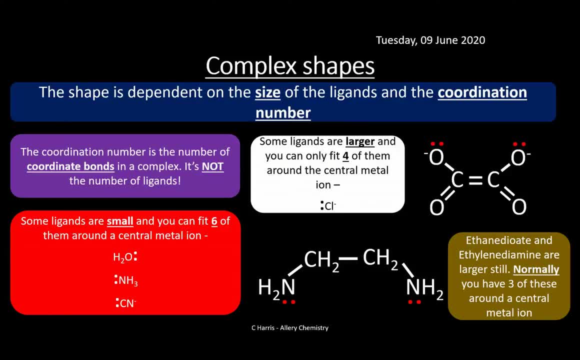 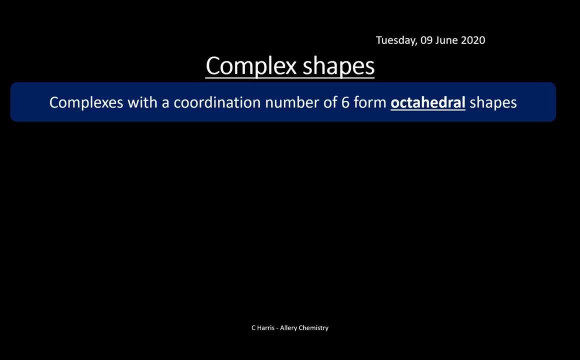 um around around the metal ion. okay, so that's important because the size of the ligand is now going to determine the shape of the complex that they form when we have them. okay, so let's have a look. so complexes with a coordination number of six: these form octahedral shapes. okay, so for 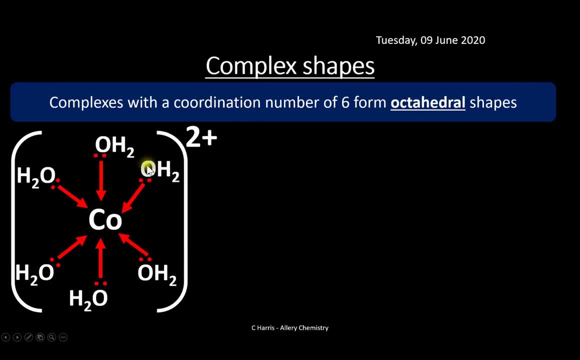 example, we've got a cobalt metal ion in the middle here and we've got a small ligand- this is water um- surrounding the cobalt ion in the middle, and this can also be written as this and you're going to see this quite a lot when we look at some of the equations later on. 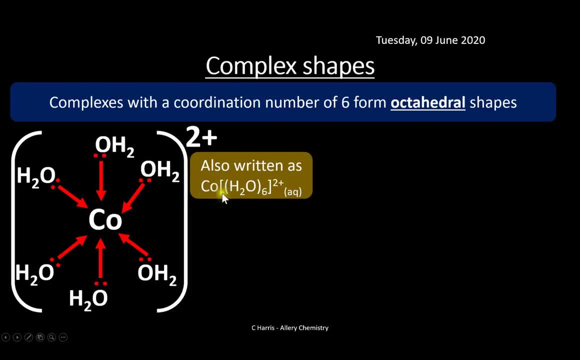 where we write the transition metal, which is cobalt, and then, in square brackets, we then put the ligands that are surrounding it. so in this case it's going to be six water ligands surrounding this. so this is just cobalt put into solution. okay, the overall charge is two plus on here. 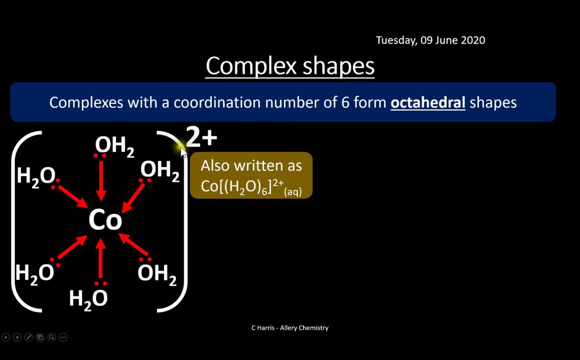 okay, so we can work this out. actually, we'll quickly go through this. we can actually work this out by: um, water has a neutral, has no charge. we know that water doesn't have any charge. we've got to have as many waters as you like and that's not actually going to change the overall charge. 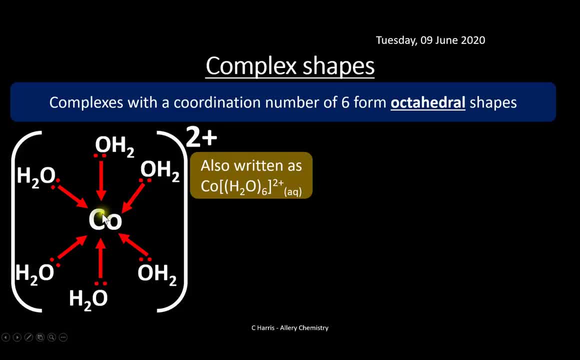 so this charge is actually coming from the charge of the metal line in the middle. so that must be two plus in the middle there. so let's have a look at another example. this is ammonia, and we know ammonia is a small ligand as well, a bit like water. so we can fit six of them around the cobalt, uh in. 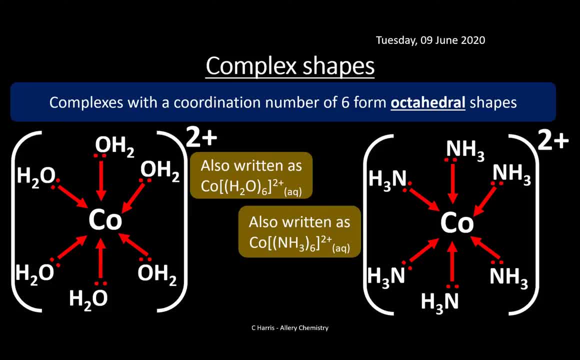 the middle there and clearly that can also be written like that. okay, so very similar to the water one. as you can see now, these are octahedral. now you may remember from year one chemistry and looked at shapes of molecules. octahedral shapes have a bond angle of 90 degrees between each. 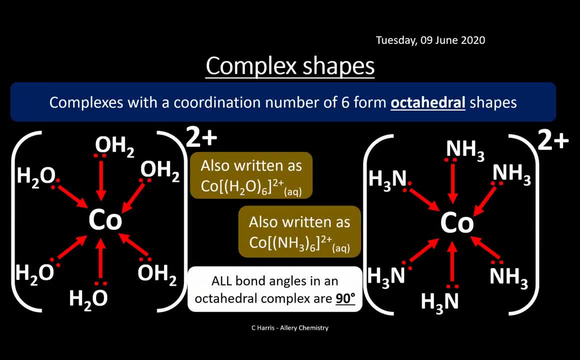 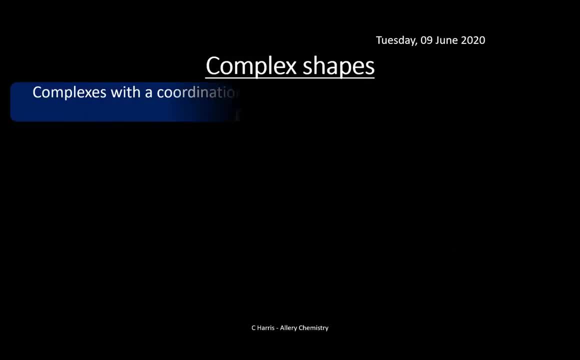 of them no different from what you've seen in year one, chemistry. we're just applying this to transition metal complexes instead, so that's an octahedral shape. so we've got six of them around there. so complexes with a coordination number of four form tetrahedral and square planar shapes. 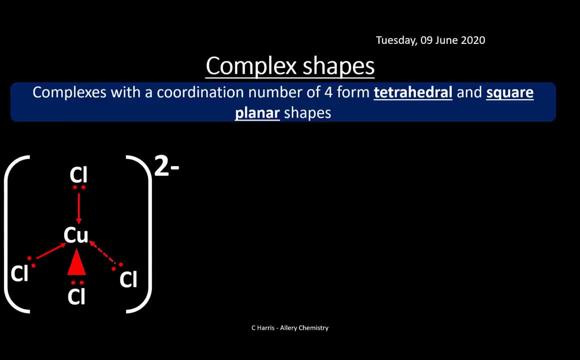 okay, so let's have a look at this one. so here's an example here. this is a copper with chlorine ligands around it. so remember, chlorine is a bigger ligand, so you can only fit four of these around the central metal line. now notice the charge on here. just to kind of um it's also. 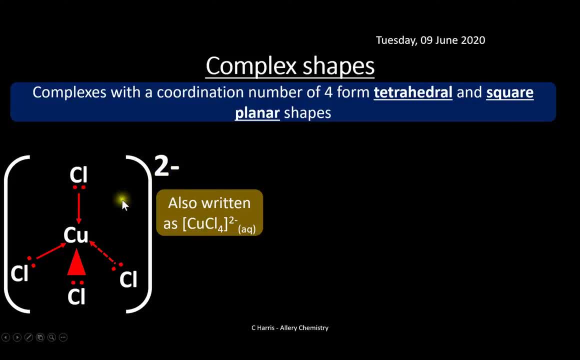 written as this as well. but just to kind of go through the charges. then chlorine: we know cl is cl minus. now we have four of these cl minuses there, so that's four minus overall. the charge in the complex is two minus. so that means that this must be plus two, so that's cu two plus that. 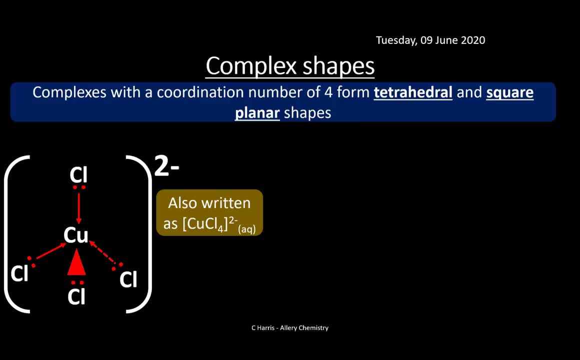 is a two plus charge in the middle. so that's the charge in the middle. so that's the charge in the middle there. okay, now because this is tetrahedral. the bond angle in tetrahedral is 109.5. again, that's something you would have picked up on in year one: chemistry. looking at the bond angle of tetrahedral. 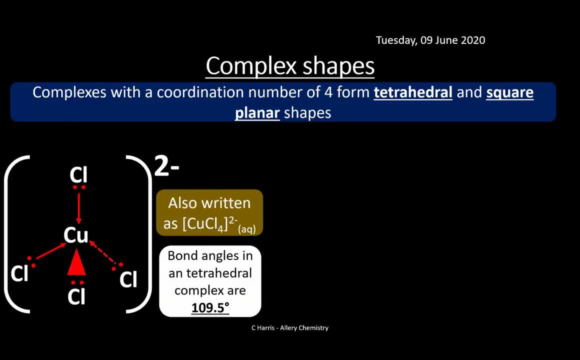 complexes. so another one which you will have come across is square planar. now there's a specific example you do need to know, which is um this one here. so this is platinum, with two ammonia ligands coming at the bottom here and two chlorine ligands. don't worry, always default to tetrahedral. 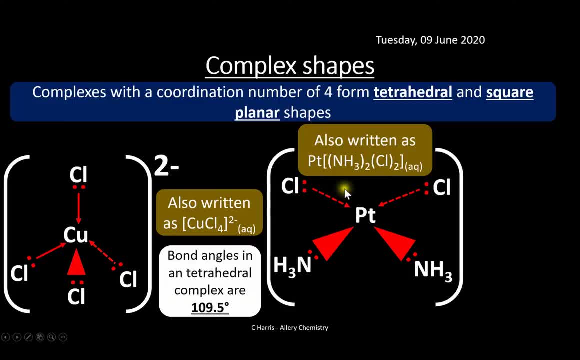 unless they state otherwise, or unless it's this, which is also known as cisplatin. okay, so cisplatin is an anti-cancer drug, so this is a specific example that you need to know, and you need to know that this cisplatin is square planar. you are expected to know that. okay, so this is platinum. 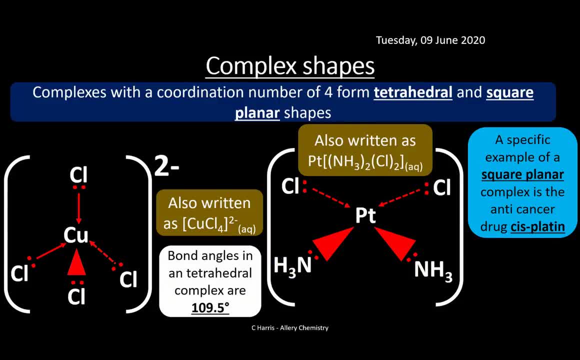 two chlorine ligands at the top and two ammonia ligands towards the bottom. there now you'll know from year one chemistry that the bond angle in square planar- uh, square planar- complexes are going to be, and you'll notice that the bond angle at the bottom is going to be in the right direction. 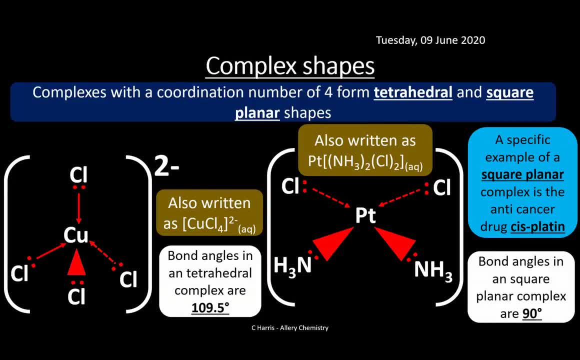 so your structure is that direction of the center of your structure. so if you were to draw a line- and we're using this as a square plane- that's going to be a slightly smaller square plane and obviously you know the uniformity of the structure perfectlyнул the bond angle that you 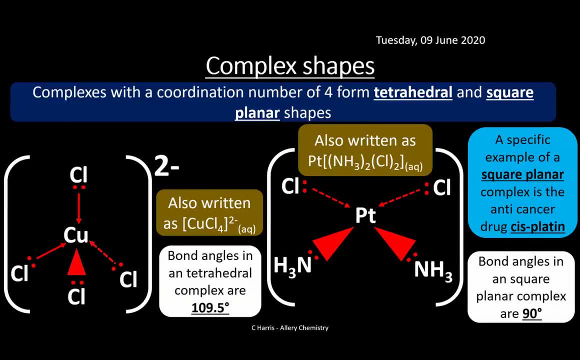 know, if we were to draw a line, a square plane, and we wrote it at the bottom, we were going to draw a three square line and if we draw a line, two square lines, that's going to be equal to square point three degrees. okay, so you have this flat shape there. there are flats complex and you'll 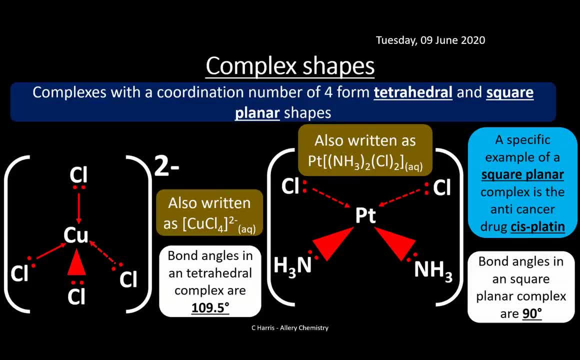 notice with the with anything to do with 3d diagrams. we have wedges and we have dotted lines, the wedges, the overall charges and how we work that out. and one of the key features as well of transition metals, as we've said, or transition metals, is color okay and we need to understand how do. 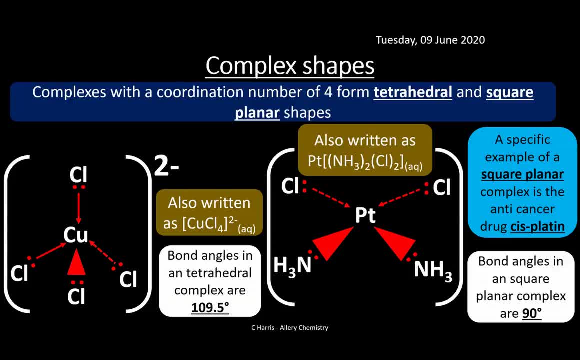 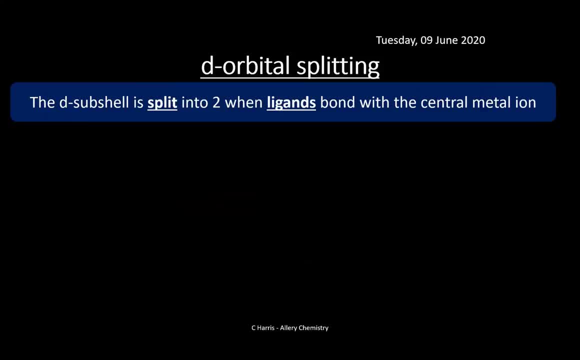 ligands or the type of ligands affect the color of what we see. okay, so this is all down to something called d orbital splitting. okay, the d subshell is split into two when ligands bond with the central metal lines. remember, we looked back at the electron configuration. we'd seen we had the 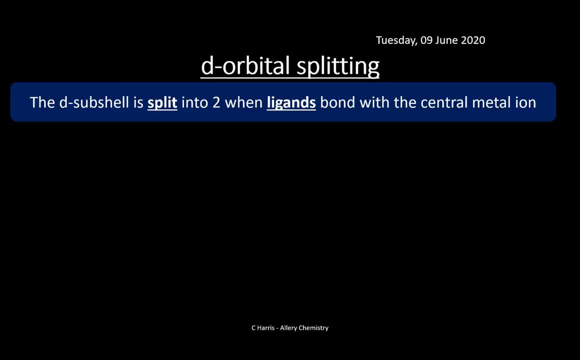 three. we had the d orbitals, the 3d orbital, the 4s orbital. so we just shown you before. um, the orbital is actually just in a row, it's linear. what actually happens is when we bond the ligand to that transition metal, the d orbital actually splits. so this is the linear configuration that 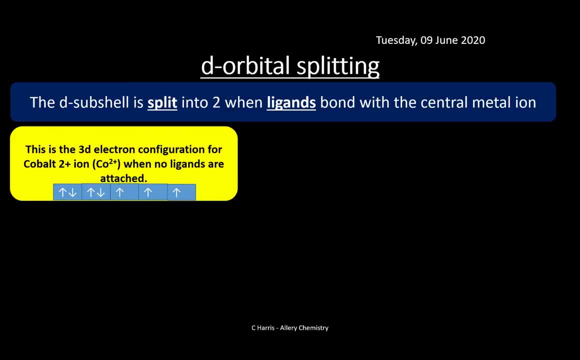 you've seen before. so this one's cobalt, cobalt 2 plus. so this is just hypothetically. this is saying that um you that we have no ligands attached, then the d orbital is actually in a nice neat linear arrangement like this. there's no splitting of that d orbital, but the moment we add a ligand to it, something, 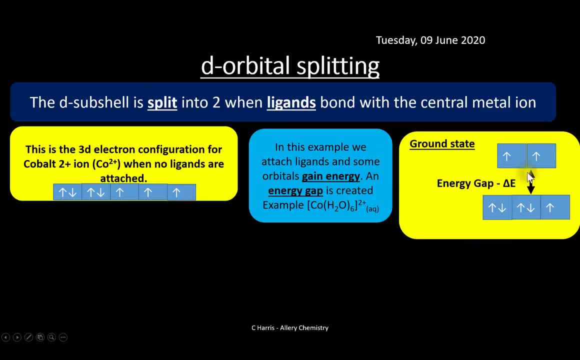 weird happens here, um, and what happens is the d orbital actually splits into two, as you can see there, um. so you can see, here we attach some ligands and some of the orbitals gain a little bit more energy. so they're a little bit higher up, as you can see there, than these orbitals here. 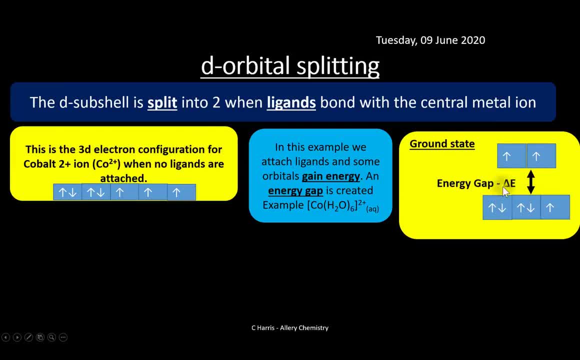 and we create an energy gap, which is delta e, which is this bit here. okay. so, for example, cobalt um, um dissolved in water to form your cobalt hexa aqua complex, which is this one here. okay, so we get this splitting of it now. this is: 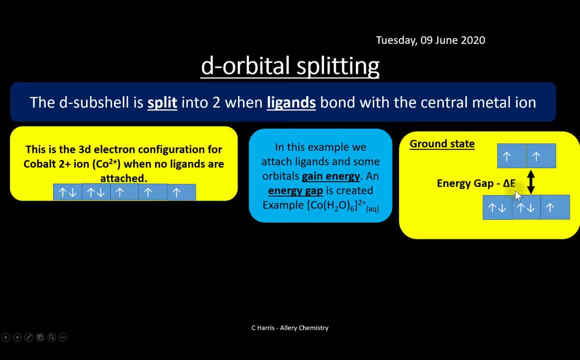 called a ground state. so, in other words, we've got some of the electrons here go to the top and three of them are at the bottom, which is here. okay, so this is the ground state. we're gonna- i'm gonna- come on to what we mean by ground and excited state. we'll look at that in a moment, okay, so? 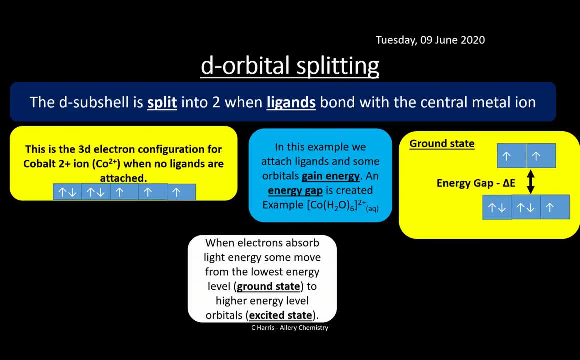 when electrons absorb light energy, some of them move from the lowest energy level, the ground state, which is this configuration here in the yellow box, that's all of that- to a higher energy level state called an excited state. so let's have a look at what we mean. so there it is. so there's. 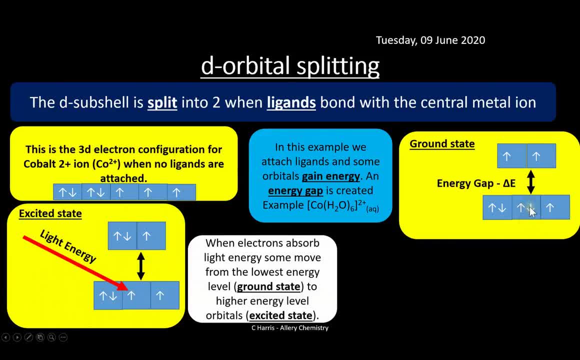 your excited state so you can see here that what's happened is in the ground state. we've had two, two and one in the bottom here. but when we give it a little bit of energy, so that could be light energy for example, then this electron absorbs some of that energy and it jumps up into the higher energy. 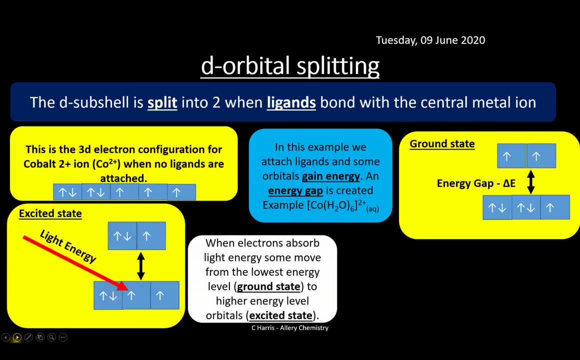 orbital, as you can see there. so we now have two one, one at the bottom. so this is the excited state. so, in order for this to happen, the energy from the light that we're, we're introducing to this complex, that might be visible light, for example, as a, as a really classic example that visible 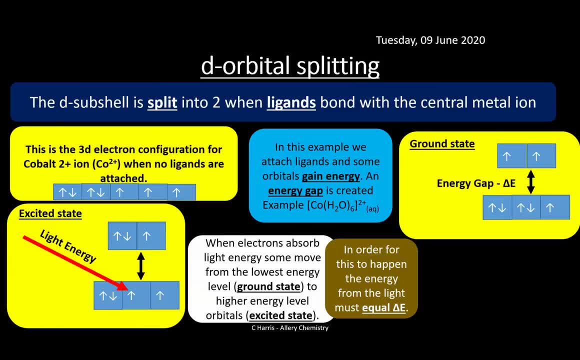 light has energy, but the the energy must the light, energy, the light must equal delta e, which is that energy gap. okay, now that gap is dependent on some certain things. so the central metal ion and its oxidation state, so depending on the metal ion in the middle, will depend on what that energy. 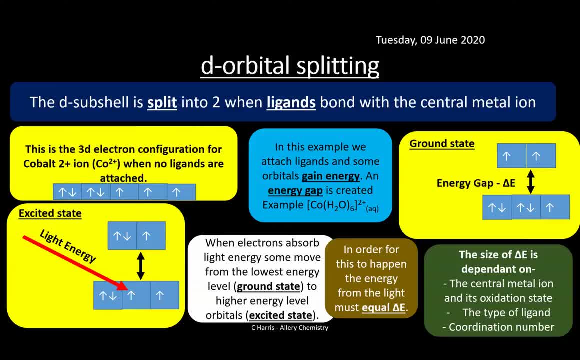 gap is going to be. that delta e and also the type of ligand can affect the size of that gap as well, and the coordination number can also affect the size of the gap. so for example, if it's got four ligands or six ligands or six coordinate bonds, 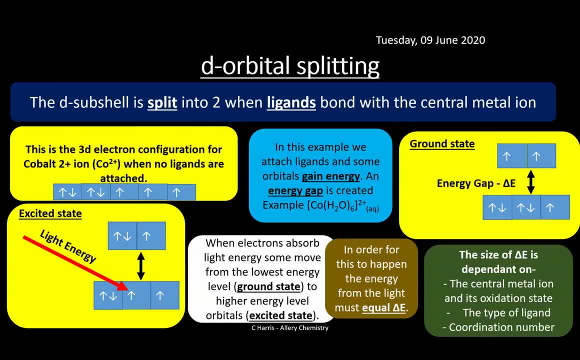 so, for example, if it's got four ligands or six coordinate bonds. so, for example, if it's got sorry, or four coordinate bonds, or um, um, or if it's only got, uh, well, you can get linear as well. you don't really need to know about linear. we can have two coordinate bonds as well. 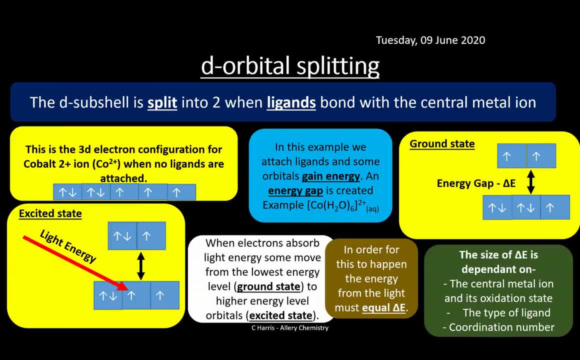 so these are the things. there's three things which affect the size of that energy gap and, as you'll see um on the next slide, the energy gap um actually gives, or this feature allows transition metals to have various different colors. so it's brilliant. i love this type of chemistry because 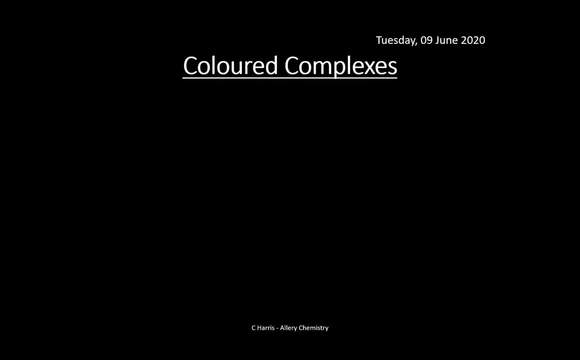 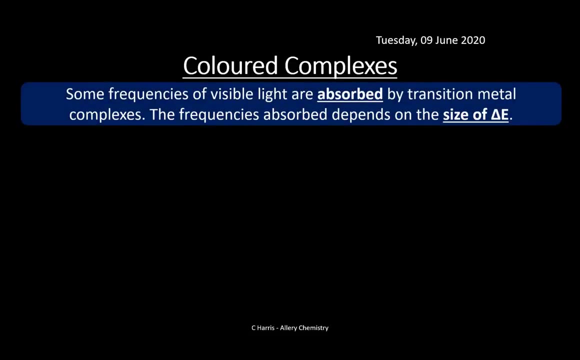 it's all nice and colorful, okay, so this leads us on, nicely, onto colored complexes. okay, so some frequencies of visible light are absorbed by the transition metal. so imagine you had a test tube with some of this solution in. okay, so we know it's a colored, it's a colored solution. if you've done this already in the lab, uh, in school or in college. 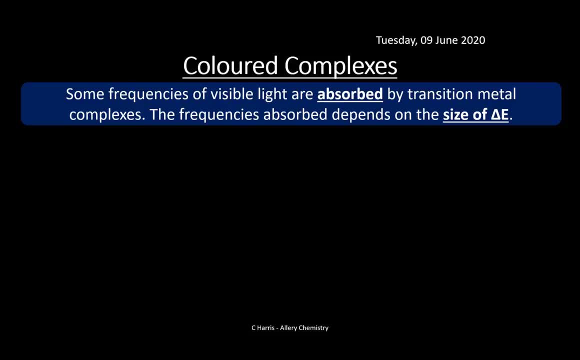 you'll know what i mean, but if you haven't, then these complexes- transition metal complexes, are colored uh in when you dissolve them in solution or if you add hydroxide to it or ammonia- and we're going to have a look at them later. but what happens is some of the frequencies of visible light are 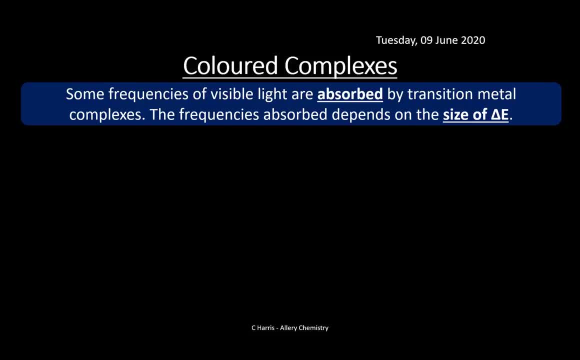 absorbed by the transition metal complexes and the frequencies absorbed depends on the size of delta e. and so remember we know what um affects delta x. we looked at that before. okay, so we know, we know there's three things that affect that. so basically, the larger the energy gap or delta e. 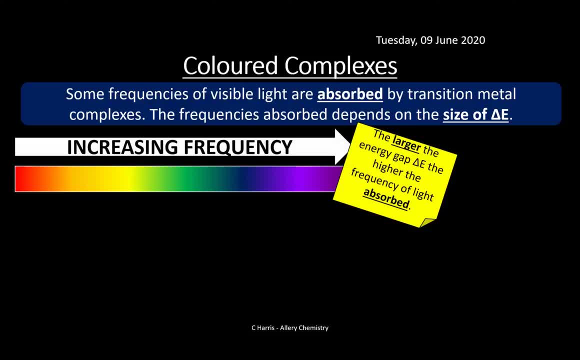 the higher the frequency of light that is absorbed. now, if you do physics, this might be quite straightforward, but basically this is the spectrum of white lights. so if we split white light, we get indigo and violet colors at the top. here these have the highest frequency and your red down at 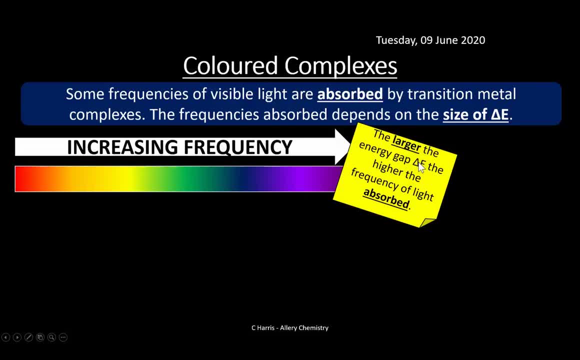 this end has the lowest frequency. so the larger that delta e, that gap that we'd seen on the previous slide, the higher the frequency of light is absorbed. so this is what's absorbed by the complex. okay, very, very important. okay. so any frequencies which are not absorbed, okay. so in 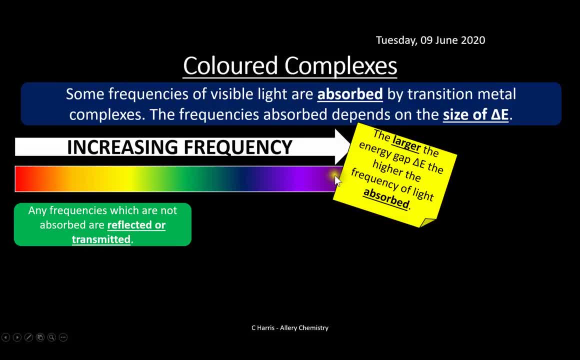 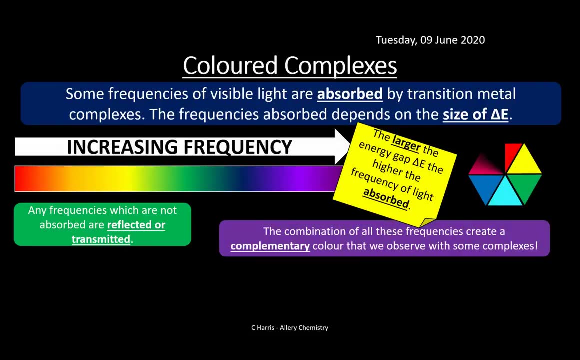 other words, if we had a very large energy gap, let's say, and we have, um, the violet was absorbed here. these will either be reflected or transmitted, so all the rest of these colors would be reflected out of the test tube. okay, so the combination of all of these frequencies that's left behind create 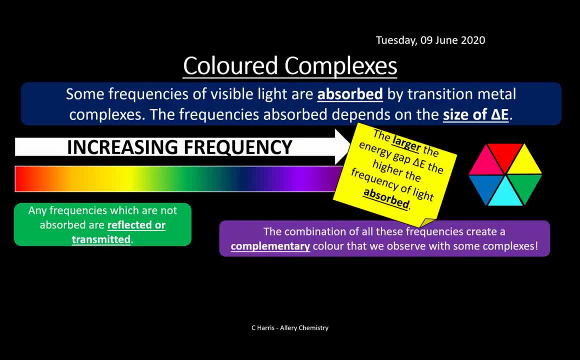 a complementary color that we observe with some of these complexes. okay, so, for example, if um, let's have a look here. so we've got copper um, copper two plus solution. so we know that this absorbs, absorbs frequencies that produce red and yellow. so we've got copper two plus solution. so we know. 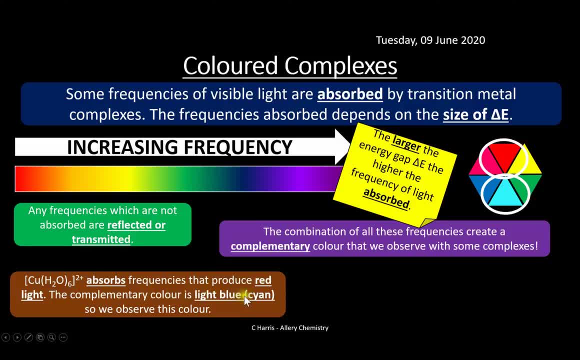 red light. okay, the complementary color is light blue or cyan. so basically, if we have copper two plus solution- you might have seen this before- um copper two plus solution or copper sulfate, for example. so you add copper sulfate to water and you form this complex here. now, that complex when. 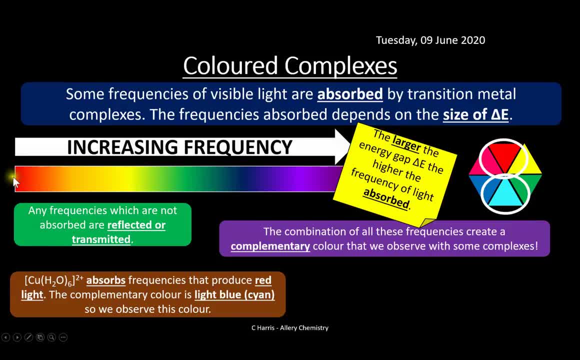 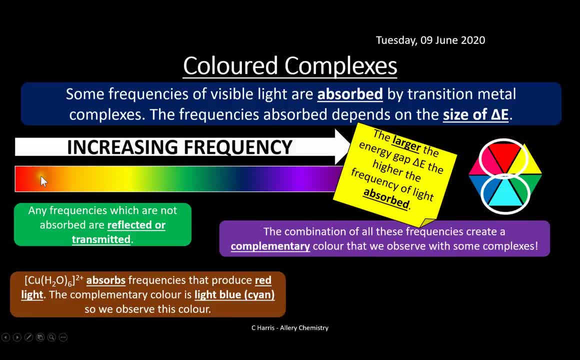 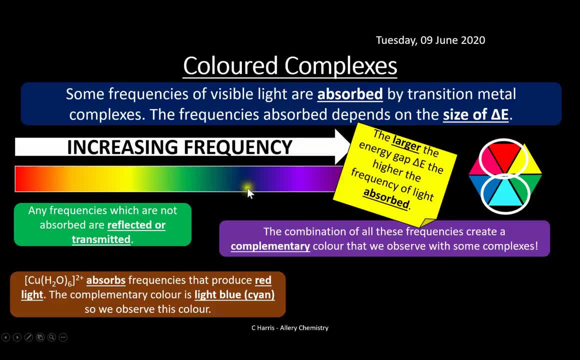 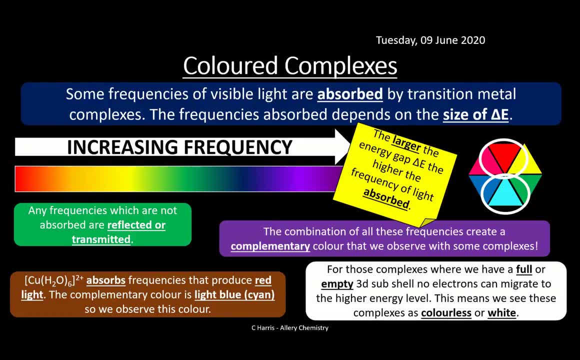 re sorte. we don't have any other red light that's taking that red line, so of course, we're going to absorb only hair, but then we are using this red line here to absorb and okay, i'll get through this very soon anyway. so sorry if this was by mistake in your case. I'm my good friends and i'm just. 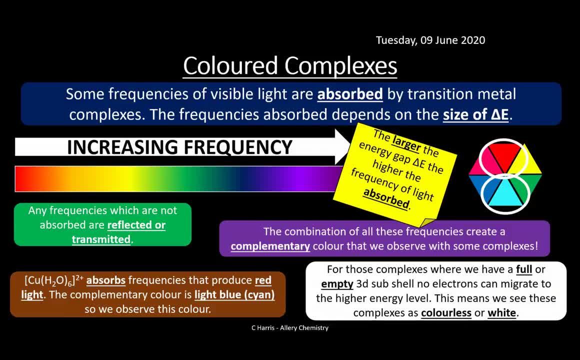 the best at explaining that. i understand why the hy предлагable, which is, let's combine all these colors 3d subshell, then no electrons can actually migrate to the higher energy level and this means we see these as colorless or white. so these are things like scandium and zinc are classic examples. so 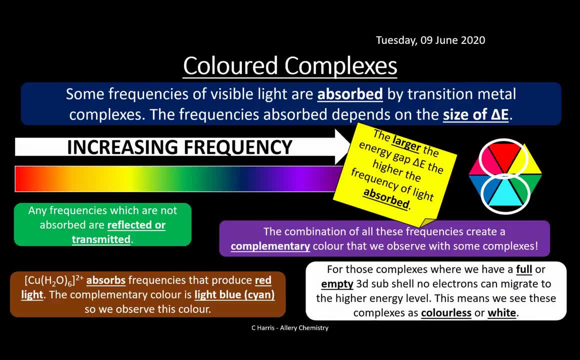 these are not transition elements. remember they have full on a full 3d subshell which is zinc or scandium has none at all. so because it's full, we can't actually move any electrons up or down. when we split them orbitals, they can't move anywhere. so because they can't move anywhere, we don't get. 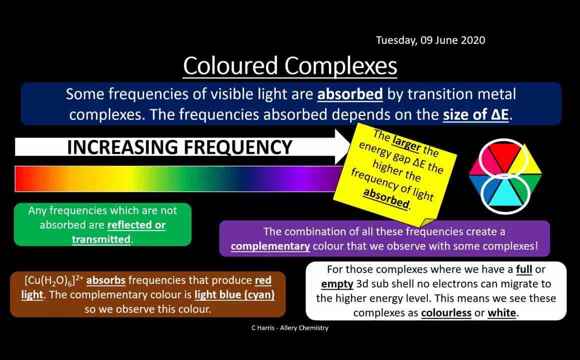 any color from them, and likewise with scandium, they don't have any electrons to move. so this is why these two do not form these colored complexes, because there's no space for them to actually move. so it kind of makes sense, doesn't it? it's all kind of coming together. i hope so anyway. 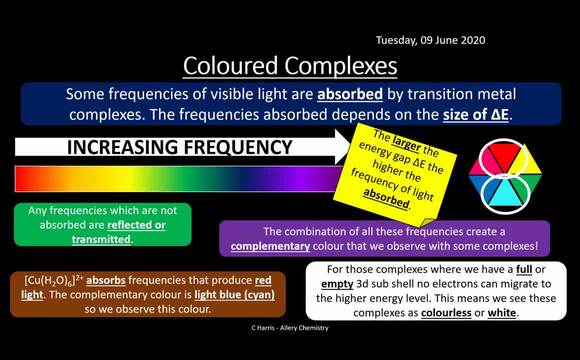 right, okay, so we know about color complexes. we're going to come on to this a little bit later on as well, towards the end of this video. when we look at um analysis, um of um of transition metals and trying to identify them, we can use the these features here. 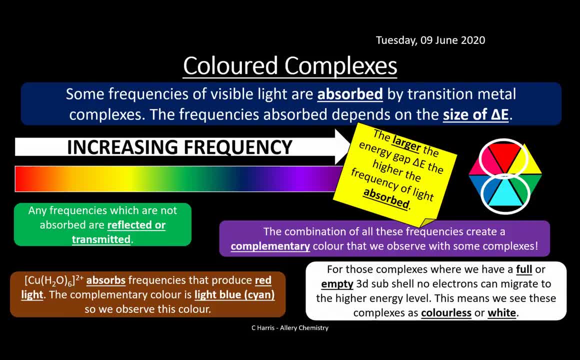 okay, so what we're going to do? so we know about um colored complexes and we know what can affect color. so it's about the um, the, the shape of the um. the shape can change the color, the um- the oxidation state of the metal line in the middle can change the color as well. 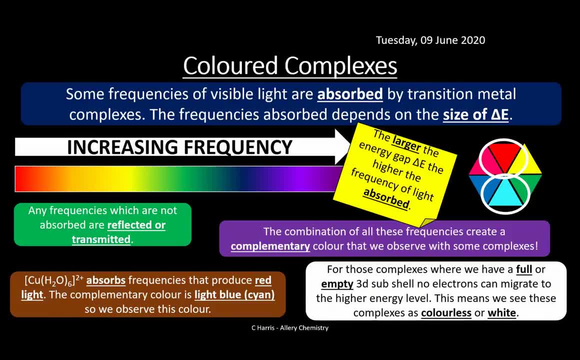 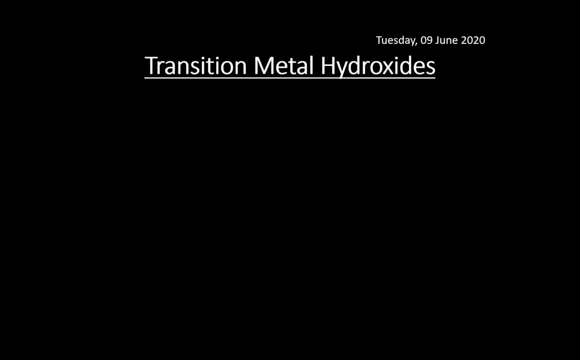 as well as um, the, the different type of metal, and also um, the type of ligand, can change the color. so what we're going to do is we're now going to um, look at a specific set of reactions here, and we're going to look at these colors and what actually. what's actually happening? 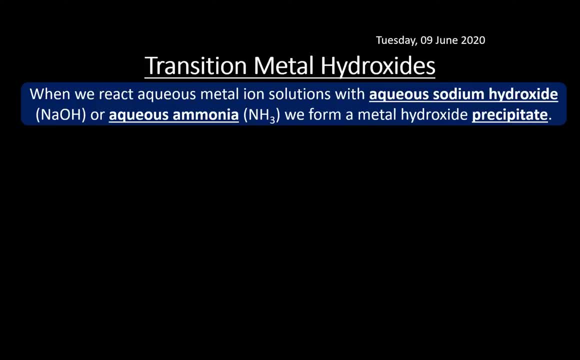 so when we react the aqueous metal ion solutions with aqueous sodium hydroxide, which is naoh, or aqueous ammonia, then we form metal hydroxide precipitates. okay, so we form these different form, these different colors. so what we're going to do is we're going to go through. these are the 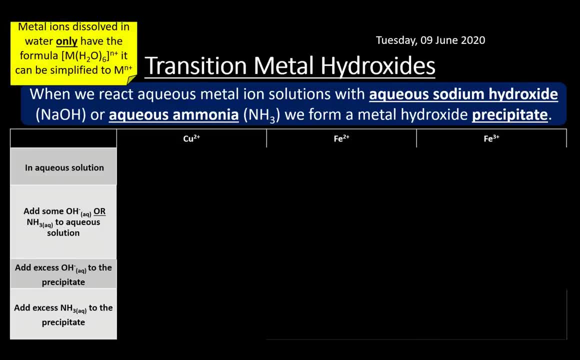 ones that you specifically need to know. so remember, in the previous slide we said you need to know copper two plus iron two plus and iron three plus. you need to know all the reactions here and the um colors associated with them as well. okay, so you've got to be vigilant, so spend a bit. 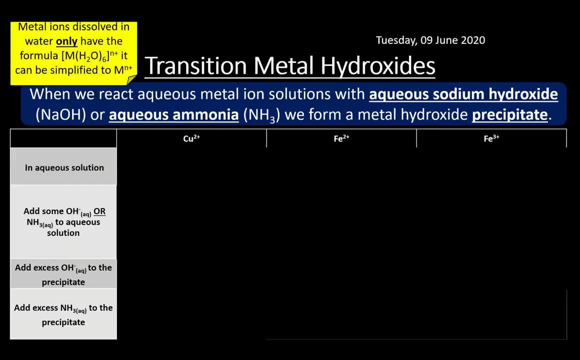 of time trying to remember all this because it's going to get you a lot of marks in the exam. okay, so just uh. before we look at the, the different uh parts here: met lines dissolved in water only have this formula remember. so it's this hexa aqua complex. so when we take our metal line and we 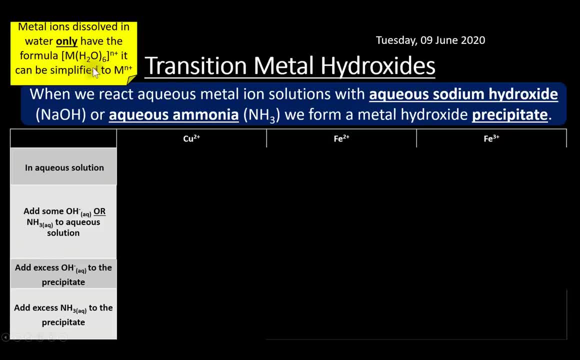 add it into water, such as copper sulfate, for example. we add that to water, it actually forms this hexa aqua complex. so what we can do is we can simplify this to mn plus. okay, that just means that that means exactly the same as six water ligands, okay. so just make sure that you're kind of familiar with these two. 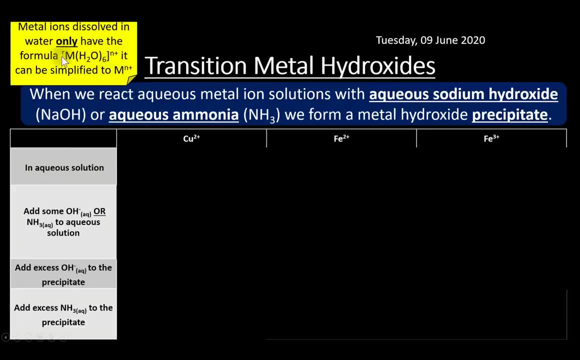 terminologies. really, when you're writing your equations, you should be writing it like this: okay, because that shows the examiner that you know exactly what, what you've actually got here, okay, okay. so let's look at the copper one first. so when we add copper, let's say copper sulfate, and we add: 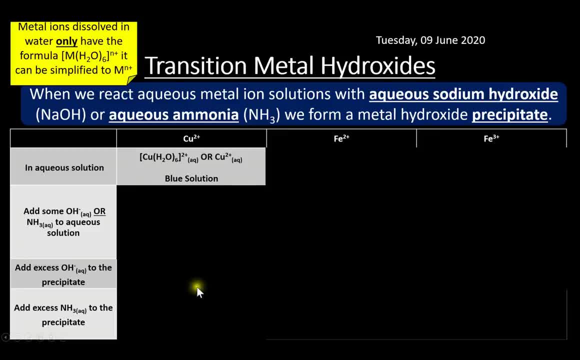 that to water. then we form our copper hexa aqua complex, as you can see there, or copper two plus aqueous, okay, and this is a blue solution. so remember, that's that kind of pale blue color that you would have seen now if we add some sodium. 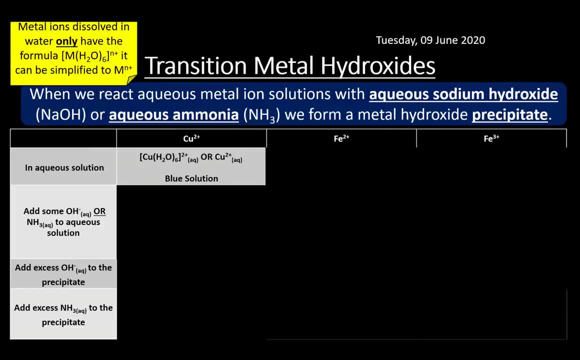 hydroxide to it or ammonia to this solution. we're actually changing the ligands here, so we get a color change. so let's have a look. so here we get a pale blue, a paler blue color. so instead of this um blue solution, we get a paler blue color, but we also get a precipitate. now what's really important? 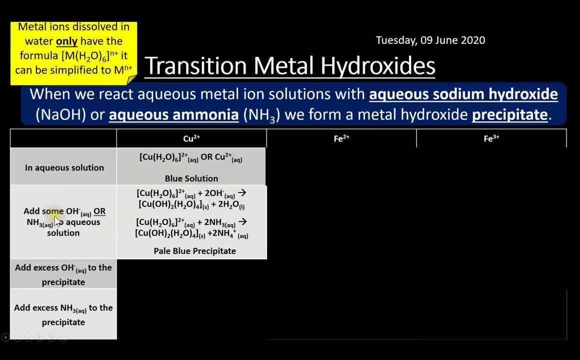 is that we're going to add a small amount, not loads, just a small amount of hydroxide, so that's going to be two oh minus and this is going to form this complex here plus water. now, the reason why we form a precipitate with either of them, um is because the complex is now neutral, so it doesn't. 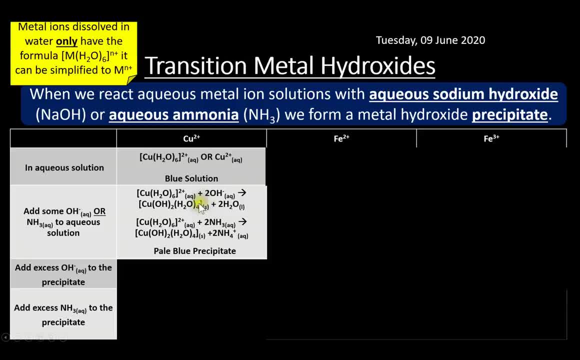 have a charge. note, there's none of these. whether it's ammonia or hydroxide has a charge. now, because it doesn't have a charge, that means it'll form a precipitate. you'll form a solid, so it precipitates. you can see there, okay, so this is a blue or pale blue precipitate. um is obviously formed here. 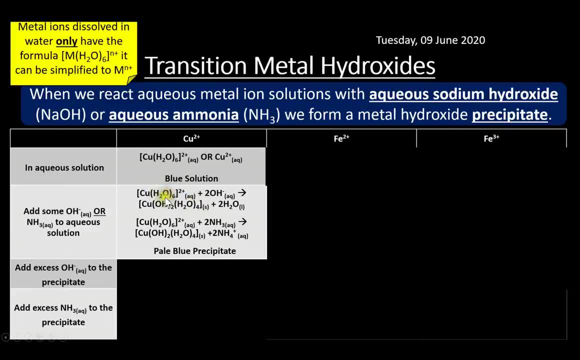 um. the reason why this is neutral is, effectively, we've got a neutral ligand here and the copper here has a two plus charge because that's what it says on there, and we're adding two negatively charged over. there's two negatively charged um. oh, minuses that have been formed within the complex. 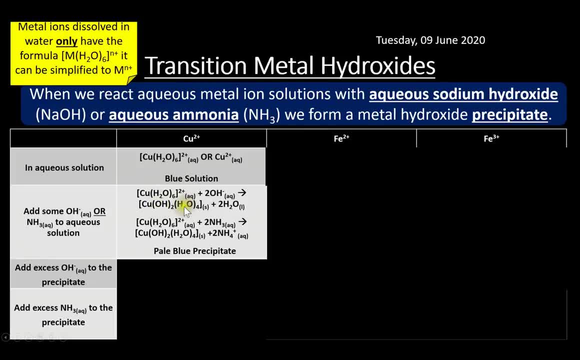 here. so these have a two negative charge, so negative each, and these are neutral. so if you've two negatives and a two plus, which is the copper, then we get a neutral complex and anything that's neutral or has no charge will precipitate out, as you can see there. okay, so that's why we need two. 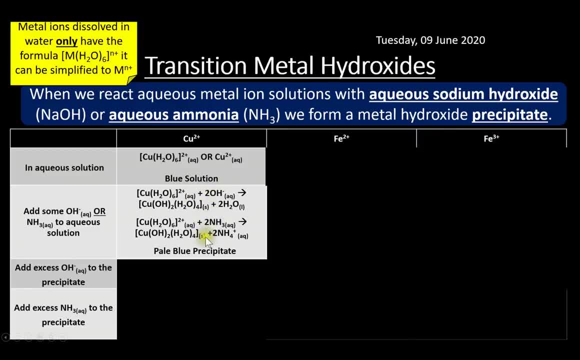 ohs, two oh minuses and two ammonias to form this neutral complex there. now, if we add excess hydroxide- so we've added that we're going to keep on adding hydroxide- then we get an insoluble um substance. so well, substance is insoluble, so it doesn't disappear, okay, so 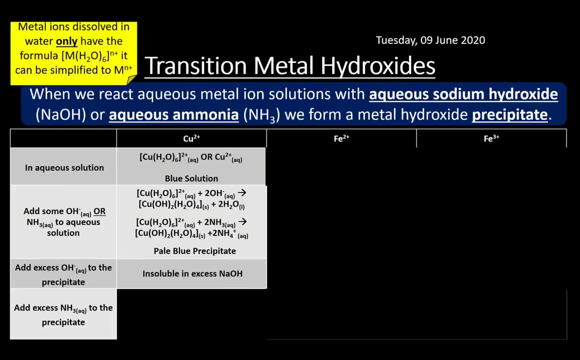 still, you still have that um precipitate. okay, so it's insoluble in excess sodium hydroxide. but if we add excess ammonia to the precipitate, then what we get with copper it's a bit of a strange one. we get a partial ligand substitution. so you can see, here there's our copper um hexa. 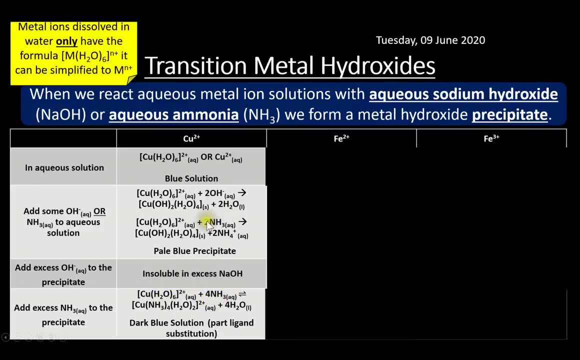 aqua complex, we're adding excess ammonia, so more than the two that we had here, and what we get is: um, we get a ligand substitution. so basically, um, four of the water ligands are substituted for four ammonias. as you can see there, two of the water ligands remain, these bonds. 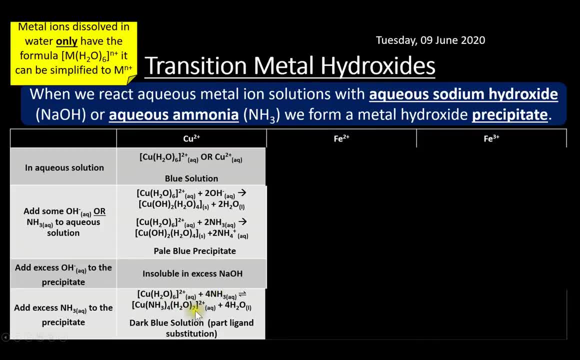 are fairly strong, so they can't be um substituted by the ammonia um. but notice that we've now got um, we've got a neutral and a neutral. so that hasn't changed because ammonia is neutral, remember as well. so this is still charged and therefore it's aqueous. okay, so still aqueous here, um, and 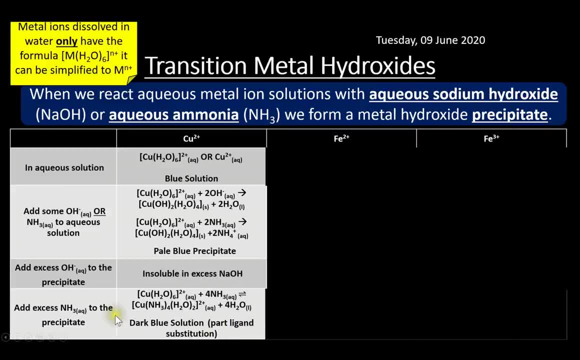 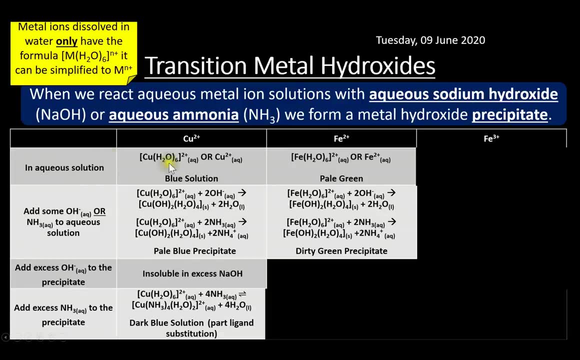 obviously the four waters have been kicked off as well, so that's a partial ligand substitution. so just be careful with that one, okay. so looking at iron two, so iron two is a pale green color. okay. same principle applies to copper. so when we add some hydroxide or h minus and some ammonia and we have the same principle, that happens, we form a. 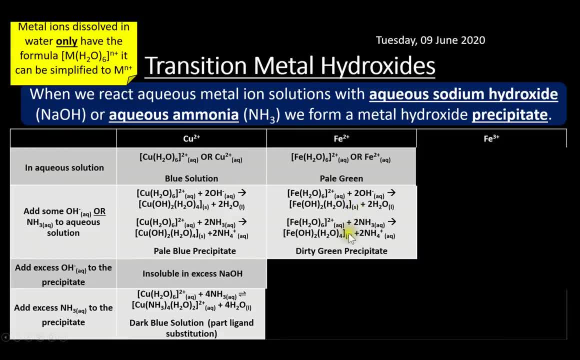 solid complex here. so this is the precipitate, because it's neutral and we form the same products as you can see on there. so there's no difference there. the color is clearly different from pale green. we get a dirty green precipitate that's formed there and then when we add excess, 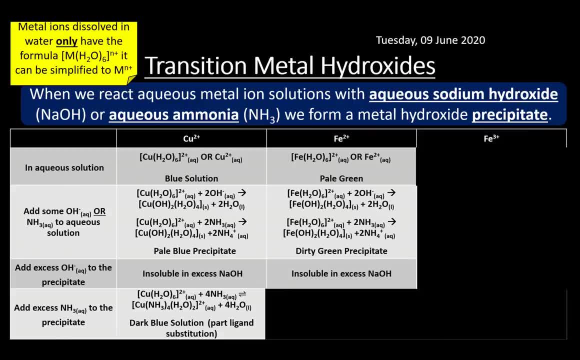 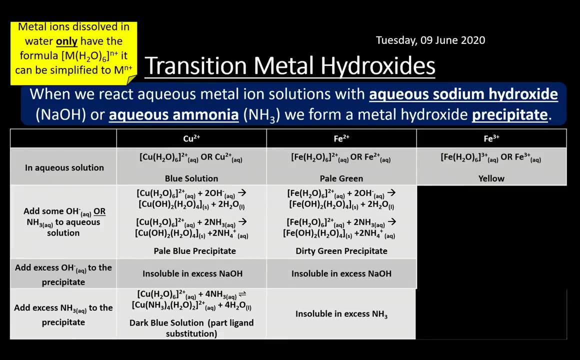 ammonia to iron two. that's also insoluble in excess ammonia. so there's no new, there's no change there. okay, so finally, fe3 plus. so this is a yellow color, as you can see there. so when we add it to an aqueous solution, now, when we add some oh minus or some ammonia, there's a subtle difference here. 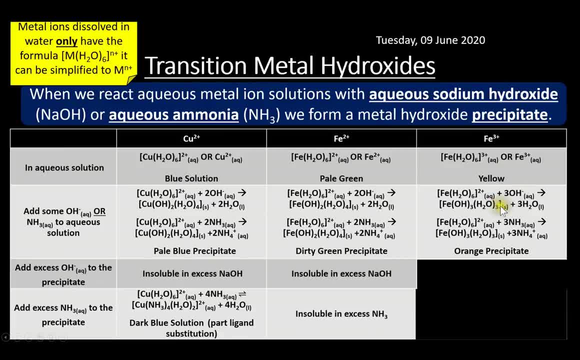 in the fact that we need three oh minuses to form this neutral complex here, because we had a three of them to form a neutral complex there. likewise with the ammonia as well. so these are neutral complexes, so they form a solid now the precipitate is orange in this case, for this one there, and 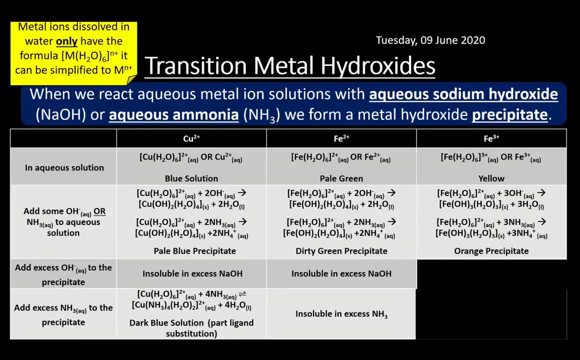 again when we add excess hydroxide and we get its insoluble. so there's no change. and it's also insoluble in excess ammonia as well. so that makes it nice and easy, doesn't it? so the only one way you get a change is the copper one, when we add excess ammonia to that. 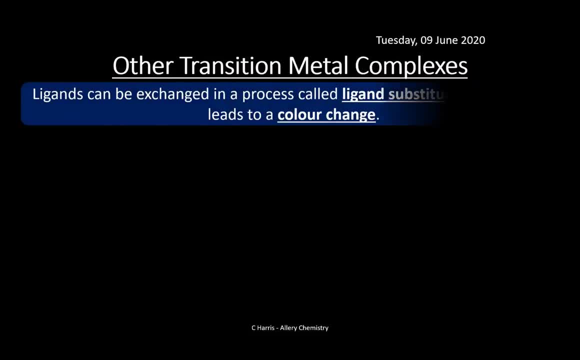 okay, so let's carry on and look at some other transition metal complexes as well, and we looked at it a little bit there in that table about ligands being exchanged, particularly when we added excess ammonia to your copper. two copper two plus aqueous solution, and now this is called 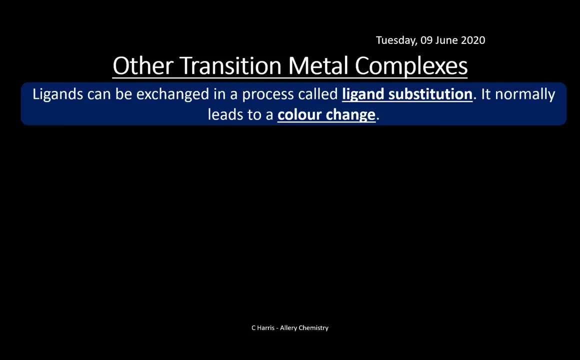 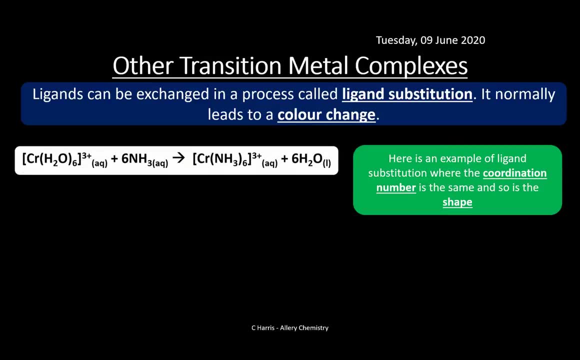 ligand substitution, as i said. so it normally leads to a color change. when we're substituting, we're changing one ligand for another, okay, so we get a substitution reaction. so here is an example of ligand substitution, where the coordination number is the same and so the shape is the same as well, but you can see here that we have chromium, in this case with. 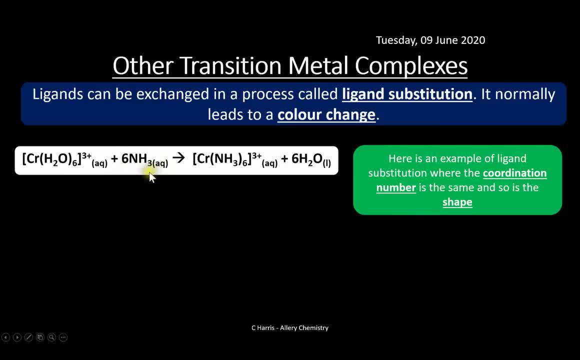 six water ligands surrounding it. we add six ammonias in this case, and we're going to get a complete ligand substitution here. so all the water ligands have been substituted for ammonia and we get our six water, six water ligands that are removed. so looking at the colors here, so it's. 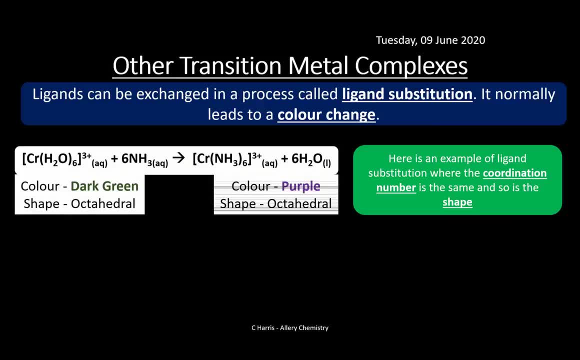 dark green on the left, but the shape is octahedral. now it's still octahedral on this side, but the colors change to purple. and this is because the shape is the same as the shape of the ammonia, because we have a different ligand attached to it and therefore the delta e, that gap between the 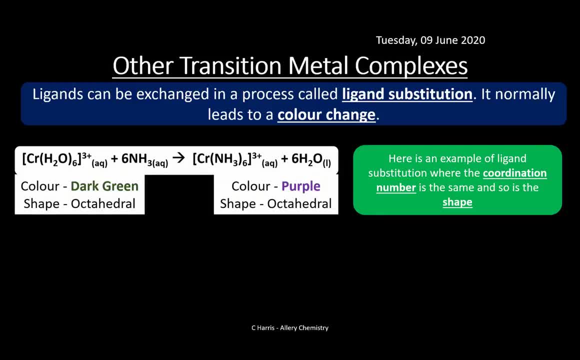 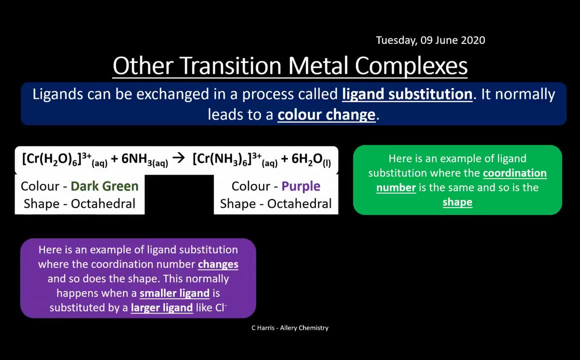 d orbitals that have been split changes, and that's why we get a different color. okay, because the ligand has an impact on that, and so here's an example of ligand substitution, where the coordination number changes and so does the shape. so this normally happens when we have a smaller ligand. 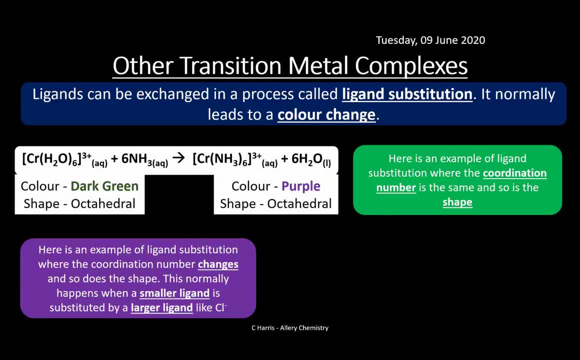 like water or ammonia or oh minus, and that's exchanged for a bigger ligand like chloride, like. so we've got copper hexa aqua here. we're going to add chloride ions that could be hydrochloric acid, for example. we'll give us this, so cl minus ions, and then we're going to form copper chloride. 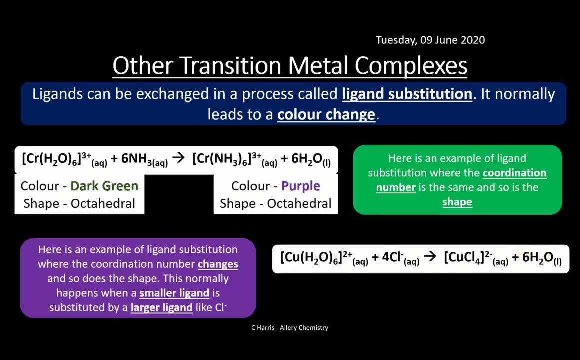 cucl4, two minus plus your six waters as well. so the color here is pale blue and it's octahedral on the left, and here we've changed the shape this time with this one, so we've now got a tetrahedral structure, and so the color changes to yellow because the shape has an impact as well, and so 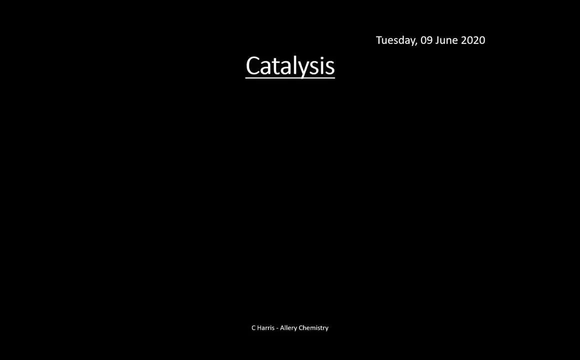 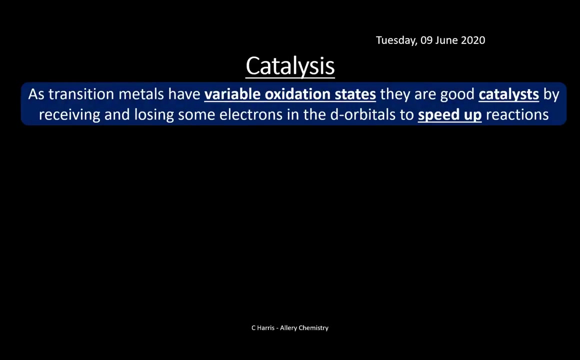 like Beef's. Please right click so you will now have the color on the color. okay, so now we're going to look at catalysts. okay, so catalysis is another feature of transition metals. transition metals are really good catalysts and we need to understand how a catalyst works. so remember from last time: 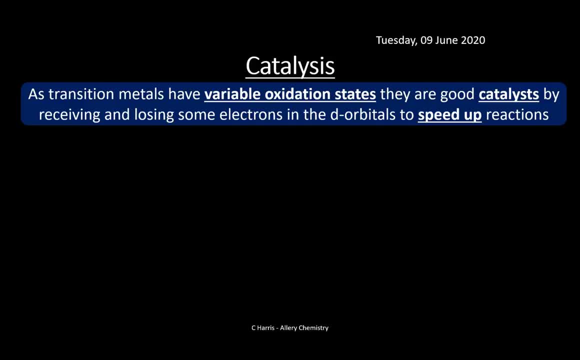 or earlier on in the video that we said that transition metals have variable oxidation states and we looked at that table with all the different oxidation states on them. that feature allows them to be good catalysts, and that's and the reason why the good catalyst is. it allows them to receive and lose electrons and that allows 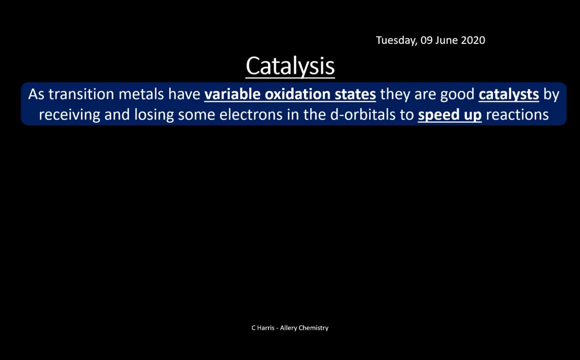 in the substance, in the substances that we're reacting and that speeds up the rate of reaction. okay, so that's what a catalyst does. so you can see, in the manufacture of sulfuric acid. so this is the, this is the contact process. so it makes sulfuric acid, which is a bulk chemical used in loads of. 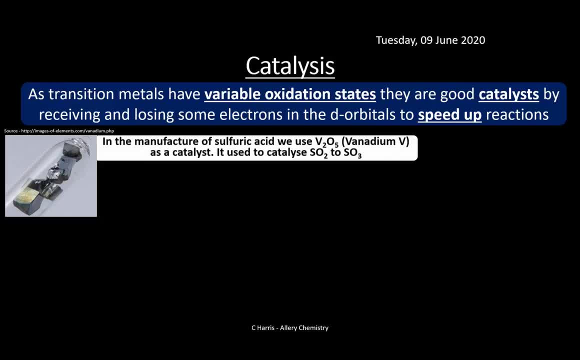 different chemical reactions. that's a vital, vital reaction, but in the manufacture that we use vanadium compound. so we use V2O5 as a catalyst and it's used to catalyze SO2 to SO3. and then what we do with that SO3 is we bubble up through water and we form sulfuric acid. so we're just looking at one. 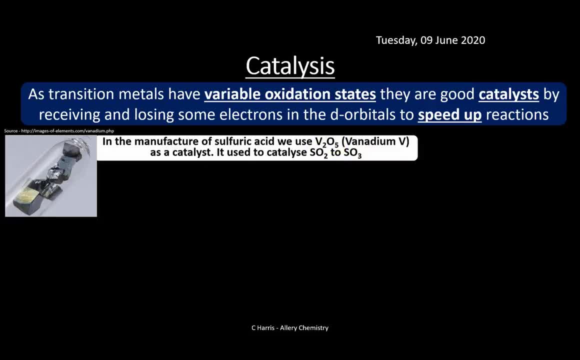 of the steps in the manufacture of sulfuric acid. so the first step is that we use the V2O5 oxidizes the sulfur dioxide to SO3, but itself V2O5 is reduced to V2O4, so the reaction is this. so it's V2O5 plus SO2- sulfur dioxide will. 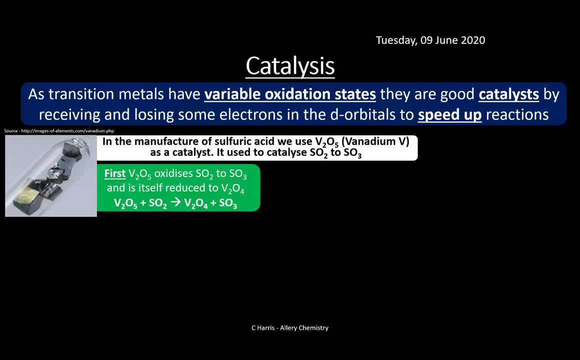 form V2O4 plus SO3. so that's the first step. and then what happens? secondly, when, because it's a catalyst, it has to be reformed, then the V2O4 is actually oxidized and it reforms V2O5. remember, catalyst is never used, it always has to be reformed. so the V2O4 reacts with oxygen. 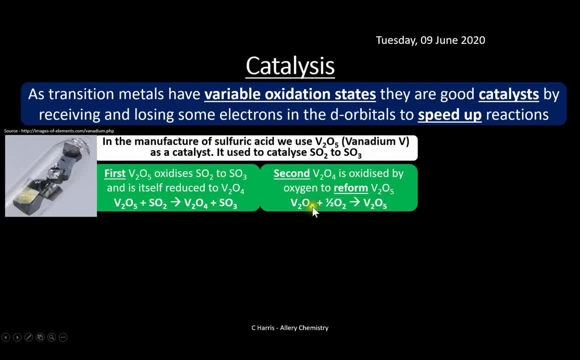 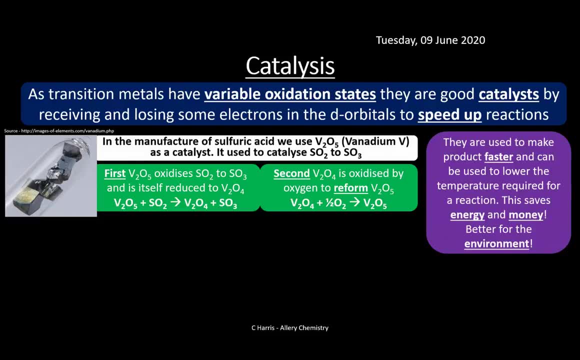 to form V2O5 and then that's then allowed to react further and continue. so very important, and they're actually used, like I say, to make the product faster. this means we can lower the temperature of the reaction and that saves energy, it saves money and it helps the environment, because 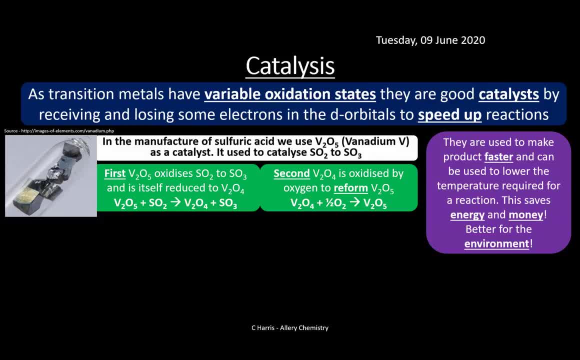 normally the heat that we need for reactions to reactions to occur is normally generated through the burning of fossil fuels. so if we don't have to use as much heat, that we're not burning as much fossil fuels, and that's got to be better for the reaction to occur. so that's the first step. 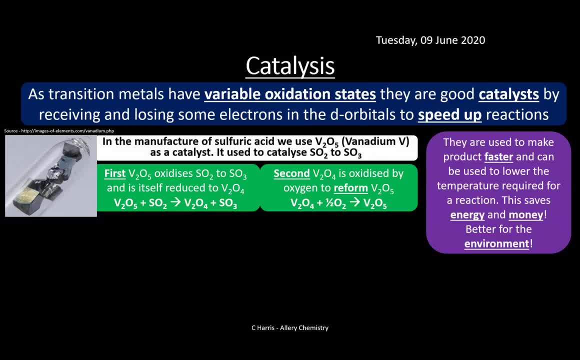 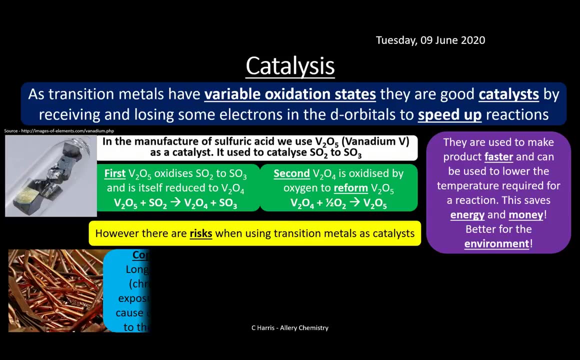 to the environment as a result. okay, but we've got to be careful. catalyst catalysts are good at speeding up reactions, but there are hazards associated with transition metal transition metals using being used as catalysts. so examples for some of them here are copper, and copper actually forms or has chronic exposure, can cause damage to the liver. you can get liver damage by. 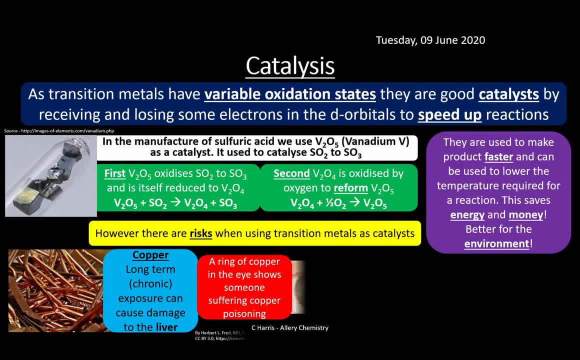 exposure to copper long term and so the copper catalysts and you can get a ring of copper in the eye shows that someone's suffering from copper poisoning. so you can see in the picture here you've got this just around the eye. I hope you can. hope you can see it quite. 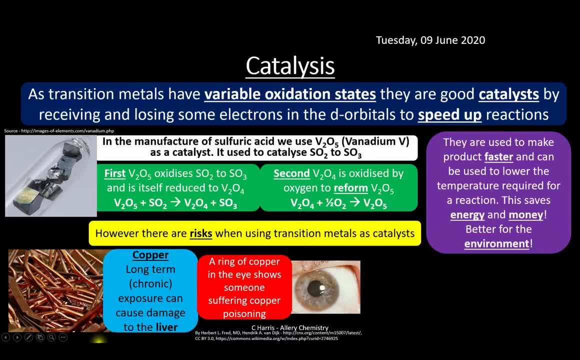 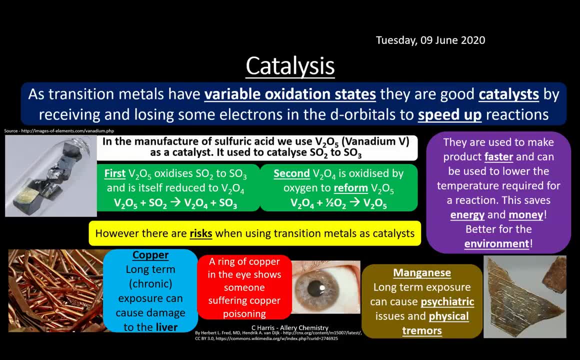 relatively easy. it's quite subtle, but you'd see we've got this copper ring around the eye there. another example of a catalyst is manganese. now, long-term exposure to manganese catalysts can cause psychiatric issues and you can get tremors as well, so not exactly the type of stuff. 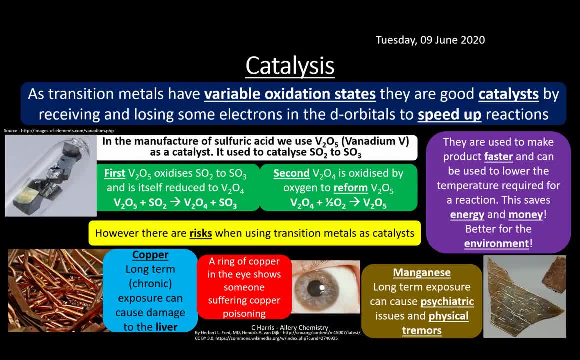 you want to be exposed to a long period of time, so you have to have a long-term exposure to manganese catalysts and you can get tremors as well. so not exactly the type of stuff you want to be exposed to suitable PPE when you're handling and some of these transition metal and catalysts, okay. so 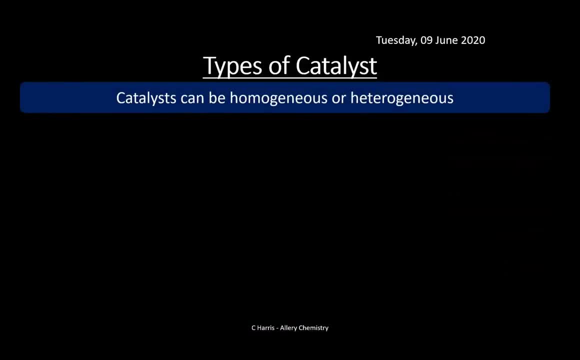 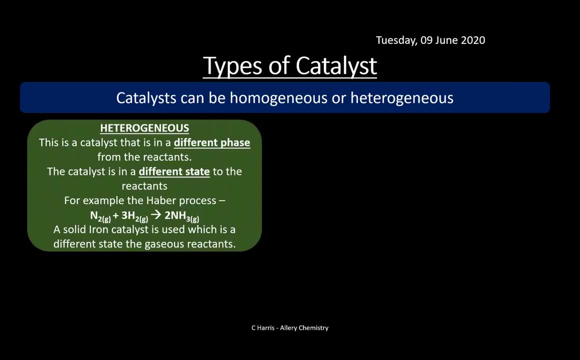 let's look at some of the types of catalysts that are available to us. so catalysts can be homogeneous or they can be heterogeneous. so let's look at heterogeneous first. so hetero means different. okay, so this is a catalyst that's in a different phase from the reactants. okay, so the 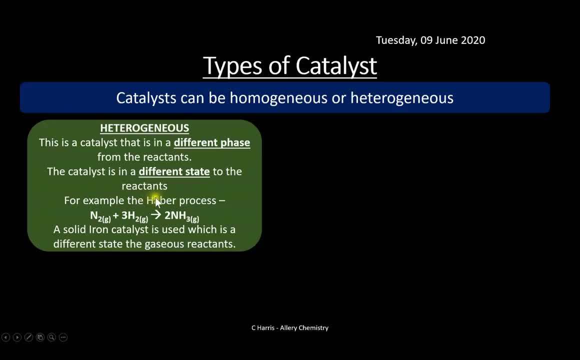 catalysts in a different state to the reactants. so our classic example: we in the hair before process. so this is the manufacture of ammonia, which is used in agriculture as a fertilizer. so a very important process. but the catalyst we use here is an iron catalyst. now, ions are solid, but 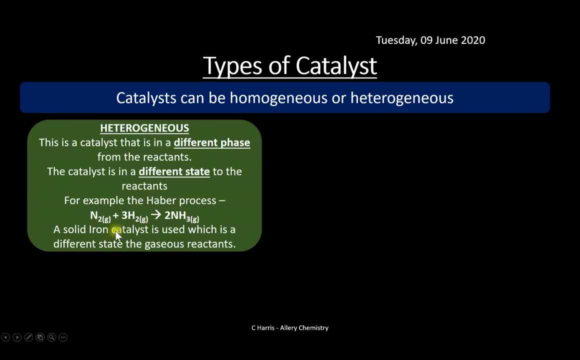 our reactants and products are gases, so you can see here that it is in a different state to the actual reactants and products here which are which are in gas phase. so, and to try and improve the performance of the catalyst, then if we increase the surface area of the catalyst of heterogeneous 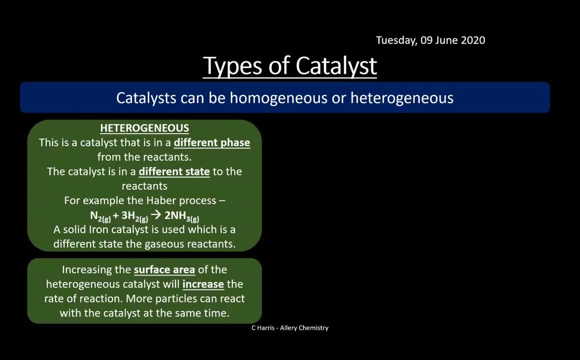 catalyst, this will actually increase the rate of reaction. so, for example, we take that iron and we grind it into a fine powder, we increase the surface area and this means that more particles can actually react with the catalyst. at the same time, if we've got a larger surface area, so that improves. 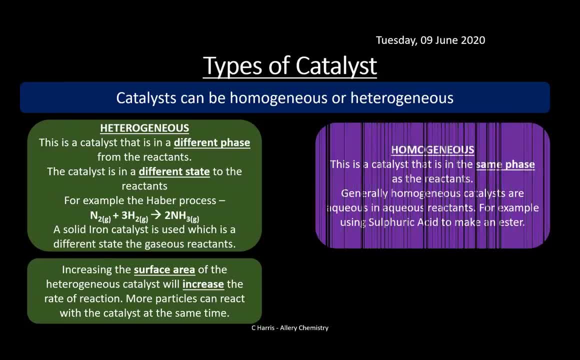 the performance of heterogeneous catalysts. there are homogeneous catalysts as well, so this means they're in the same phase as the reactants. so homogeneous catalysts are normally in aqueous solution, so it's normally with aqueous reactions and an aqueous catalyst. so, for example, we're using sulfuric acid to make an. ester is a classic. 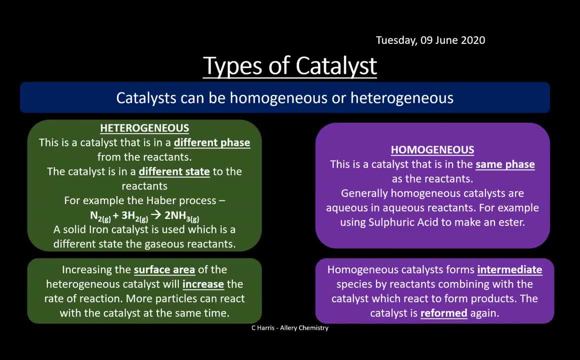 example of this. now, homogeneous catalysts actually have a slightly different energy profile. they actually form an intermediate species by reactants combining with the catalyst, which then react to form the products, and then the catalyst is then reformed back again. so the homogeneous catalysts actually integrate quite, you know, quite integral within the reaction, whereas a heterogeneous 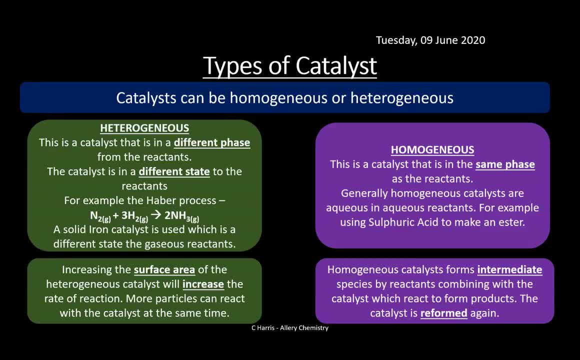 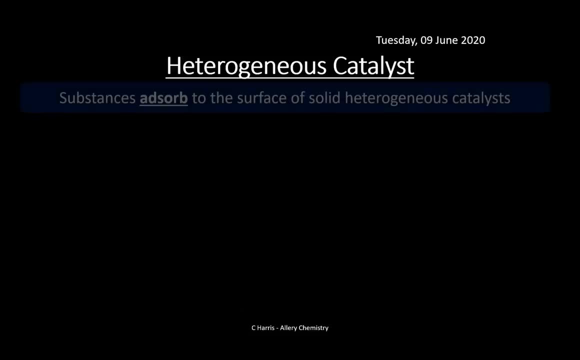 catalyst just kind of sits on a on a plate and the product passes through the powder, let's say, whereas a homogeneous catalyst is actually integral within the, within the reaction. excuse me, right, I'm starting to lose my voice. I think, right. so let's look at a little bit more detail at heterogeneous catalysts, so substances. 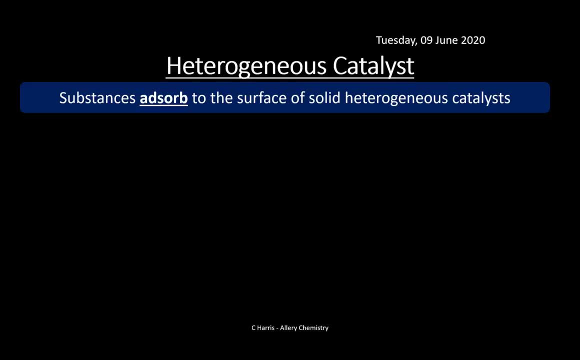 heterogeneous catalysts work by substances adsorbing. that's not a mistake either. that's definitely a D adsorbing to the surface of the catalyst. so reactions occur on solid heterogeneous catalysts. so they actually occur on the surface of these and, like I say, the 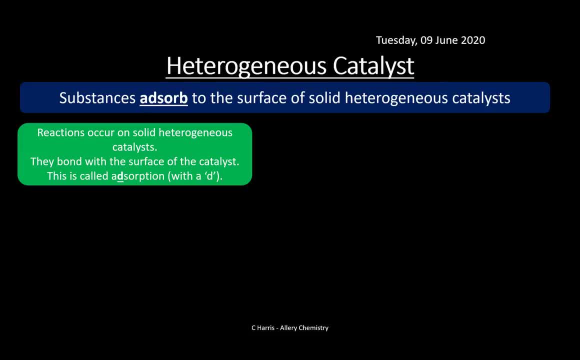 substances bond or adsorbed the surface of the catalyst and that allows reactions to happen. so the reaction actually happens on the surface of these catalysts. so bonds and the reactants weaken is an unpaired electron. so for example, CL radicals are chlorine atom and these radicals react with an unpaired electron. 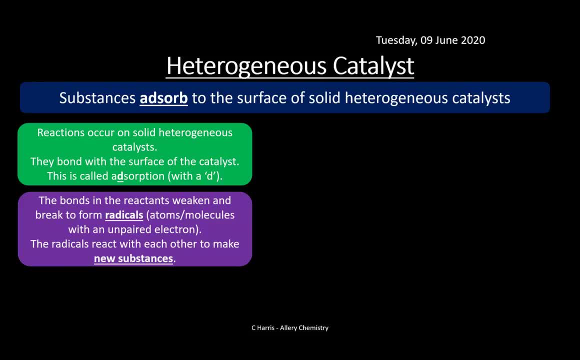 cl radicals are chlorine atom and these radicals react within a carbless each other to make new substances. okay, so this is basically how heterogeneous catalyst works, and so these new molecules are then released from the surface of the catalyst and we call that desorption. so the reaction happens on the catalyst surface. okay, so let's bring back that other. 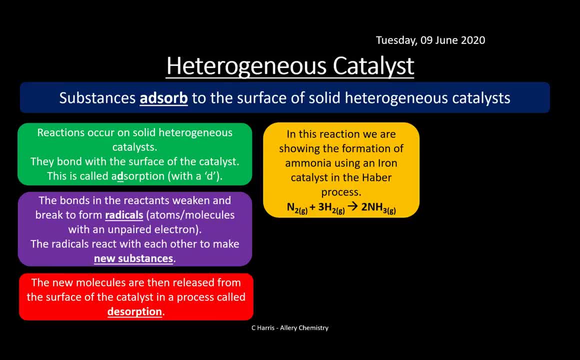 example that we mentioned before. so this is um the manufacture of ammonia, so in the herba process. so we're using an iron catalyst in this reaction. so here's our iron catalyst surface here and we've got adsorption of the substances. so here they are. so there's your adsorption, so you can see. 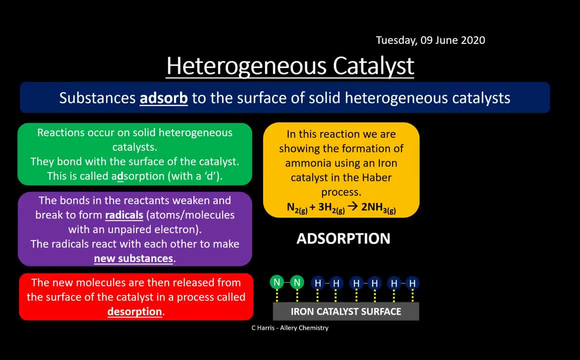 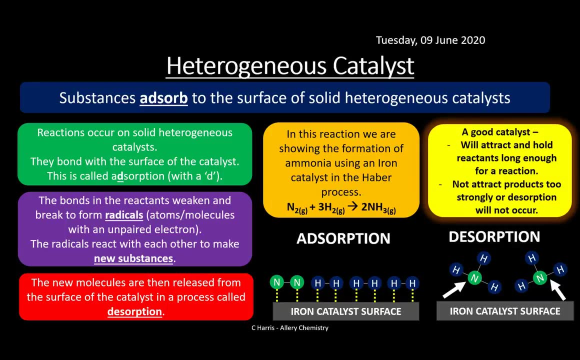 there you go. we've got our hydrogen molecules and our nitrogen molecules. so this is adsorption. so they stick to the iron catalyst that allows the reaction to happen. once the reaction has occurred, we then get desorption. they break away, as you can see there. okay, and that's basically how the 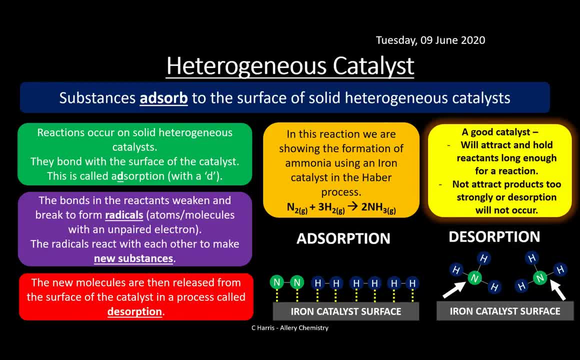 reaction works okay. so you've got adsorption- desorption- so make sure you're aware of that. so good catalyst will and hold the reactants long enough for a reaction. if they don't, then the catalyst isn't very good, and a good catalyst as well will not attract products too. 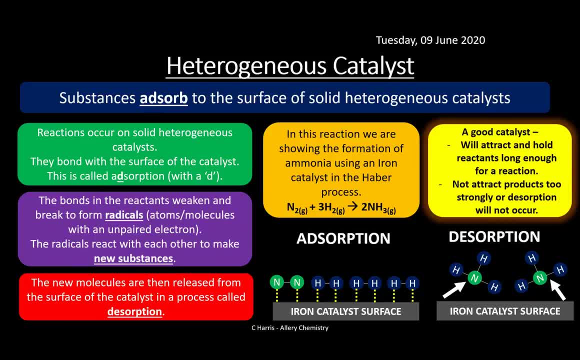 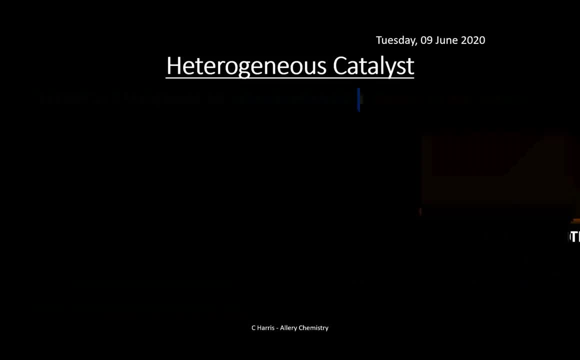 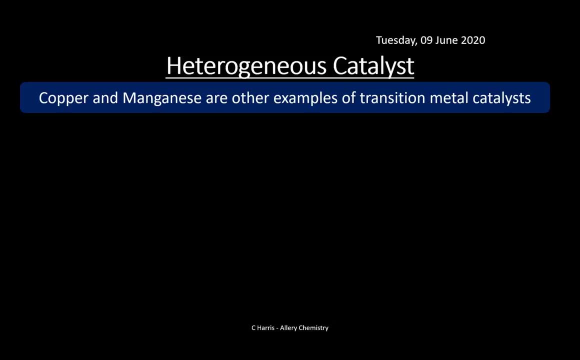 strongly, otherwise desorption won't occur either. so you need enough of an attraction, just enough for that reaction to happen. so it's a very fine balance, as you can see. okay, so copper and manganese are other examples of transition, of transition metal catalysts, as we've- as we've seen earlier and we've got to be. 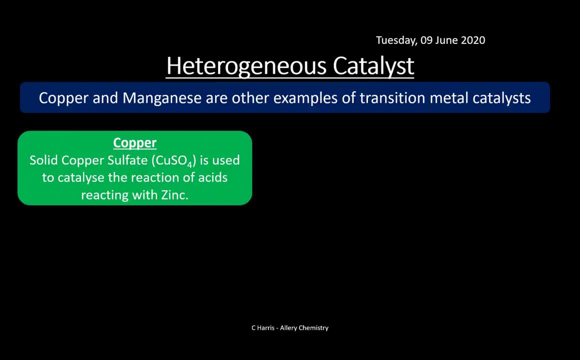 careful with these types of catalysts. and but copper, so solid copper sulfate is used to catalyze reactions of acids reacting with zinc, for examples. we use copper sulfate as our reaction there, so you need to know this particular example. these are specific examples that the exam board want you to know. okay, so zinc. 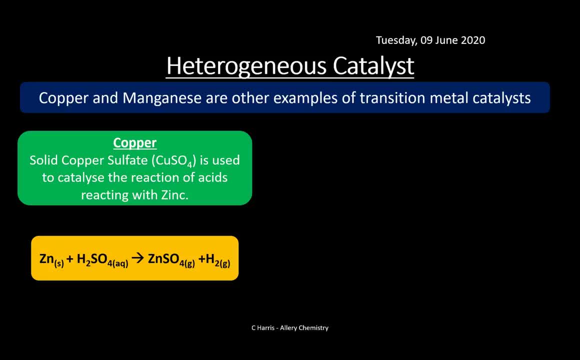 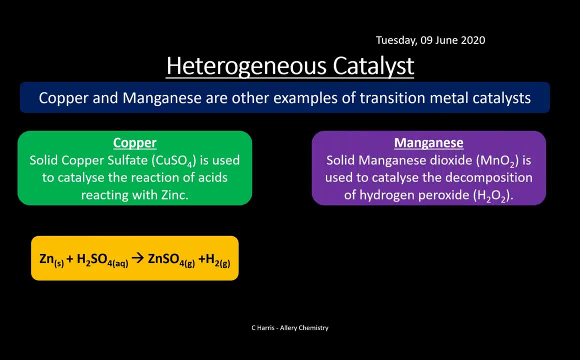 reacts with sulfuric acid to form zinc sulfate and hydrogen of. should we use the catalyst, solid copper sulfate, to catalyze that reaction, and manganese? solid manganese is a catalyst for the reaction of sulfuric acid, and manganese- manganese dioxide or MnO2, is used to catalyse the decomposition of hydrogen peroxide. So we 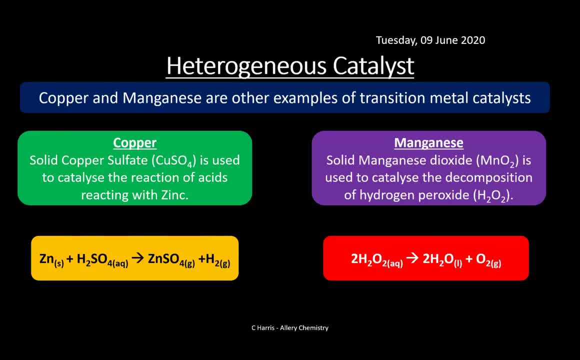 need to know that hydrogen peroxide breaks down into water and oxygen. Okay, so you need to know them. specific examples there. and obviously you need to know the risks as well associated with handling copper, as we said before, and handling manganese as a catalyst. Okay, so let's look at. 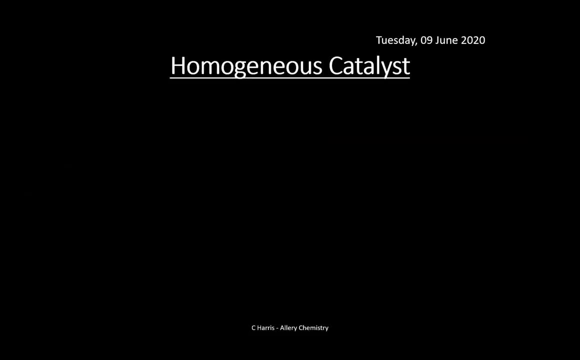 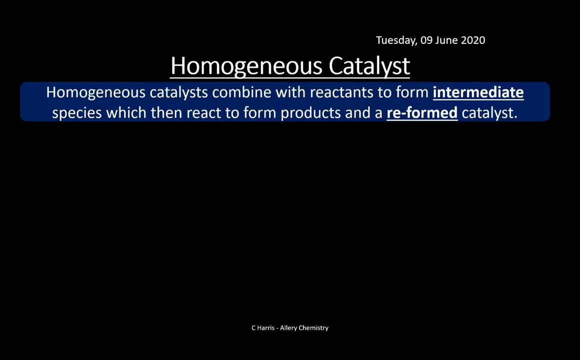 homogeneous catalysts because, remember, we've got these types of catalysts as well as heterogeneous. So homogeneous catalysts, these combine with the reactants to form an intermediate, So it's not like heterogeneous, where you have a surface and the substances adsorb to the surface and desorb. 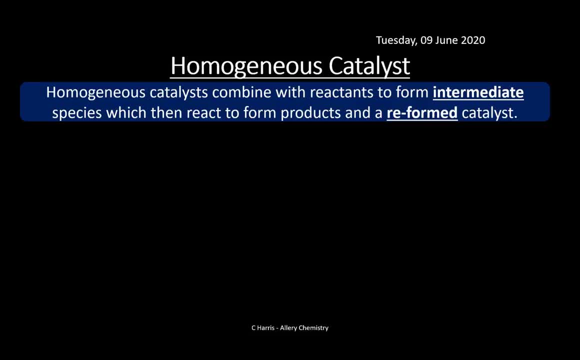 These actually form an integral part of the actual solution that we're reacting. They form an intermediate, but, just like with any catalyst, it must remain unchanged at the end of the reaction. So in this case they're reformed. Okay, so 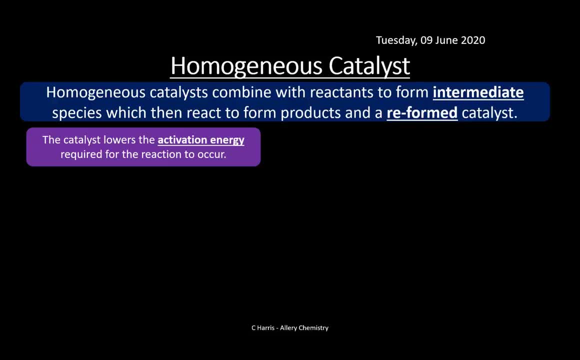 a catalyst, always. this is any catalyst, whether it's homogeneous or heterogeneous. it lowers the activation energy, So this means less energy is required to allow the reaction to happen. So this is the main part of a catalyst. So remember, the catalyst is always reformed. It's never actually. 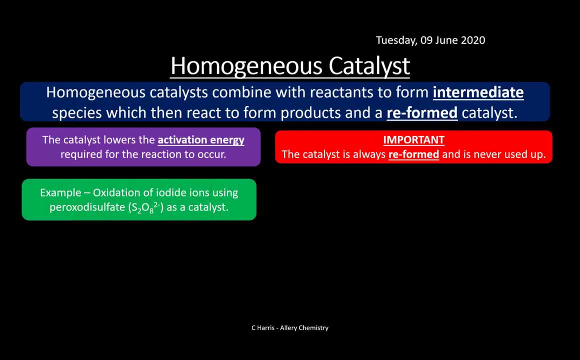 used up. It's really important. So let's look at this particular example here. Now you need to know this example, specific one as a homogeneous catalyst. So oxidation of iodide ions using peroxyl disulfate- Which is S2O8 2- as a catalyst. Okay, so this is a homogeneous catalyst. It's a little bit more complicated, but 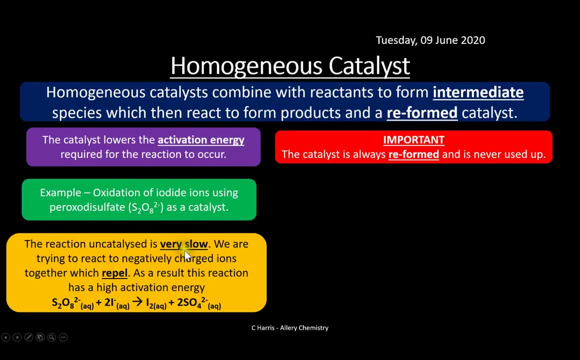 there's a, there's a rationale behind this. So the reaction, uncatalyzed, is really slow. So we can see here what we're trying to do is react this, which is a 2-, with this, which is a minus. These two negatives are never. 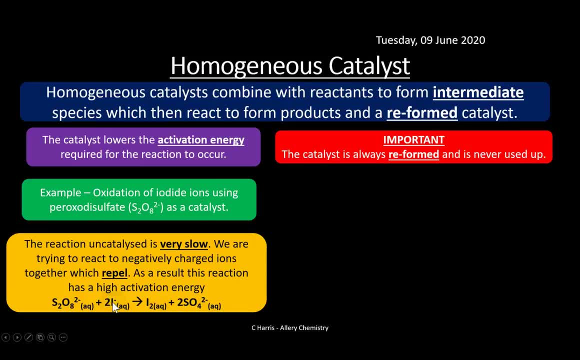 going to react with each other. I mean, they're just unless you give them really severe conditions, these are just going to repel each other. So we need something that allows these two react, But we need something to kind of act as a mediator, I suppose, between the two, or a catalyst. Okay, so these two here are never going to react, So we need a catalyst to react here. So it happens in two steps. 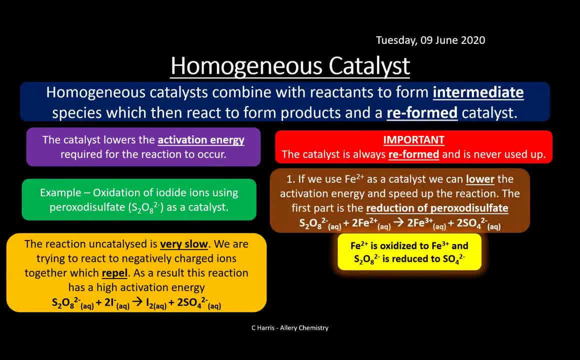 So step one: we use the Fe2 plus as a catalyst in this example. here, Okay, Fe2 plus is a solution, So it's all in the same phase. It's a homogeneous catalyst And this lowers the activation energy, speeds up the reaction. So the first step here is the peroxyl disulfate. 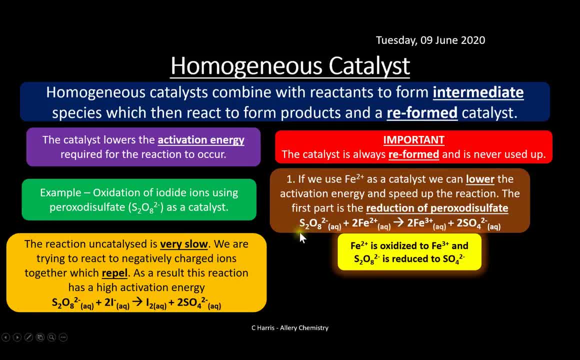 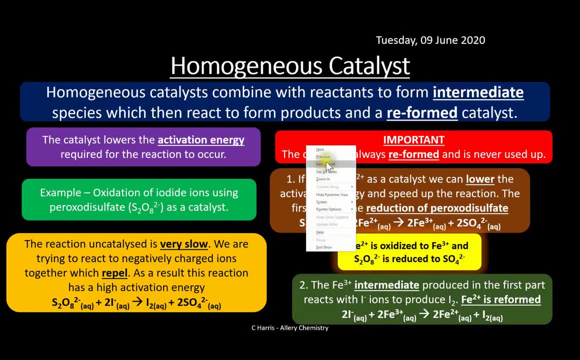 So this lowers the activation energy, speeds up the reaction. So the first step here is the peroxyl disulfate. So the first step here is the peroxyl disulfate. And S2O8 2 minus reacts with upgrade. 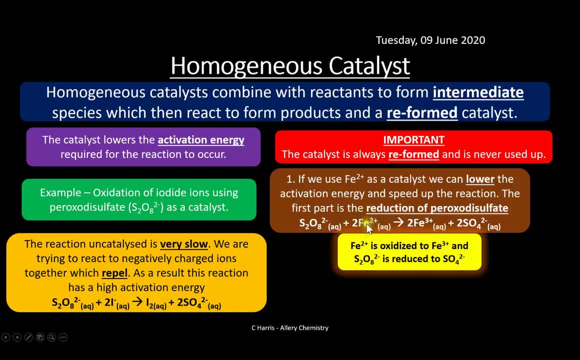 So you can see here we've got S2O8 2 minus reacting with two Fe2, as you can see there. So these will react because that's a negative and a positive. So that's fine, and what happens is that the ion is oxidised to Fe3 plus and the S2O8 2 minus is. 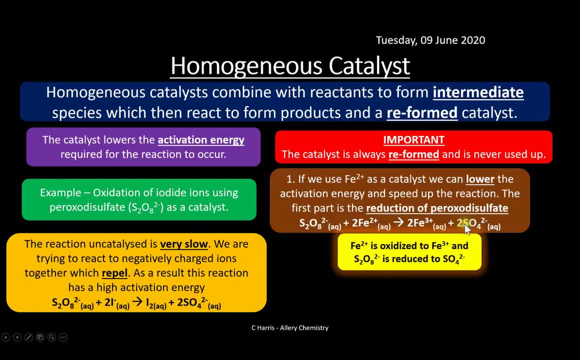 reduced to So2 minus. Okay. So we've got two lots of that. So there's one of our products. look there, Okay. so then what we need to do is this: fe3 plus that we formed always we have to. we must have fe2 plus. 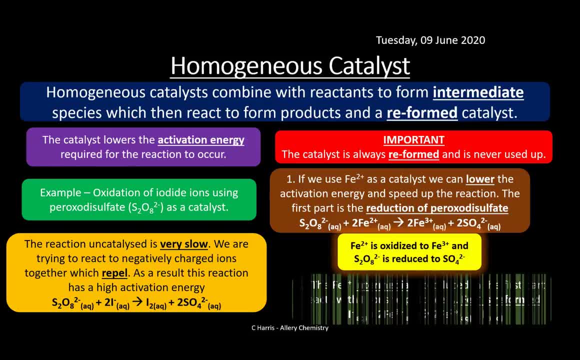 as a product. okay, because it's a catalyst, so it must be reformed. so the second step is that fe3 plus intermediate produced in that first step reacts with the i minus ions- that's the other reactant that we need here- and that forms iodine i2 and obviously we reform our catalyst back. 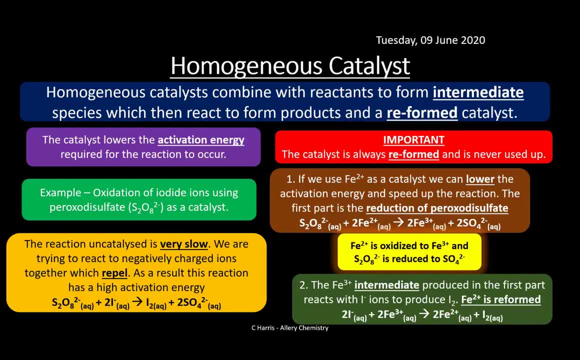 again. so that's fe2 plus, as you can see on there. so you can see, this is a homogeneous setup. you form an intermediate and it's crucial that the catalyst is reformed as a product in that second step there, okay, right, okay. so we're now going to move on to the last section of this video, which 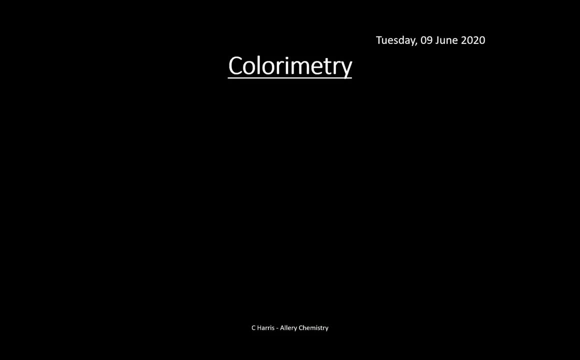 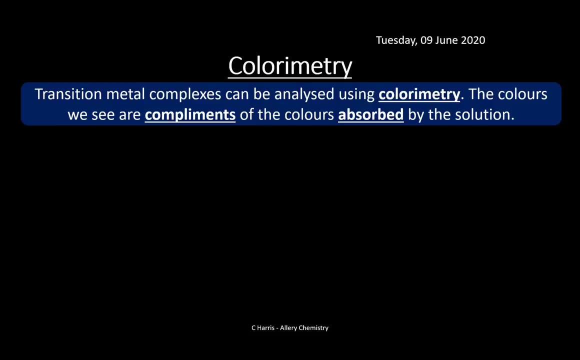 is looking at colorimetry, and colorimetry is a really useful technique of trying to identify our transition metals. okay, and obviously we're using colorimetry. the reason why we're using color is because we know that one of the main features of transition metals is they form colored complexes. okay, and we've looked at that with the d-orbital splittin. 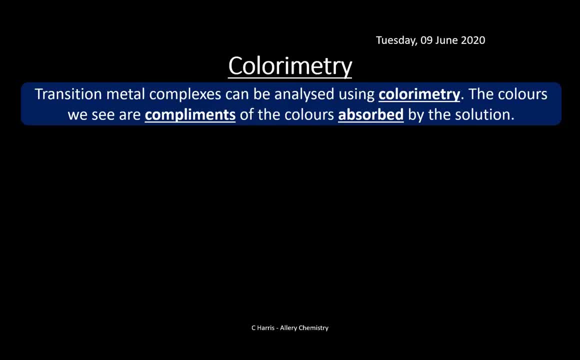 so, remember, the colors that we observe are complements of the ones of the of the colors that are absorbed by the actual, by the actual transition metal. so, remember, your white light is made up of all these colors here, okay, and so when that white light hits a transition metal, 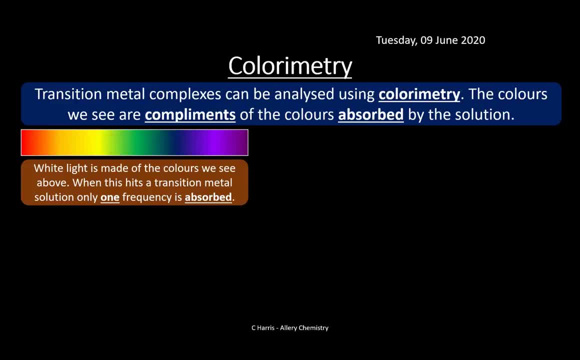 only one of the colors that are absorbed by the transition metal is the white light frequency. one of these in the spectrum is actually absorbed. so if you remember that from what we said before, so any frequency which are not these are reflected or transmitted. so if you remember that, okay, so that means 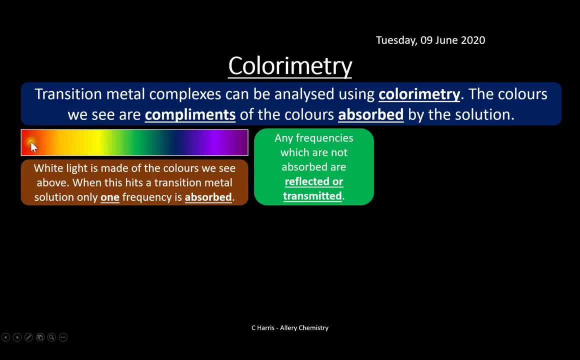 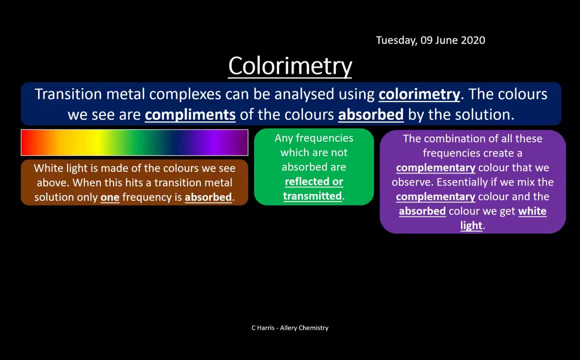 anything that is not here. so, for example, if red is absorbed here, then all the other colors here blend together to reflect or transmit from the test tube. so the combination of all of these, they create complementary color that we observe and remember that from what we mentioned before and if we mix the 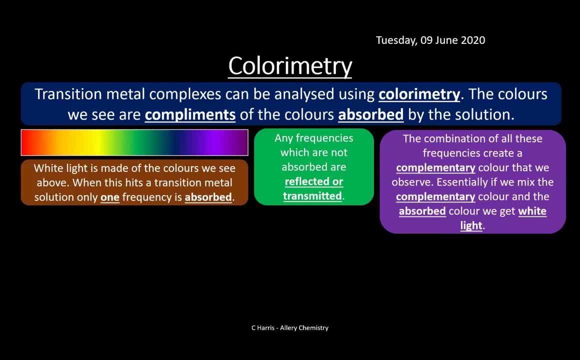 complementary color and the absorbed color, we get white light. in other words, if we mix all these together, and the absorbed and the complementary ones, then we get white light that combines. so if we bring back our wheel again, so remember, and the color wheel allows us to predict the color of light. this 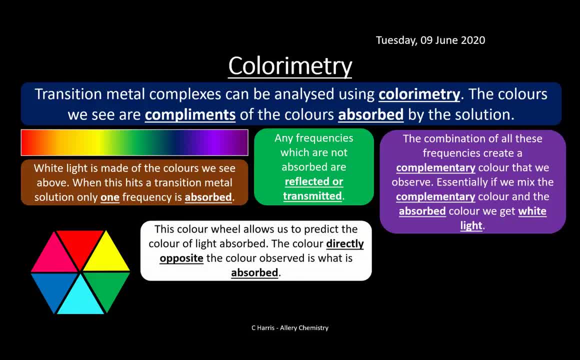 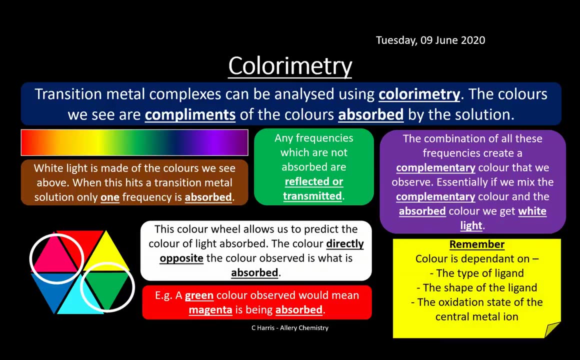 absorbs, and the one that's directly opposite is is the one that's actually being absorbed. so, for example, a green color. if we see green color, it means that magenta is being absorbed by the transition metal complex. so remember what actually changes, or the color that is dependent on, is the type. 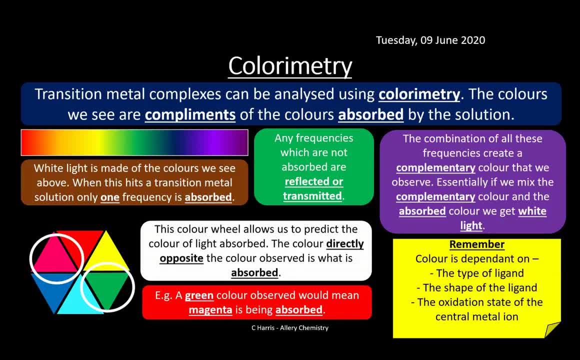 of ligand, the shape of the ligand and so the shape of the complex, should I say not the shape of the ligand, it's the type of ligand, the shape of the complex and also the oxidation state of the central metal line. so these things, 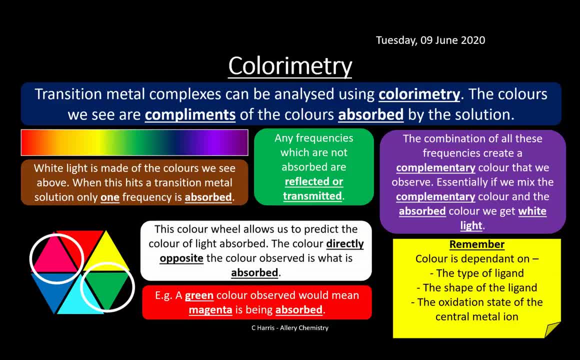 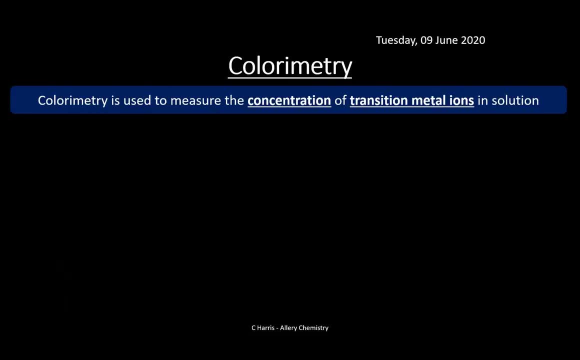 impact. the color that we see now in terms of colorimetry is a spectral technique, so this, this, obviously this set up here- is a way in which we can identify certain transition metals. okay, so colorimetry is used to measure the concentration of transition metal ions in solution. so it's got this set up here. 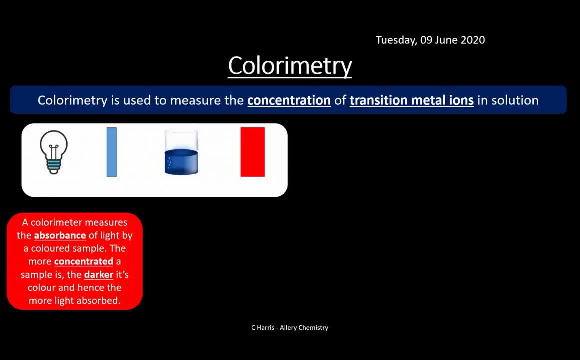 okay, so a colorimeter measures the absorbance of light by a colored sample, and the more concentrated a sample is, the darker its color and hence the more light is absorbed. so you can see, we've got this set up. we're going to use this diagram in a moment to show you what happens. so the first thing is the color. 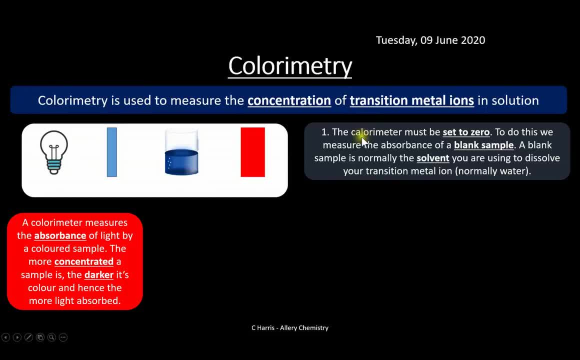 the colorimetry. that's not colorimetry, that should be colorimetry. okay, so the colorimetry must be set to zero, and to do this we measure the absorbance of a blank sample. okay, so the blank sample is normally the solvent we're using to dissolve your transition metal ion in, so that might be water for. 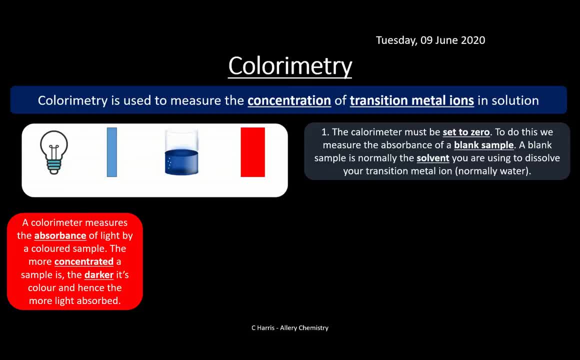 example. so we shine the light through and we take a zero. so we know that any absorbance has got to be because of the substance, the transition metal, rather than the solvent. okay, so that allows us to do that. so once we've got that, once we've got our benchmark, our zero, then white light is filtered into a narrow 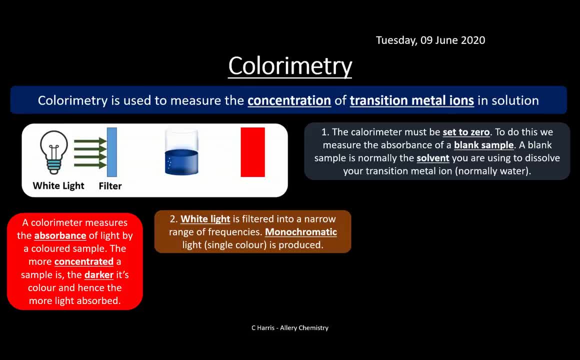 range of frequencies- so we call this monochromatic light, or it's a single color- is produced. so we've got white light there. it gets passed through a filter and we get one frequency of light that is produced. okay, now the choice of filter here is really. 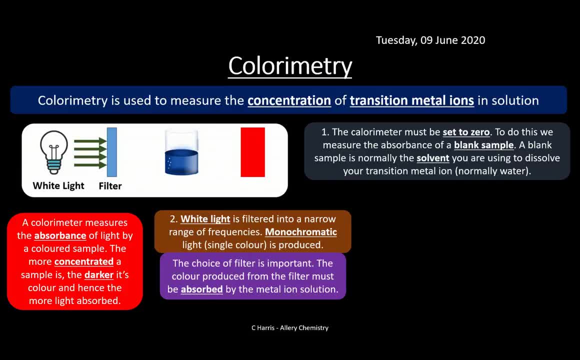 really important. so the color produced from the filter must be absorbed by the metal iron solution. okay, so depending on what filter we're using here, if we use the wrong filter, then it may not be absorbed at this end here. so we've got to make sure we're choosing the right filter here for the substance that we're. 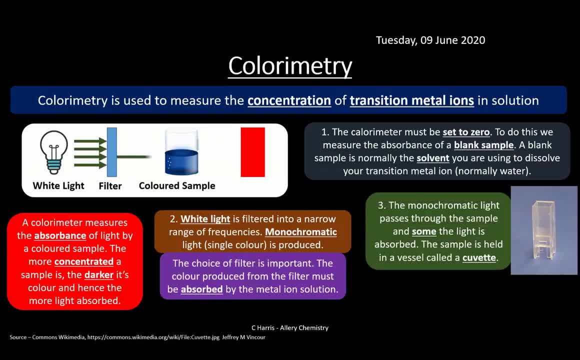 testing. so once it goes through the filter, we get this monochromatic light, as you can see here. now that's the colored sample there. in reality, it looks something like this: this is called a cuvette and you might have seen these- and they've got a frosted side at two sides and that's where you pick it. 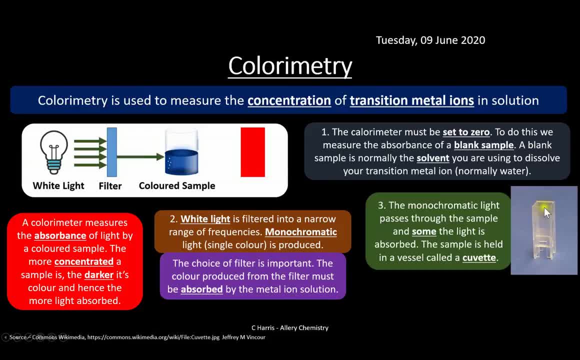 up and it's got a colorless side on the other side and that's where the light goes through that cuvette. so you put your sample in there and the light would then shoot through that cuvette and basically we're measuring the absorbance of that light. so some of that light here is going through will be absorbed by 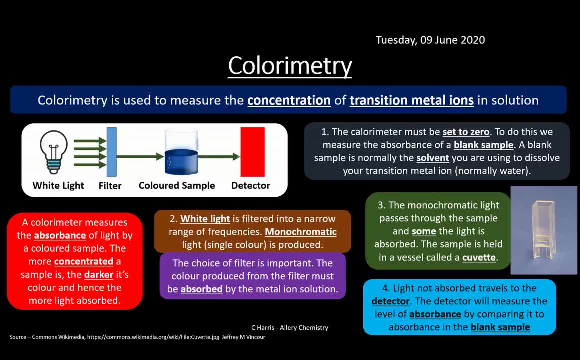 that colored sample and then at the other end, you can see that it's absorbed by the color sample, and then, at the other end, the light will go through the sample and it will hit the detector. now what the detector is doing is it's measuring the difference between the intensity of 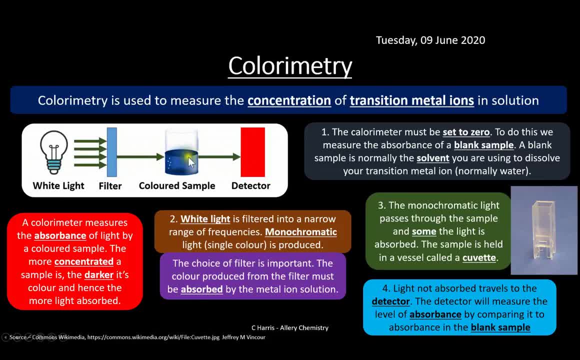 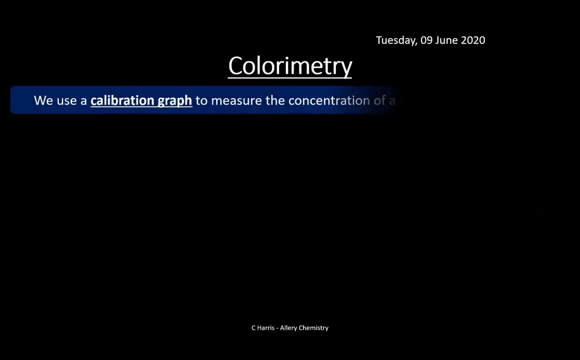 light here compared to the intensity of light here, and it's measuring the absorbance. how much light has been absorbed by this colored sample? okay, so that goes through to the detector and that's effect whether detector is measuring here. okay, so we use calibration graph to measure the 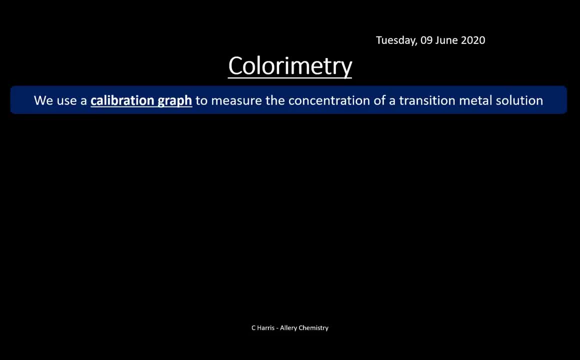 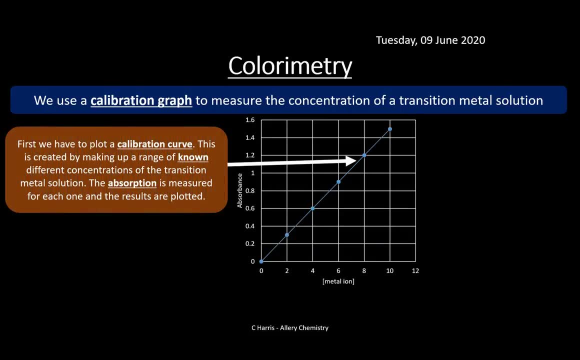 concentration of a transition metal solution. okay, so this is what we're going to be using to see how much of that transition metal we've got in our solution. so, first of all, what we have to do is we plot a calibration graph. so this is created by making up a range of known different concentrations of the 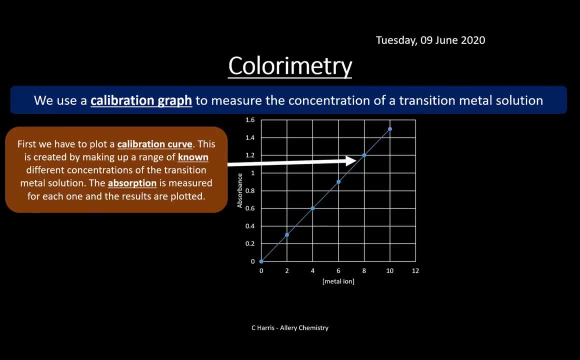 transition metal solution. okay so, and the absorption is measured for each one and the results are plotted. so we use that bit of equipment that we've just seen before. so we take, say, if it's copper sulfate solution, we make a known concentrations of copper sulfate solution, we measure the absorbance of. 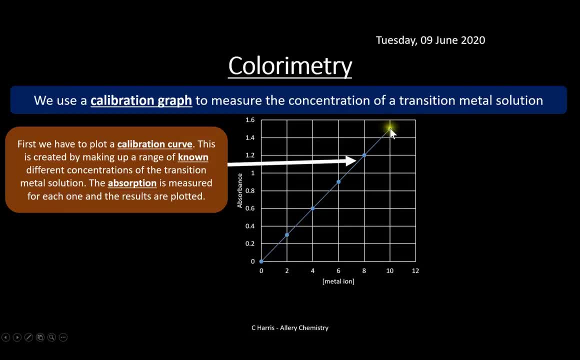 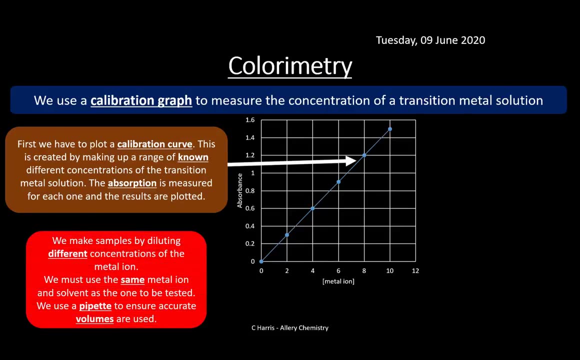 each of them concentrations, and we measure it on and we plot it on a graph like this. so this is a calibration curve. so we've got absorbance against the concentration of metal ion which we've, which we've made up, we've deliberately fixed the concentrations of these so we know what the absorbance is of each. now 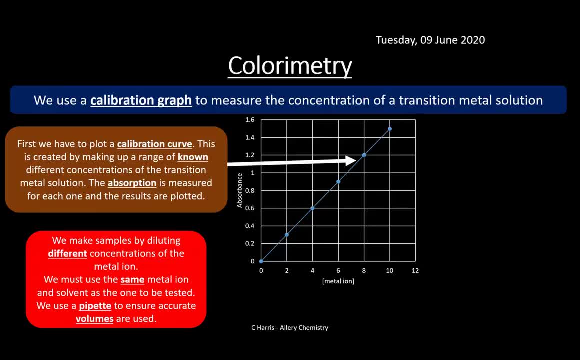 we do this? we make the samples by diluting different concentrations of the metal ion, like I say, and we must use the same metal ion and the solvent to the one that's going to be tested. so, in other words, if we're wanting to work out the concentration of a copper sulfate solution, for example, in other 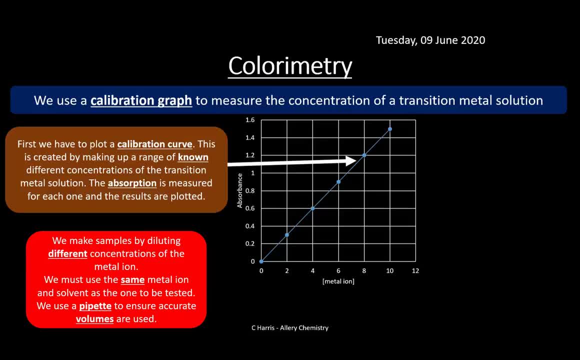 words, what's the concentration of copper ions in there? then we must make ready, or we must make known concentrations of the same metal ion using the same solvent. so for dissolving it in water we must use everything the same, okay, and we use pipettes to measure the, to measure the volumes of these, of these known samples. 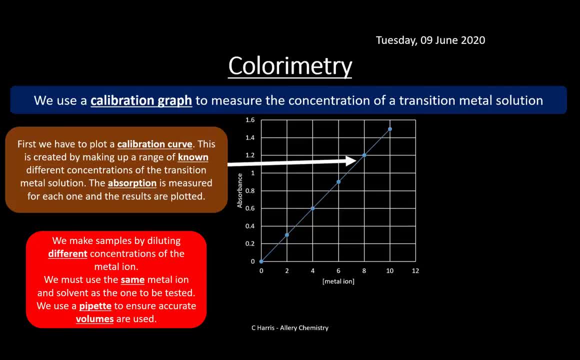 that we're going to be using, and we're going to be using them to measure the we're making up here. we use a pipette to do that, okay. so we then test the sample that we want to know. so we've got our known samples here, so we've made up a. 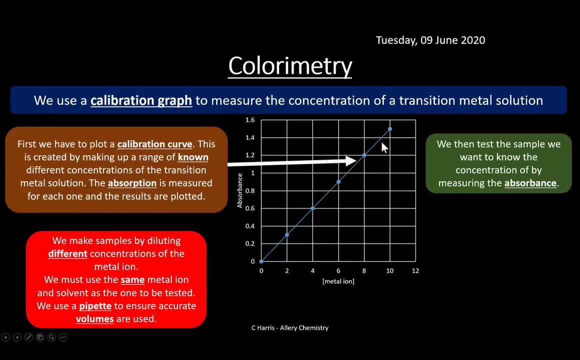 range of different concentrations, measure the absorbance and plot them on this graph. we then bring in our one that we want to test- okay, and we measure the absorbance of that, okay, so we put that into our colorimiters- colorimetry- colorimeter as it's shown before- and we measure the absorbance. and once we know, 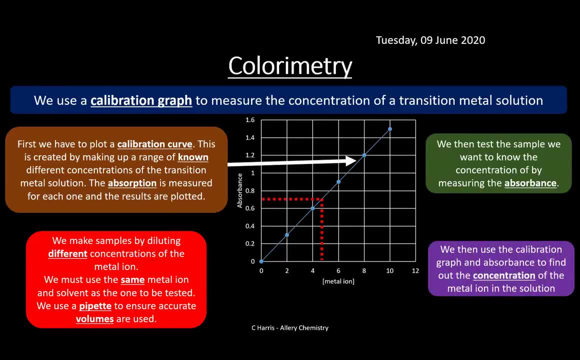 the absorbance of that. we then plot it on this graph, and then this graph allows us to work out the concentration of the metal ion from the absorbance of our unknown substance. okay, so we use that to work that out. so it's fairly straightforward, as you can see. 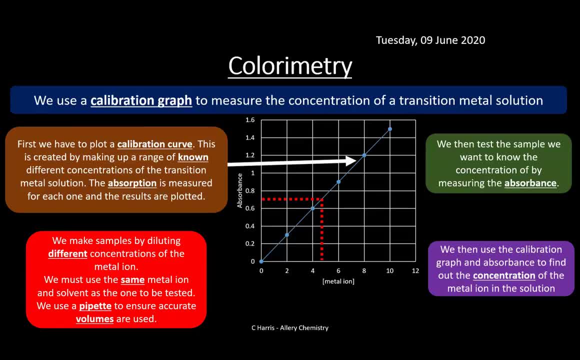 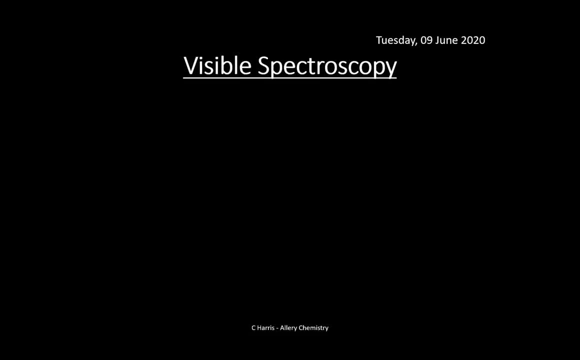 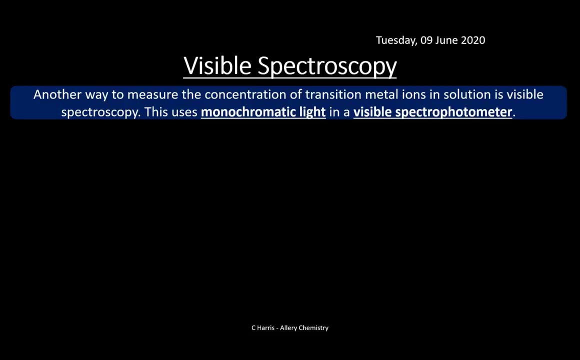 it's quite clever way of working out, you know, the, the, the other concentration of our, of our transition metal ion. now, finally, another way of using color. we can actually identify transition metals as well in our solution by using some called visible spectroscopy. so it's also another way of measuring the concentration of transition metal. 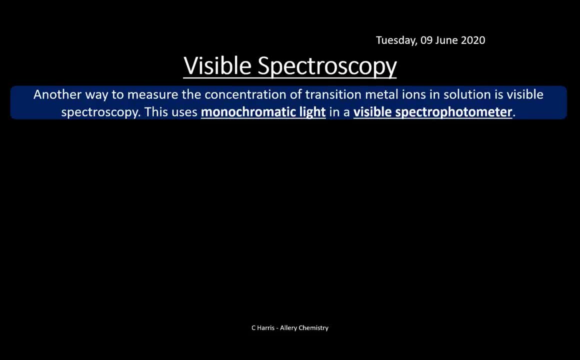 ions as well, and we can use. we use monochromatic light, as we've seen before in a book. this time, we're going to use a visible spectral photometer. okay, sounds complicated, isn't it? so we're going to use one of them instead. so white light. 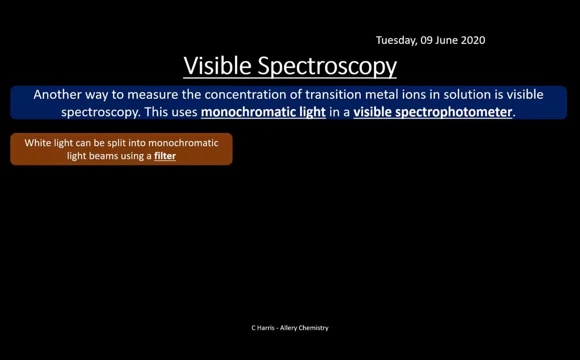 can be split into monochromatic light beams using a filter. so remember we'd seen that before in the previous bit of equipment, so there's no change there. okay, that monochromatic light beams then pass through your sample and the intensity is measured before it goes. 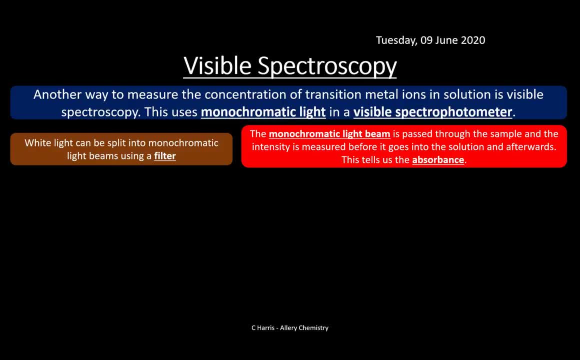 into the solution and afterwards, and this tells us the absorbance. again, there's no difference. what we've just seen before, it's exactly the same method. so far, okay. so we then use the calibration curve and the absorbance of the calibration graph and the absorbance to find out the concentration of the 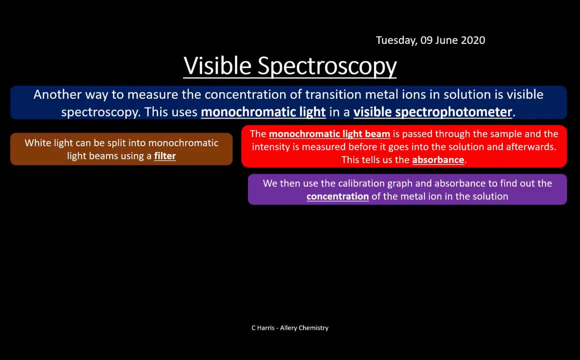 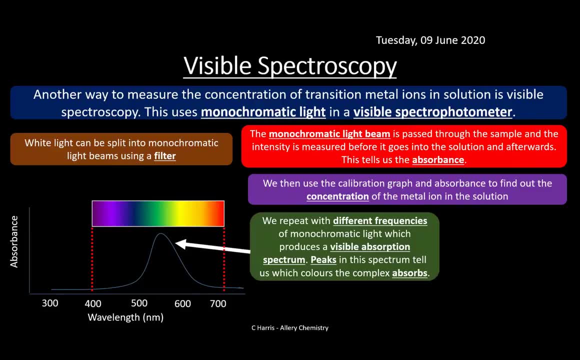 metal ion in the solution. okay, so that's what you're seeing in the previous slide there. now, with this one, what we can do is we can repeat that with different frequencies of monochromatic light. so we just keep repeating that and that same experiment, but we change the frequency of that and this produces what we call a visible absorption spectrum. so we 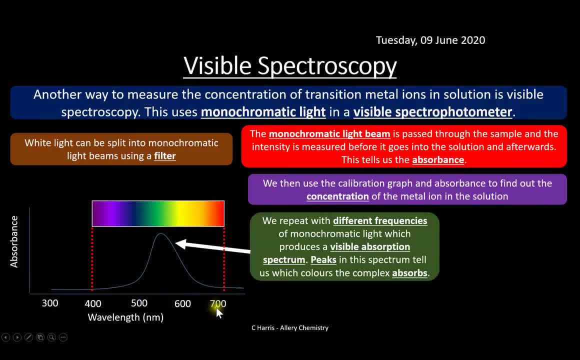 form something like this: you can see, there's our different wavelengths of visible light that we're putting in. this is the visible region as you can see there. so that's the colored light there, okay, and any peaks that we see in here, as you can see there. this will tell us which colors the complex.